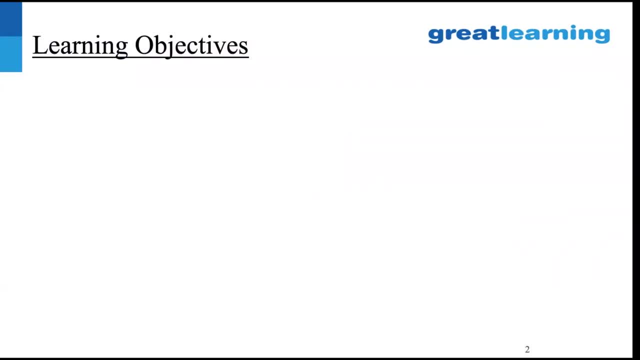 touched upon what is the purpose of visualization last time. Can someone quickly touch upon the scope of visualization, where we are, why we need visualization? Easy representation, Yes, easy representation of the data that is out there To make sense of the data. 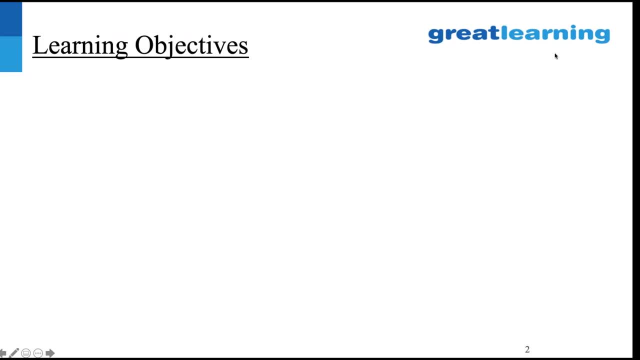 and to look at the patterns which you know, which right right See. basically two main points. I think both of you covered on the things Quickly. one is when you have a huge amount of data, it's not possible for you to go through each record that is out there and understand what the 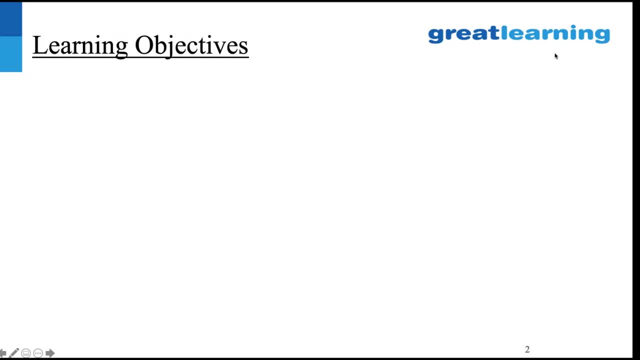 data is telling for you And also you want to do an analysis. you won't have the overall behavior of the data. So when you visually observe some data, it makes a lot more sense. you will try and observe patterns in the data. you try and observe anomalies. you try and observe. 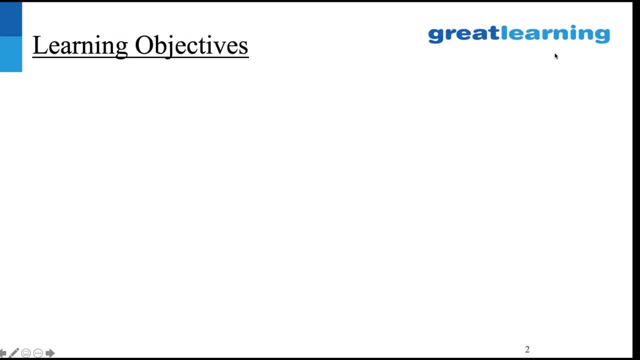 layers that are there in the data And you see what is the basic distribution of data that is out there. That's the primary focus of visualization from an analytics standpoint. then there is other purpose of visualization, which you presented data to business users so that they can understand. 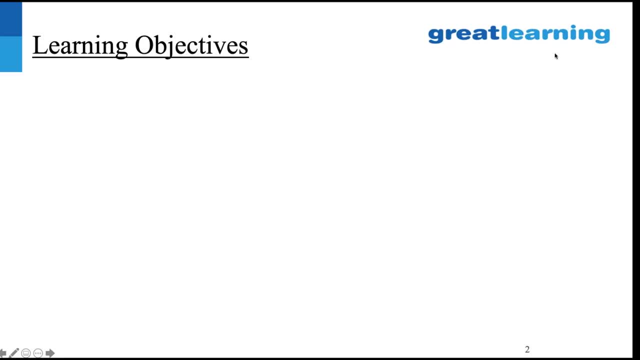 and interpret easily than going to the complex analytics of the things. So the two objectives of visualization. So now, where does this visualization come into play in the whole scheme of analysis? So let's quickly, we touched upon these things. let me go on to the next slide. 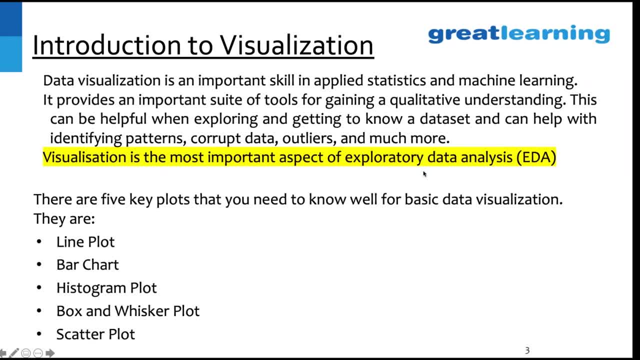 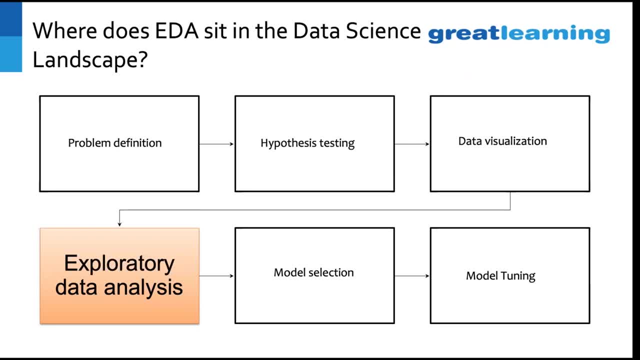 We touched upon these things, but we'll go in detail about this. Yeah right, So this is this whole scope of analysis. what happens right from you get a problem from your business to solve, to when you come up with the final model. So in the process, if you look at you have a problem that is given to you, you start. 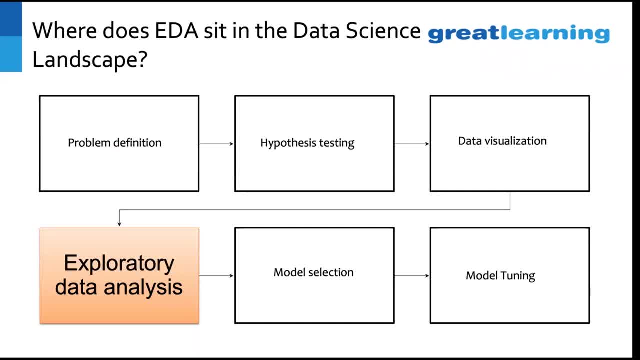 looking at the problem and you define what exactly are you going to solve. it is sometimes imperative that the problem that is stated by the business is not exactly the problem that needs to be solved, Because more often than not, the business talks about symptoms and not the problem. So it is your. 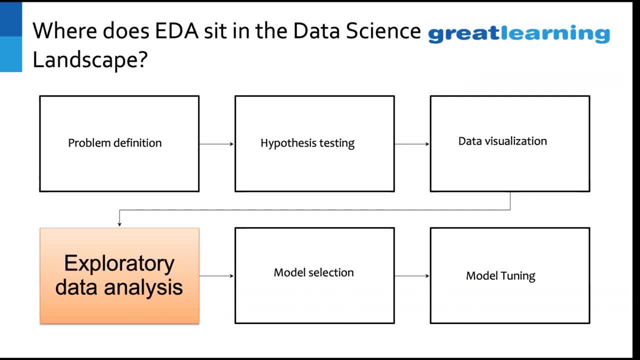 responsibility to translate that business problem into an analytical problem. There is temperature. you go to the doctor. the doctor does not treat for temperature symptoms. yes, he gives you paracetamol, But what is the underlying infection that is out there, How it is caused And what is? 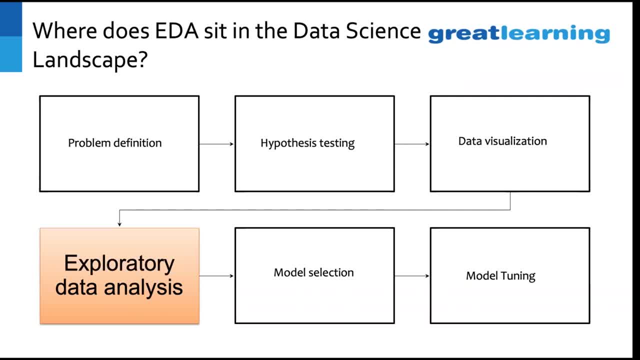 the antibiotic to be used is the doctor's responsibility. That's exactly the role of an analyst. you understand the problem, you convert that business problem into analytical problem And based on that you can solve the problem. So you can solve the problem. you can solve the problem. 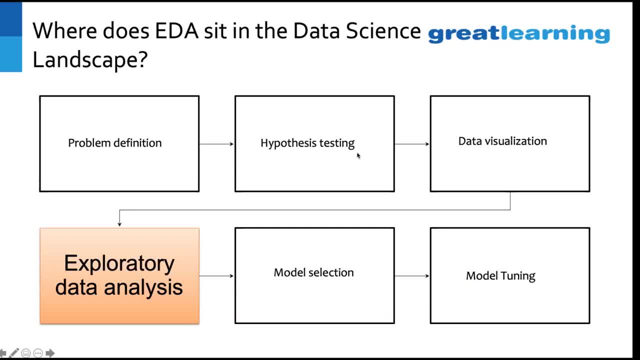 that you start creating your hypothesis. Once you create your hypothesis, then you start looking at your data, what my data is telling to solve my hypothesis, And then you come up with visualization here, essentially to see what my data is distribution, how it is looking like, what I can do. 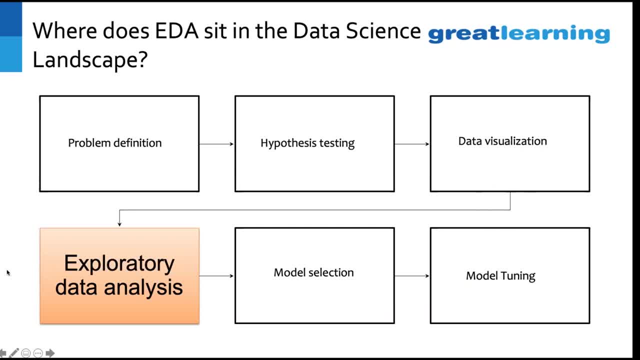 on it. then, once you understand your data visually, then you get into exploratory data analysis. So exploratory data analysis and this visualization go hand in hand. Once you analyze all your data, you get your initial results and everything. Then you get into creating a model And once the model is done, you test your model. you feel that. 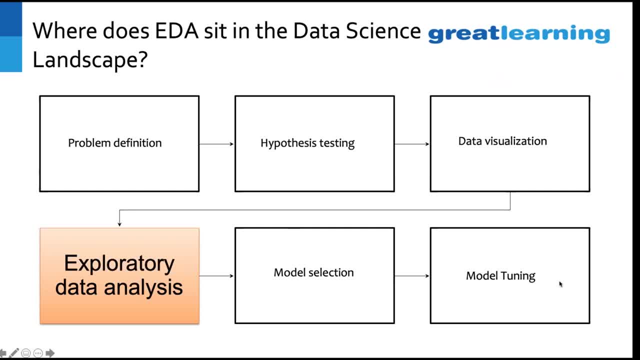 the model is working And then you start applying it And as the data comes in, you start tuning your model so that you get better results and optimize results. That's the flow of the exploratory data. analysis comes into play From that lens. there are four different terms that are used in the 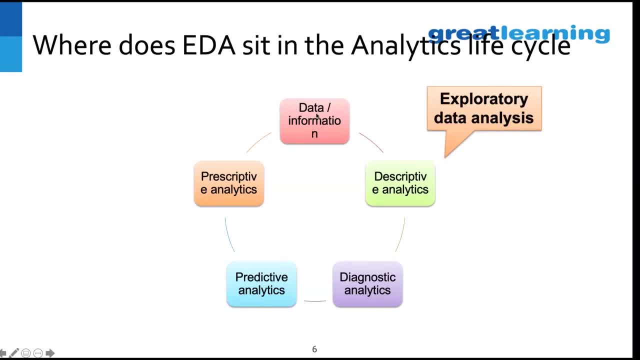 videos. if you have seen what are those four areas, you have your data or information. whichever way you call it, we look at what data was this information? Have you heard of these terms in the videos? descriptive analytics, diagnostic analytics. 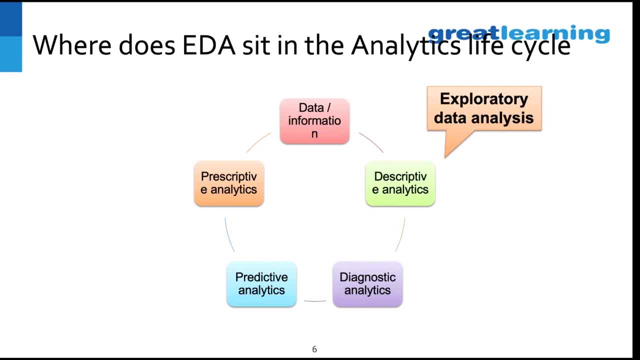 predictive and prescriptive. Yeah, What are these things, These terms? descriptive. What does that mean? It's describing what the data tells you. Yes, it's exactly what is happening with the data. So what we see, getting a basic sense of the data. what is it telling you? That's all descriptive. 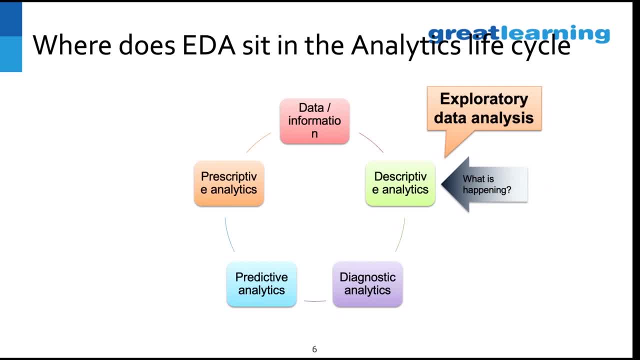 analytics does. So if you take an example, I go to the temperature example that I gave earlier. So if I go to the doctor, doctor sees it. okay, you're having temperature. for how long? you have it? for last three days, Are you? 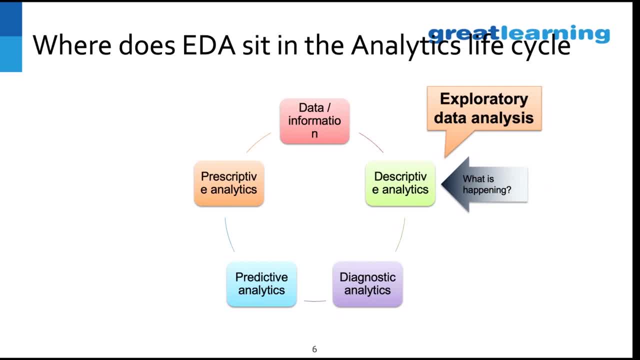 feeling hungry? Is the temperature continuously there versus it is coming off and on kind of a thing: Are you feeling sick? Do you have warm things? Do you have motions? he will check different parameters. it's data gathering and he's analyzing data and collating it to come up with an aggregated information, to come up with some. 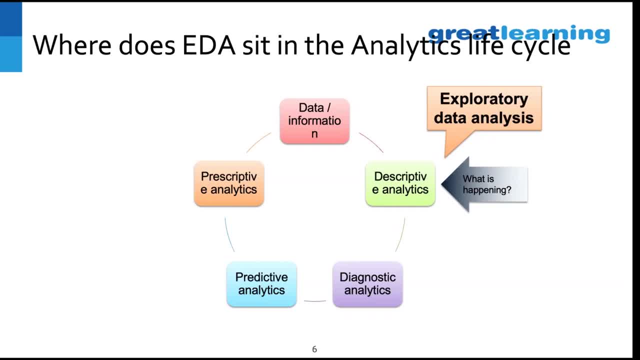 kind of a hypothesis to be formed. That's what descriptive analysis does. So we'll spend good amount of time on descriptive analytics today. But if we get deep into the diagnostics, why did Terence talk about what was happening before his jump? well, 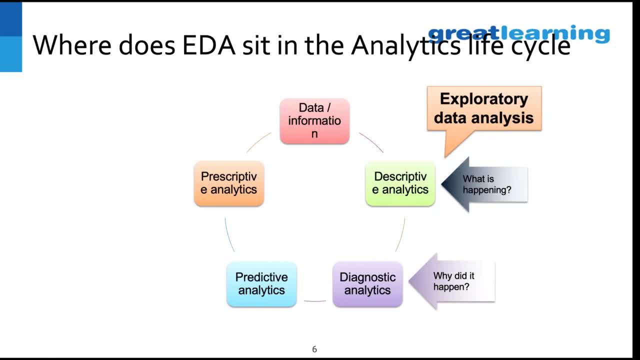 dead Or why did it happen? if you feel that you were vomiting your motions or something, then he gets into underlying causes. Why have you eaten food outside? Have you drink water from public tap? or submit Amirツ falak, have something. 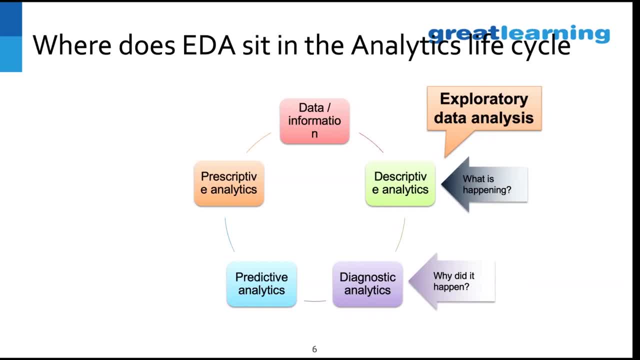 Moran oksana, that you ate food that is normally doesn't suit your body, Constitution something diagnostics would be done. Then you start predicting in what scenarios This is likely to happen. So in future, what you should avoid. doctor gives you kind of a prescriptive prediction and making why. 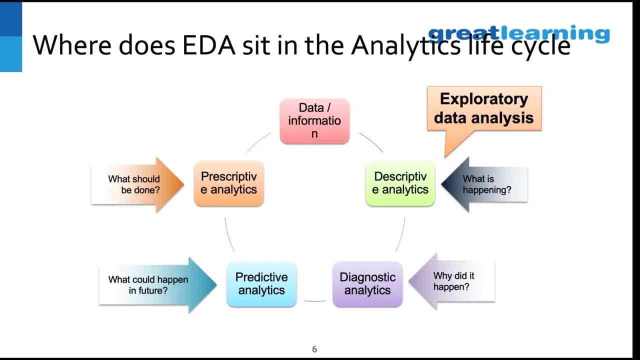 it will happen. Emed Raisin And he prescribes Moran oksana the medicines and the care that you need to take for yourself. same goes for an analogy example in analytics, business problems and anything. is the point clear? i i try to explain that through a very simple. 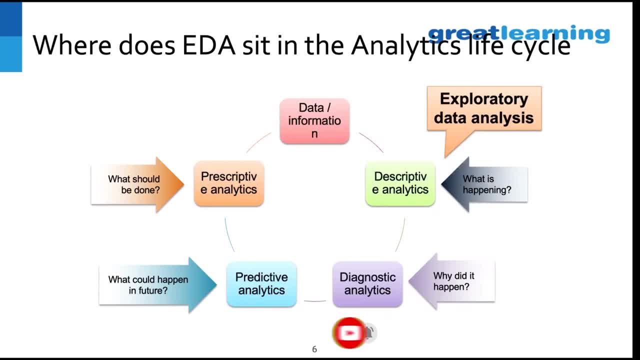 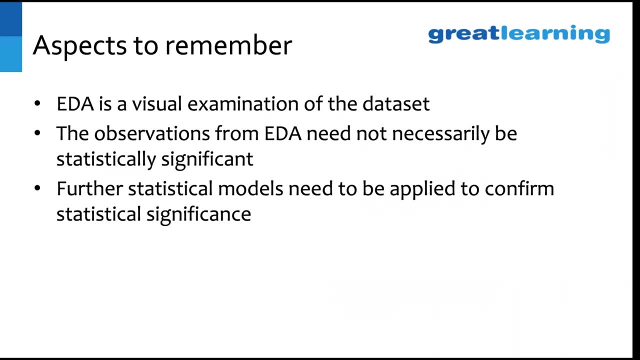 example, but the approach, the methodology that we take for applying for a business problem exactly lies into the same, so that we can connect with the terms. does that sound? does it resonate folks makes sense, yeah, great. so, yes, how many hypotheses do we actually create, or rather, do we have multiple hypotheses for the same data set? brilliant question, brilliant question. so yes, 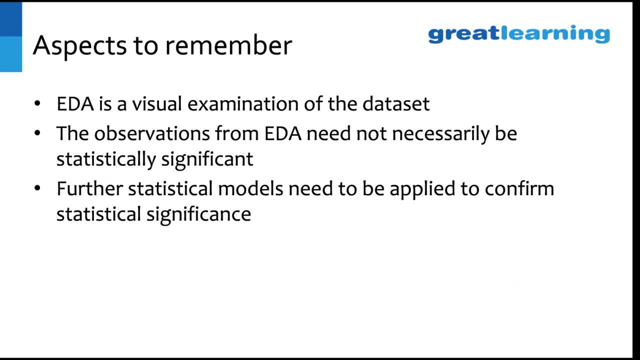 you can have n number of hypotheses that you can form based on your data. hypothesis is nothing but an articulation of business problem into an analytics problem. you are trying to solve a bigger problem. let's say tomorrow, your client- hypothetically i'm calling a retail firm- 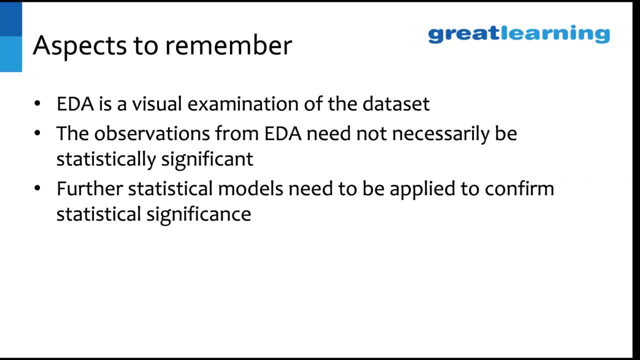 or one specific apparel firm like vimal or aravin mill. something comes to you that my sales are going down. what should i do? i'm seeing for the last four quarters my sales are continuously dropping down. i need to understand the problem. that's the problem that is given to you now. you 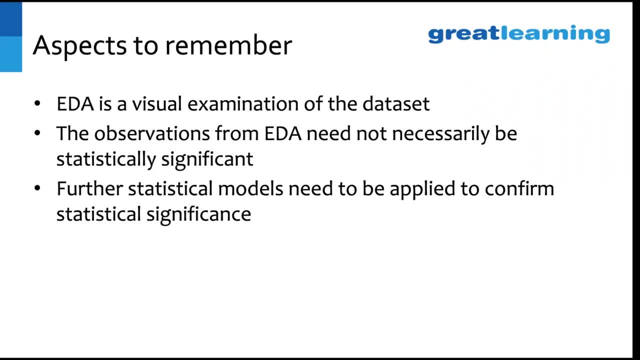 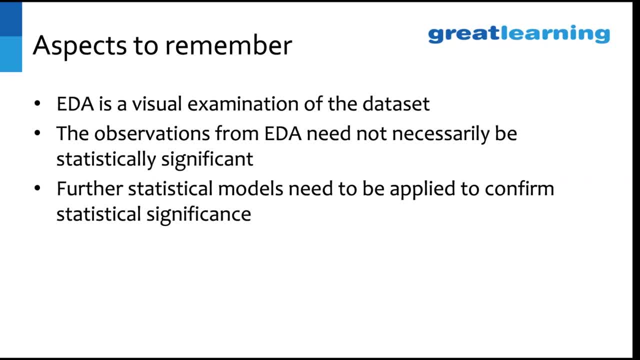 is it like men's section, women's section or kids section, or where are the sales dropping? then you know that. okay, across the sections you are seeing drop. okay, then the problem is not about the classification of the business unit. there could be something else. is it by geography particular? 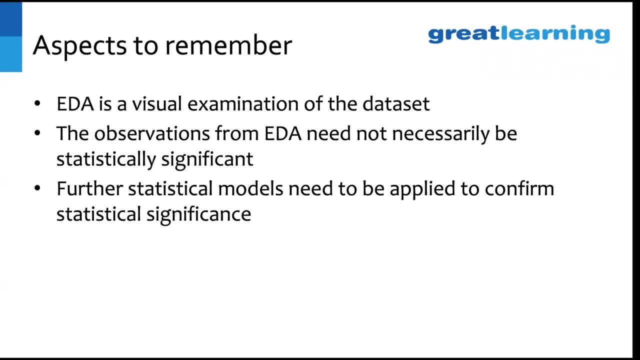 geography causing it, or particular season causing it, what is causing exactly where it is going. then you start digging deeper and understanding so you'll form- sometimes based on your intuitive hypothesis. can be formed on two things: one, once you do your exploratory data analysis, initial data patterns that are coming up, based on that you form a hypothesis. or, as a business intuition, your 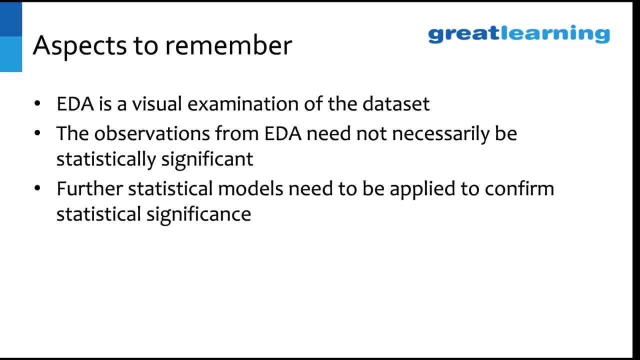 business knows a new competitor emerged, so you know a competitor is playing a role. then your hypothesis could be different or in some cases, both could be a reason. you have a production related issues, you have a competitor coming into play, you have a market changes that are happening, and then you start digging deeper and understanding. so you'll form, sometimes based on 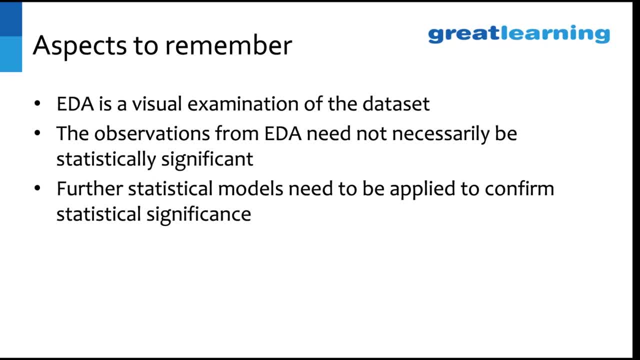 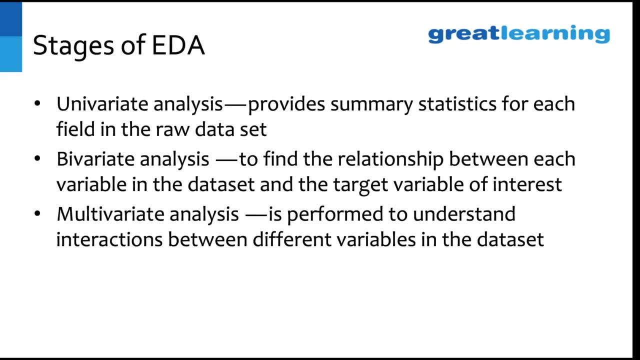 then you form three different hypotheses of the same data and you solve three things in three different ways, so you can form a number of hypotheses on your data. all right, so let's move on. so this is where the data comes in and the next step as we are talking about here. 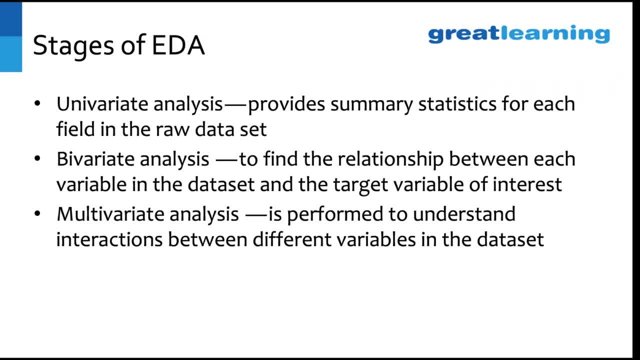 there are three stages of exploratory data analysis. one is univariate analysis. two is bivariate analysis. three is multivariate analysis. i'm assuming through the videos you would have gone through, i'm just skimming through and giving you clarity on the things. univariate analysis: 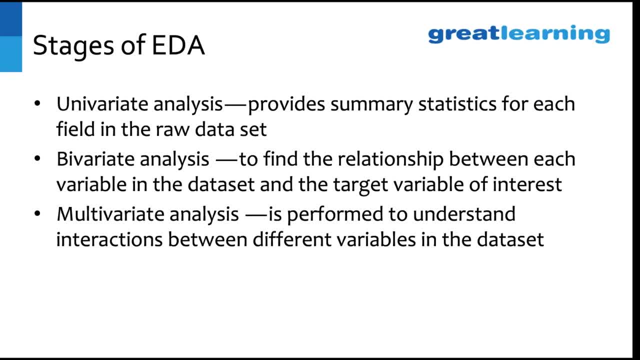 is all about. you take one variable, like you take temperature, and anything you do is just about temperature. you do analysis of the data- temperature collected over a period of time- and you do certain analysis on that one. it can be mean, it can be median, it can be trending patterns, ups downs. 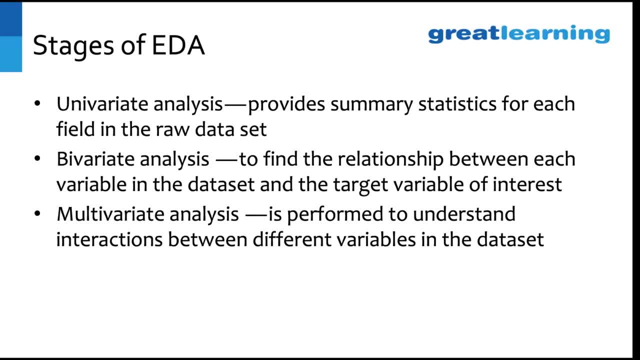 whatever it is going, you do only one variable level analysis, then two variables, when two variables have a interplay between them. so, for example, when temperature is coming into play and water scarcity in a city, you, the temperature goes up, water scarcity goes up. as the temperature goes down, water scarcity goes down. 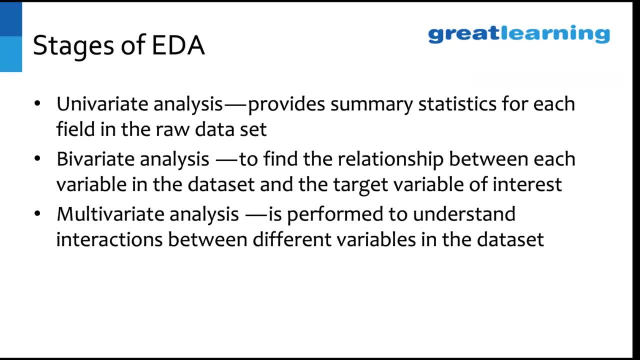 is it just these two variables? how much they are connected with each other? how is one related to the other? one is a bivariate analysis. when i say multivariate, it's not about temperature and water availability in the city. there is a third dimension that is out there, which is: can someone think about? 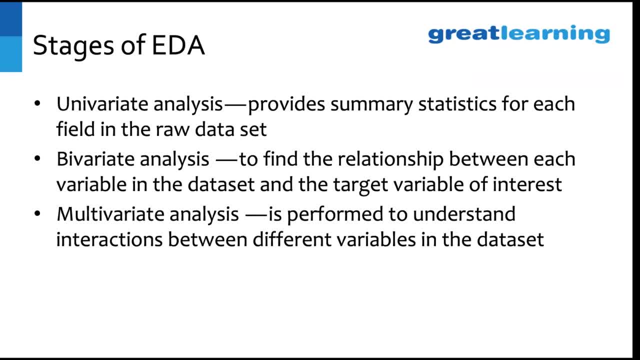 what is the third dimension that can come into play? rainfall. so rainfall is the other one. so, despite having high temperatures, that area is known to get a lot of rain. so as the rain has gone down, so now you can see that the area is known to get a lot of rain, so as the rain has gone down, so now. 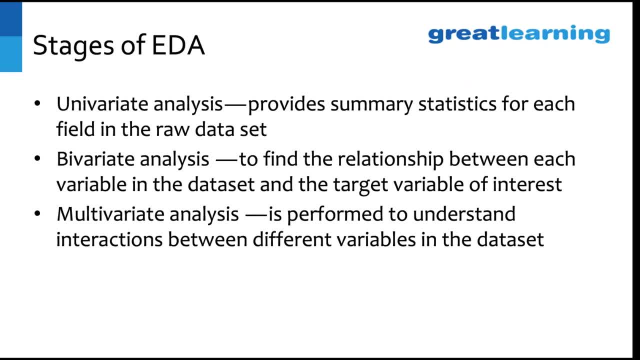 how is the interplay between your temperature, rains and waterfall? uh, are the rainfall coming in? so those three variables. we will play a multivariate analysis. you understand different dimensions. so this is the simplest of the examples. once you get into your business problems, you'll start dealing with thousand variables, two thousand variables, 3000 variables, then the interplay. 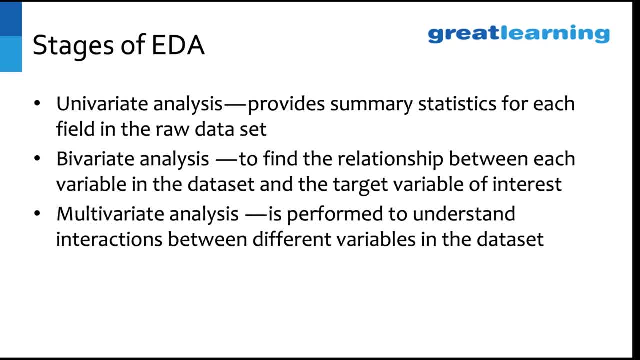 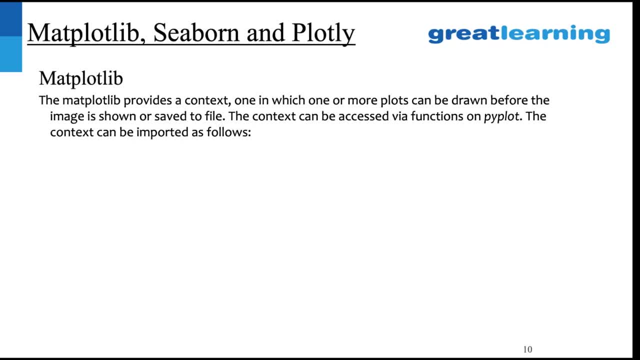 between all these variables really, really becomes complex. so this is all what we'll try and analyze in the process, right? so just moving on. so there are three different libraries. we have seen matplotlib, seaborn and plotly that we touched upon last time. i will go through a case study now, uh, to see each of these things plotly. we won't touch because it's. 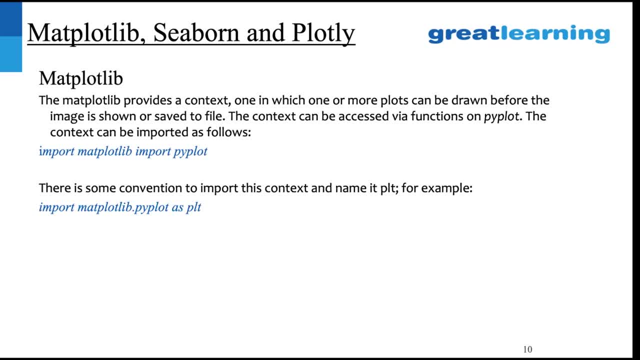 primarily a web related stuff, more about dynamic visualizations and everything slightly away. if you are interested, you can definitely touch upon. there's a complete library available for the purpose of this session and these classes. we predominantly rely on matplotlib and seaborn, which should be pretty good enough for us. okay, so the syntax will get into the case study and 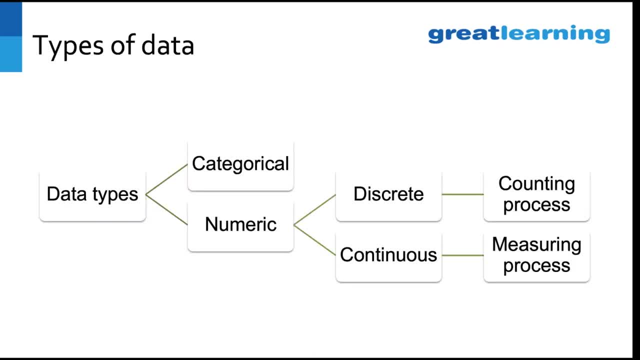 we'll solve that now. the data you you have heard of these terms in the last week's videos, as well as uh statistics videos. you would have seen these classifications, two different types of data, sorry. yes, so there are two different types of data that we primarily look at. one is quantitative. 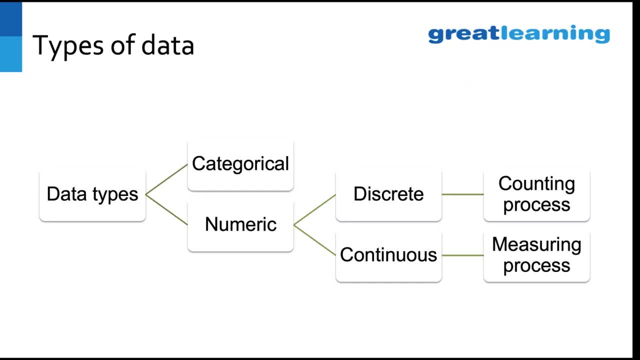 data. the other one is qualitative data. your qualitative data is nothing, but your categorical quantitative data is all about numeric and again, each of these things will get divided into two types. your categorical data can be two types: ordinal scale, all these things. so what is nominal? let's take small example of quickly what is nominal data looks like. any example for nominal data name: 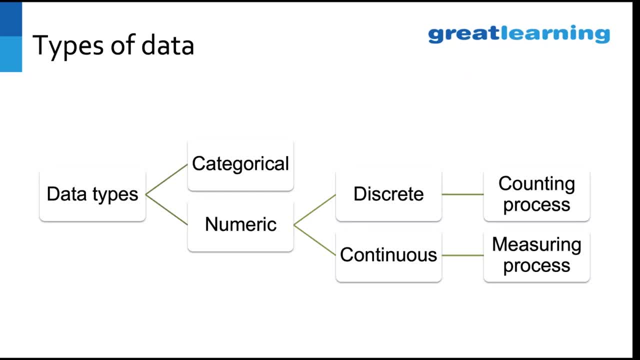 name, yes, but just name alone, or anything else? car color, wherein you have a finite set of variables or attributes. so what is the purpose of a nominal variable? why a nominal variable is used? it's purely for the purpose of identification, nothing else. so it's like an identification id that you use in a data set. you use a country name. it's for identification. 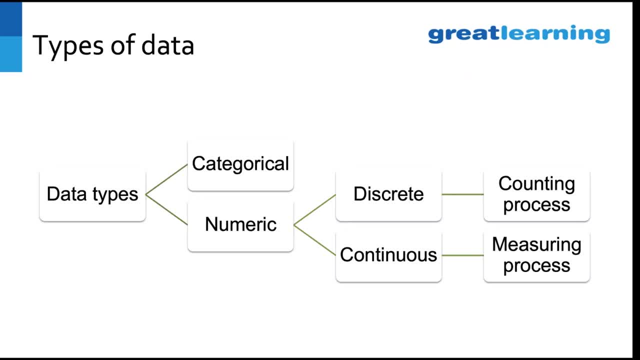 purpose. in a classroom you use a person's name. it is for identifying that person, tracking his record, what he is doing. in a gdp you perform how countries gdp is growing. what is the inflation? what is the wpi- whole price index, consumer price index- everything you are capturing against every. 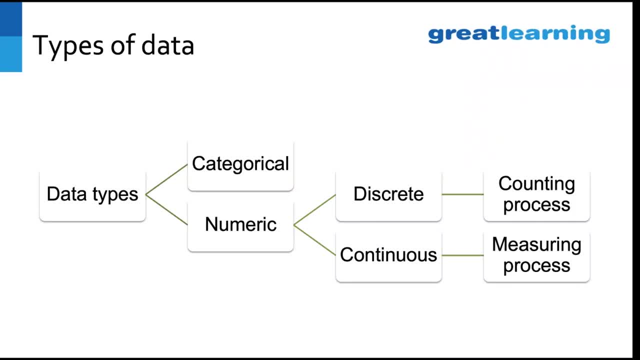 country that is out there country becomes a nominal variable. all you have to do is to use a reference rest of the data with that particular variable. it's that connection that is out there. that is the purpose of nominal variable. so, yes, sorry, this can be used as an address, if any, yeah. 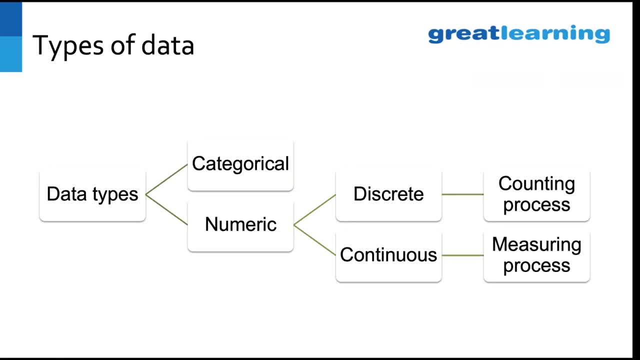 anything. it is one single value- is just for the purpose of identification. for example, if you talk about address address- sorry, i missed the point. can you come again? is this can we use as a address for that data stream? yes, yes, yeah, exactly, exactly, and now i get it. it is like an address for that particular thing. 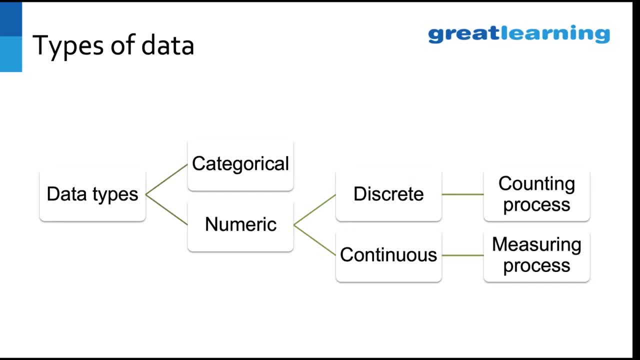 so rest of all the data is referred by that variable. that is out there. that's what i. when you mentioned address, i literally took the regular postal address that you are talking about. no, it's the address of the data. that's how it is. it can be considered. absolutely, absolutely makes sense. 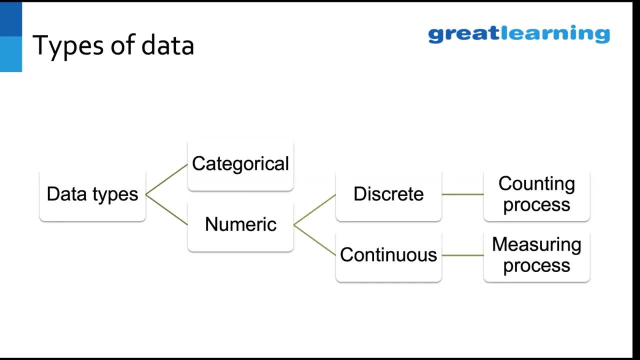 right. so the second type of the data is or ordinal data. boolean is one type, we'll come to that. but what is ordinal data? what does ordinal mean? there is an order in place. let's say, for example, a telephone directory. names are arranged in alphabetical order, but beyond alphabetical 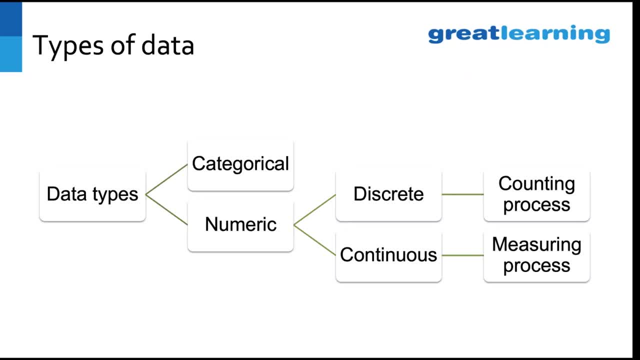 order. for easier reference. does the order make any difference there? a phone number associated with the name is just a nominal data, but you just put it in an alphabetical order. it helps you in getting some sense. you arrange the data in alphabetical order, that's all. there's no, no other things that you can do on a nominal data except for identification. 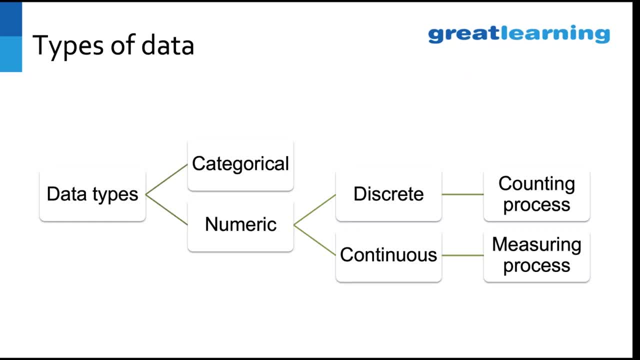 you cannot do any other operation on that data. for ordinal data, you can arrange them in a order. it is like low, medium, high, it is like good, bad ugly. you, you know the difference between the things, but you cannot do anything other than ordering them in a place. so if i know something, 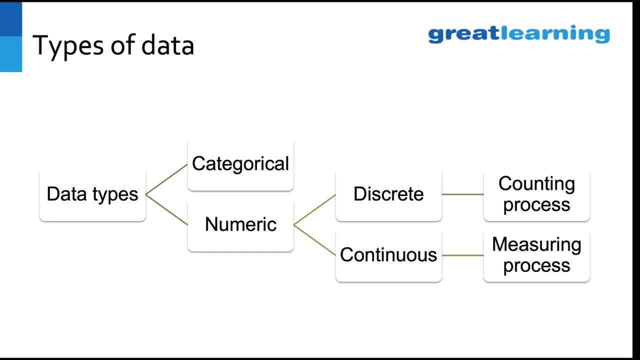 is good or bad. i can just put it in an alphabetical order. i can just put it in an alphabetical order. then something, some other thing. can i know how much good it is unless you have a measure, unless you have a metric to calculate? what is the quantifiable value of those good and bad there? 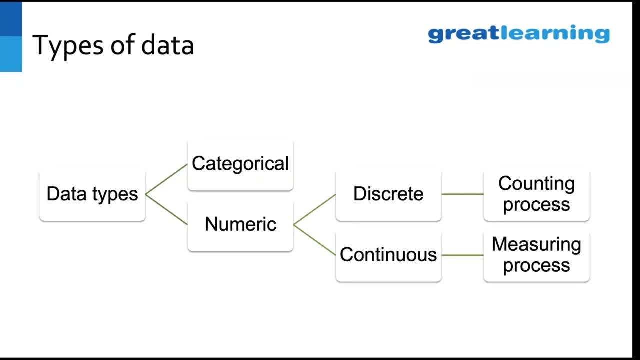 is no way you can differentiate them. so that's what the ordinal data does. it just orders them in a particular way. but there is no way for you to distinguish how good it is or how bad it is or how ugly it is. that's what the ordinal data does, so your categorical data primarily handles those two. 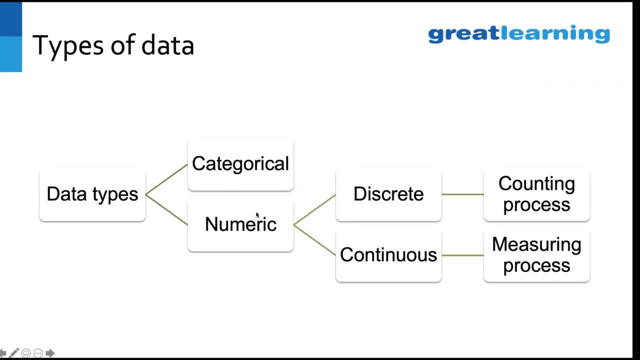 types, then your numerical data. we'll come back to that when we touch statistics again. we get those slides, we get this binary and symmetric binary, asymmetric binary. we'll touch on those things. this is primarily for the purpose of visualization. when you do visualization, there is a categorical data. 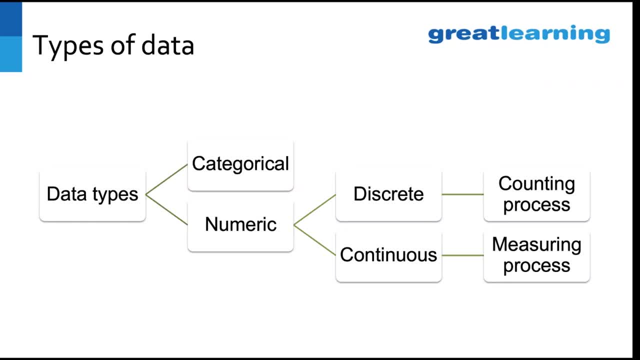 you can combine nominal and ordinal together as one unit and then you apply those labels for your numeric data. so now just we'll jump on to numeric data. what does numeric data tell us? what kind of data is there a numeric data? two types we are seeing here: discrete and continuous. what is the difference? 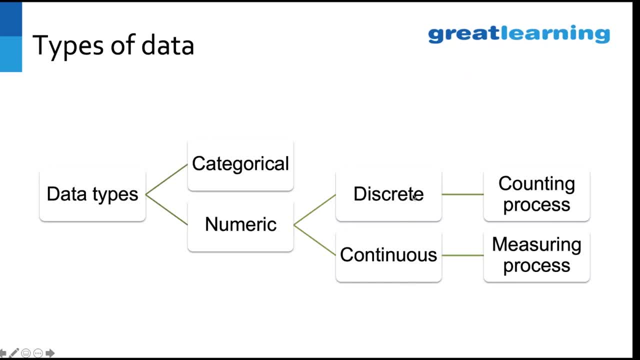 continuous changing with respect to time. discrete is a whole, whole value. there is no parts or something in that particular process. then in continuous the data is like at analog scale. you can think one as digital, one as analog kind of thing. this is very, very basic and name example. but one is digital. when is analog analog? 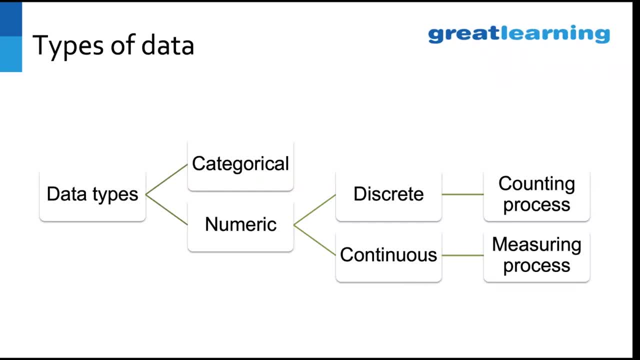 is like. it's a continuous value, continuous thing. it goes on to digital and analog. it's the same thing. if you look at the previous data, whenever you use it, you can look at the next, get to the next in the next. it goes on. discrete is very value in that particular, based on the. 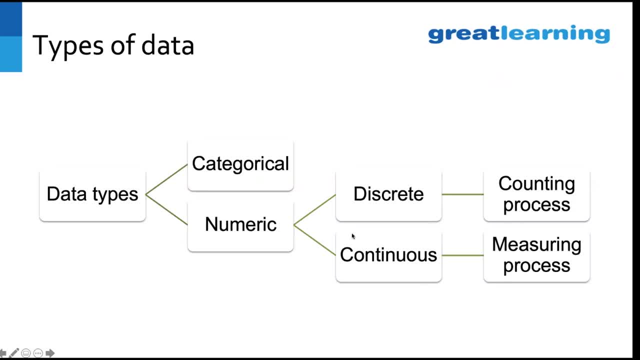 visualizations that you are trying to do. you can do two types of analysis. one is you can represent your data. you have numeric data you represented in some form. some charts are more convenient to represent. you have some categorical data. some charts are convenient and some charts cannot use categorical data at 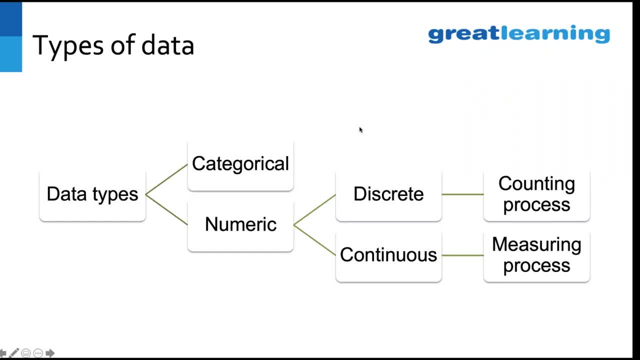 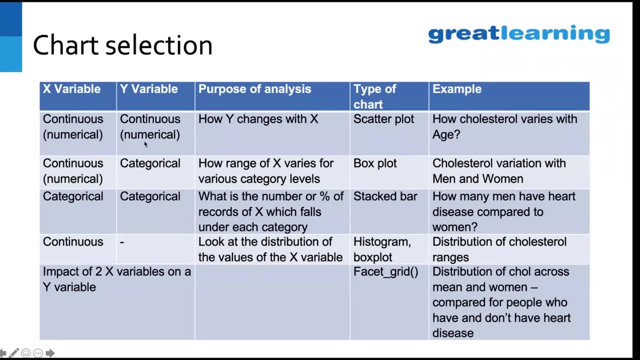 all. so we will see which charts are convenient to represent what. so let's see: for example, you have a continuous data. you are taking here two variables: X variable and Y variable. you are using that. so now you have to combine X and Y and see how the Y is changing with X. you come up with something called as a. 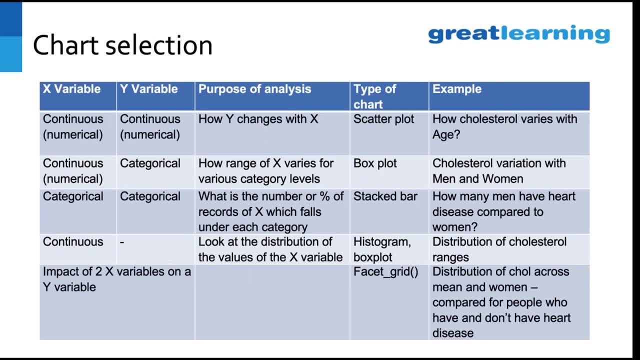 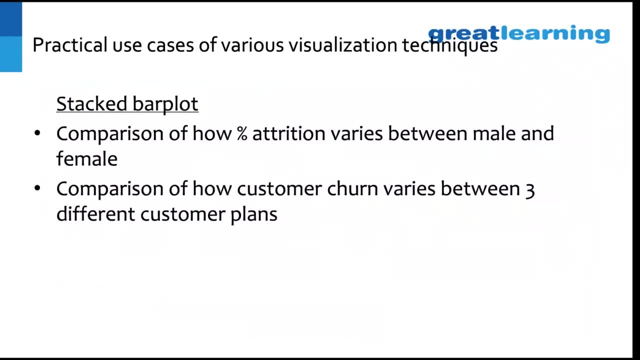 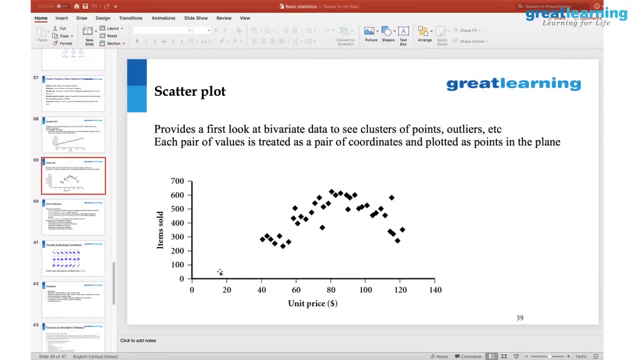 scatter plot. you have seen a scatter plot, rightly, in the videos you would have gone through. so what does the scatter plot do? I was just trying to look for an image of that scatter plot. a bunch of dots in next job, right. first fair point. let me jump onto the statistic because I am combining two. 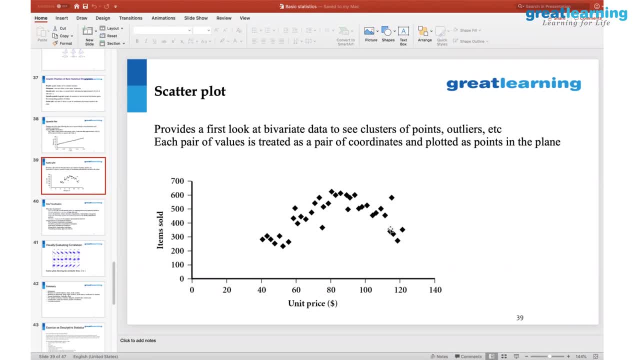 sessions here. this is, for example, is a scatter plot for you. so every point represents a value of X and a value of phi, but every individual, every record, for one record you have two values, X and Y, and that is pointed here. so if there are a number of observations, there are endpoints which are scattered across in. 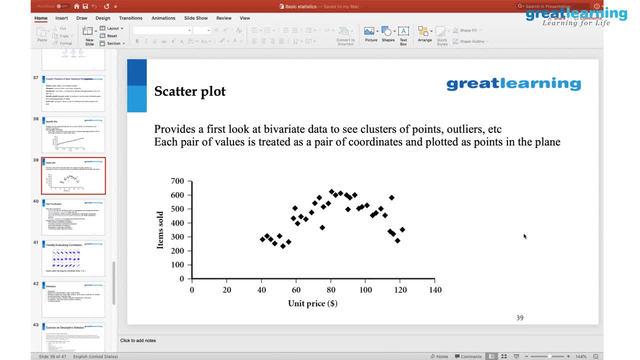 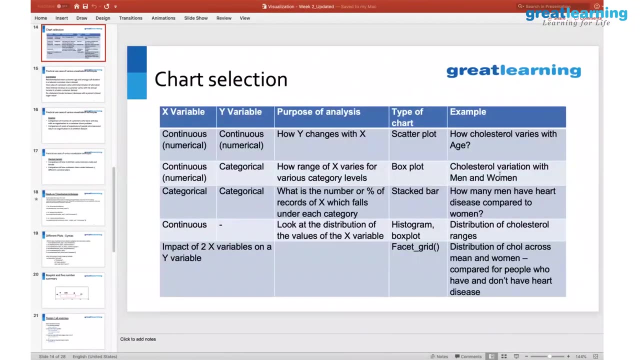 the plot of a linear. that's why it's called scatter plot. so the scatter plot primarily tells you distribution of data in the surface, how the data is being distributed, so you'll get a sense of what the pattern is, what is happening in that particular one. so that's scatter plot. so box plot: has anyone 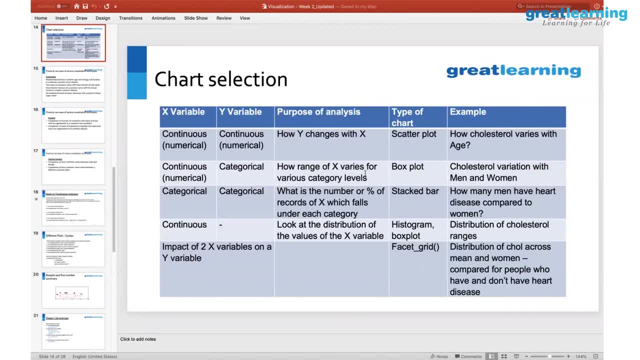 seen what a box plot is. yes, so what does the box plot represent? yeah, it's a five. it's a five point summary of your data. you, you have one variable, that variable you can have, and if it is a numeric variable, because it's a continuous variable, you can represent five different values. so what are? 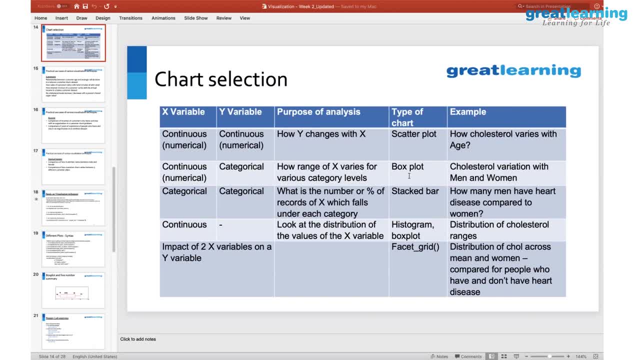 the five different values that a box plot can give you. what is the minimum value, what is the maximum value, what is the first quartile, what is the median, or also called as a second quartile, and what is the third quartile. so the order would be like minimum, first quartile, median or second. 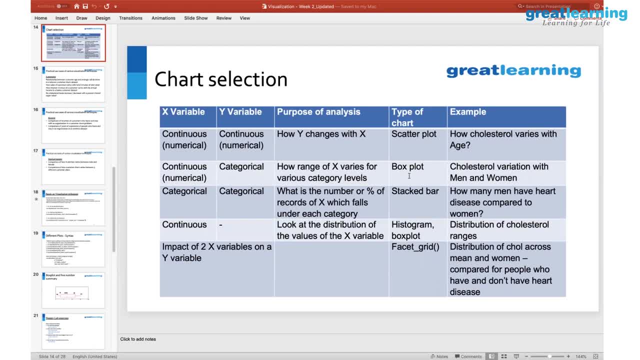 quartile, third quartile and maximum. these five values are represented by a box plot. we'll look into box plot how it looks like and the same. let's say, for example, your data temperature. as i said, you have temperature data continuously, which is a continuous variable. you can draw a box plot of it. but let's say i have 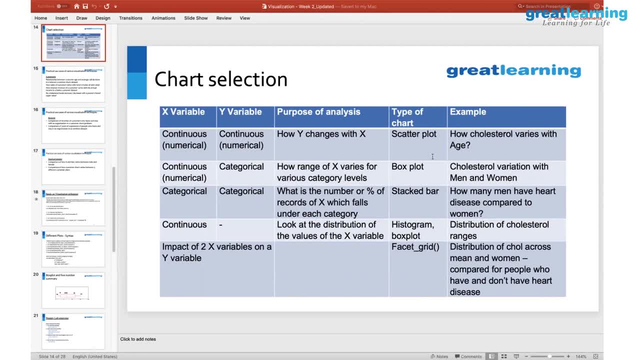 temperature captured for three different cities. so if i break that box plot by a categorical variable, i can get it for three different box plots, for three regions or three cities. that's why categorical variable comes into play. beyond that there is no application for categorical here. and when we say stack bar, stack bar is more like a. 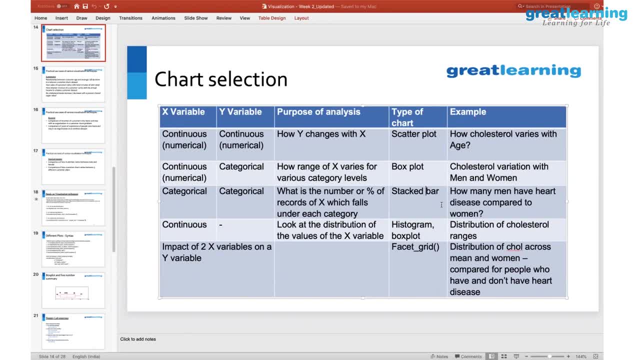 histogram kind of a thing, so it just represents one value and how much it is. that's all what stackbar can do. so, for example, you see how many men have heart disease compared to women. so you can have two bars, one for men, one for women. number of men having a heart disease, number of women. 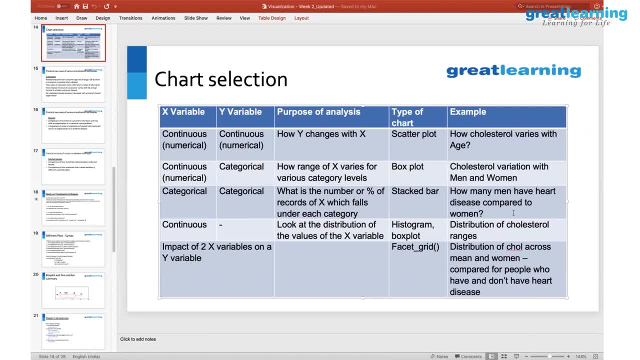 having a heart disease. that's all stackbar can do. and if we want to combine all human beings together one single bar, you can break that bar into two parts. half of it is represented by men and a different part of the other part of it is represented by females. so that's what is stacked. 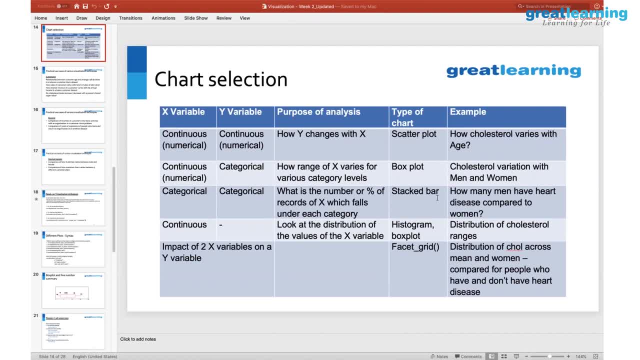 bar stack is one over the other. essentially, you can have two different bars versus in the same bar, you can have two parts histogram. and how does the histogram work? what does the histogram tell us? frequency, perfect. it basically talks about the distribution of data, and you divide your data. 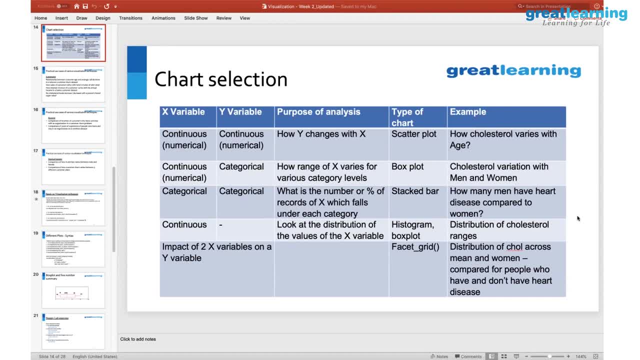 into different classes or you have certain categories in your data. each of the categories, what is the frequency? that's what a histogram plots. at the end of the day, facet grid- when we get into there we'll create. facet grid- is about creating some grid or an image where you can have different plots plotted. 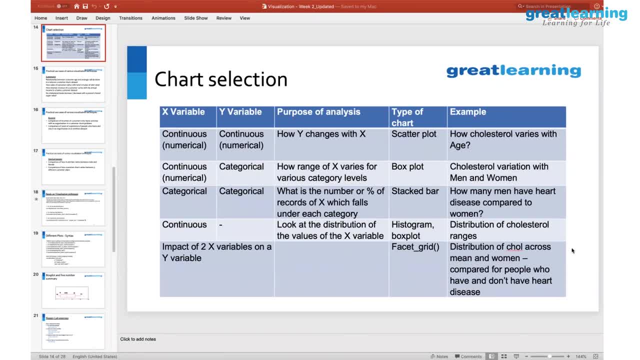 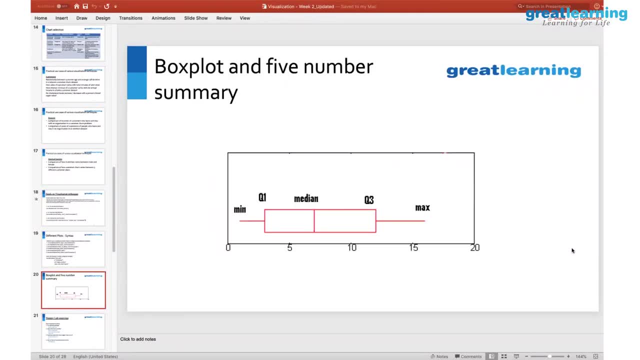 together and you can use it for representation purposes. we'll get into facet grid when we touch on example in seaborn. we'll do that right. so this is a box plot that we talked about: minimum, q1, median q3 and max. so here is the case study that we talked about we quickly touched upon last time. 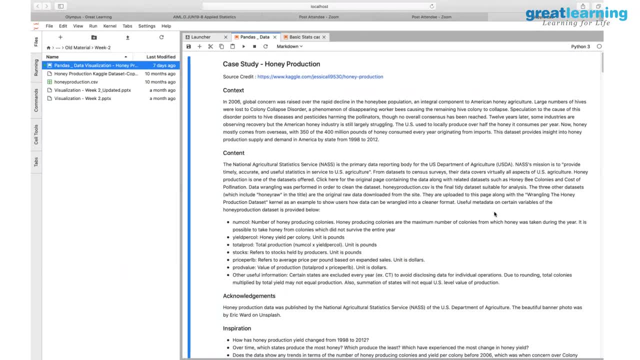 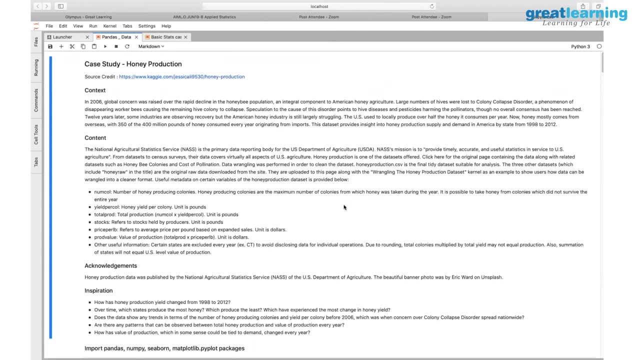 any questions anyone on the different types of charts. once we see examples of those things, we get more questions and we get more clarity on the things. but if you have any questions, please ask me. okay, this case study is all about honey production in united states at some point. so what they have realized is: historically, 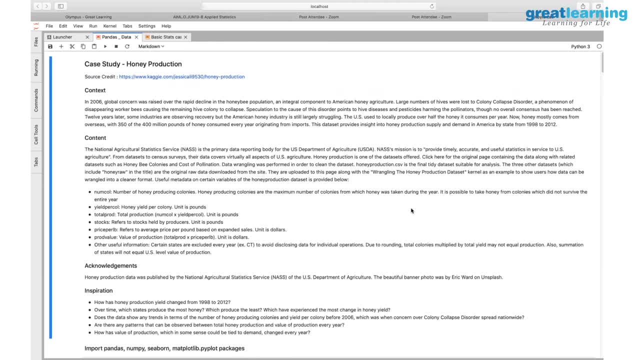 honey us, which has been very self-sufficient in honey production and consumption, they started relying on honey- importing honey from other countries, essentially so. then they start to gathering the data historically and they wanted to do an analysis of what is all causing that honey production, what are the reasons that are happening, what data we have and what are the. 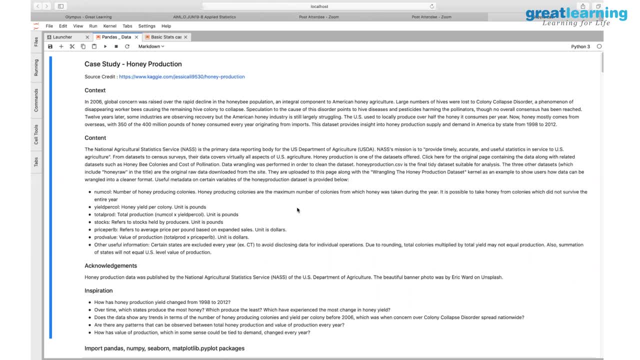 insights we can gather from that particular data. that's the exercise, essentially so, the us user to locally produce honey. or now, honey mostly comes from overseas, with 350 to 400 million pounds of honey consumed originating from imports. primarily so, that's the extent it has. so the data that we 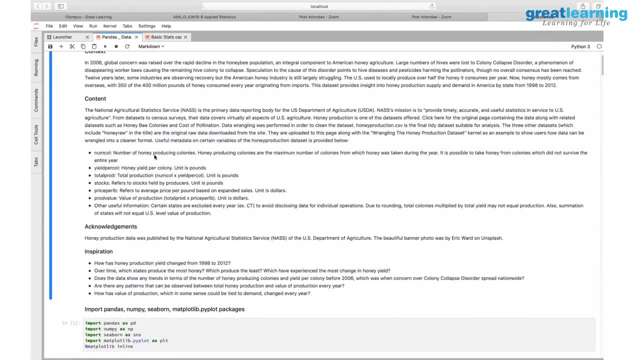 have at this point is there's one particular variable, which is number of honey producing colonies. if i have to just think about how honey is produced, honey is produced by honeybees which are in a hive, so so many honey is getting them produce the honey. those and those bees are called us working bees, so those are predominantly. 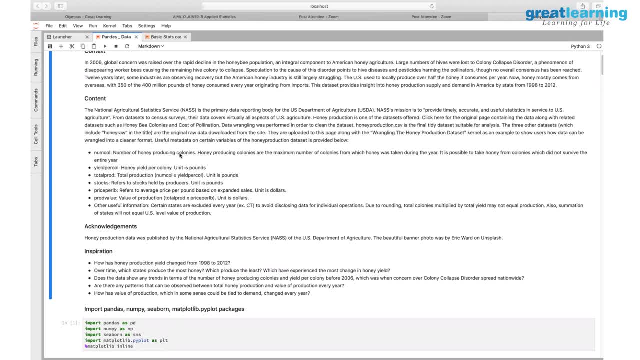 very important for producing honey. so this is number of honey producing colonies. how many colonies means it's a collection of uh beast is called as a colony, so how many honey producing colonies are there? What is the maximum number of colonies from which honey is taken during which year? 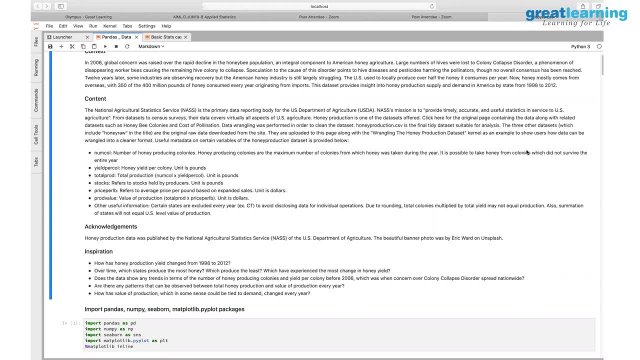 So that's the thing. So one colony how much honey it has produced during the year, that's the data is captured. What is the yield? Honey yield per colony in pounds, Then total production of honey, which is multiplication of those two things, numcol and yieldcol. 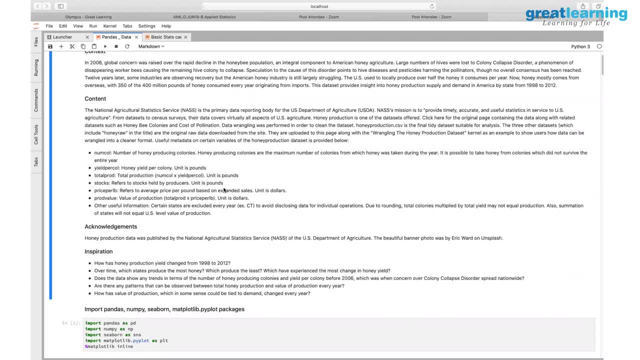 Then stocks refers to stocks hold by honey producers. This is the number of stocks they produce, they have in the market. This is the stock market type. So then price per LB: what is the rate of that honey being produced And the production value of that particular one, which is again a multiplication of total production and price per LB here. 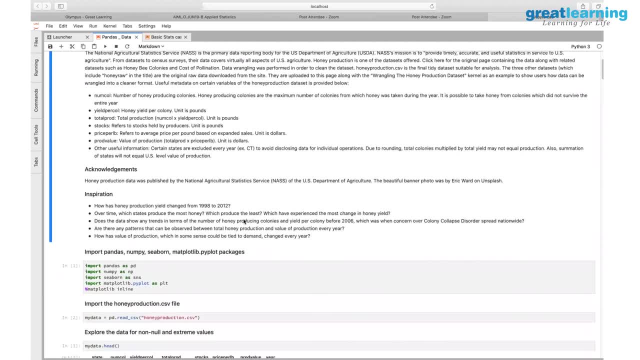 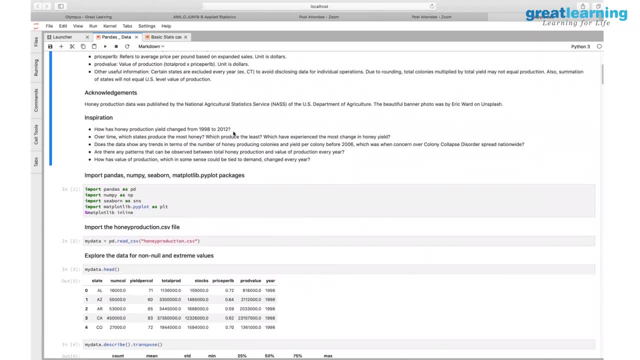 Then some other information about states, categories and everything. That's primarily the data. So the questions we want to understand is: how has honey produced yield changed from 1998 to 2012?? One thing: They want to understand the patterns of honey production changes happening over a period of time. 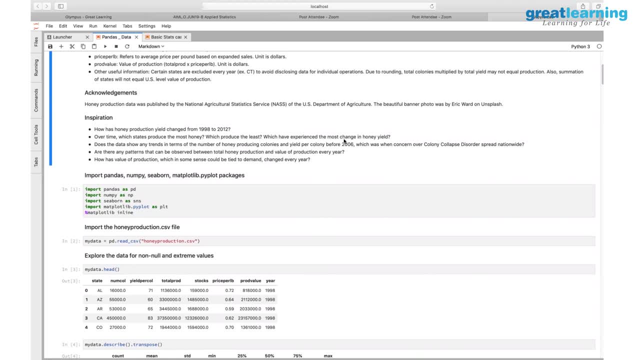 Which states have produced most honey, Which states have leased honey And have we experienced which states have experienced most Change? Can we come to that? It is about now. we talked about the exploratory data analysis earlier, So this we are getting there. 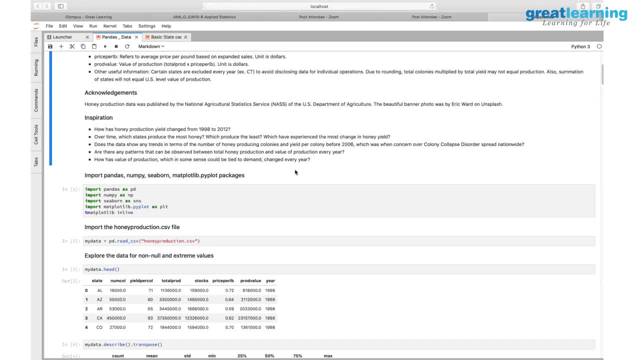 Now we're trying to break the data into some kind of a meaningful information where we can form our hypothesis. So then, does the data show any trends in terms of the number of honey producing colonies before 2006?? Which was the concern over colony collapse? disorder spread that happened. So, basically, there is a natural thing that happened, natural calamity or whatever you call the term. So that happened. And then there is the thing where the colony collapse disorder happened, because of which the honey producing bees, the colonies, have started going down. 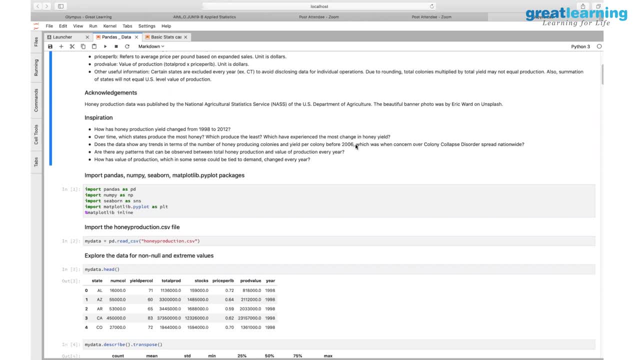 And that has an impact in 2006.. So what is the difference between pre-2006 and post-2006?? Then, are there any patterns that can be observed between total honey production and value production? How has the value of production, which in some sense could be tied to demand, changed every year? 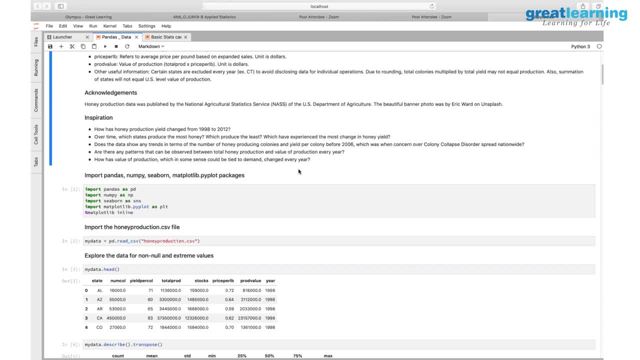 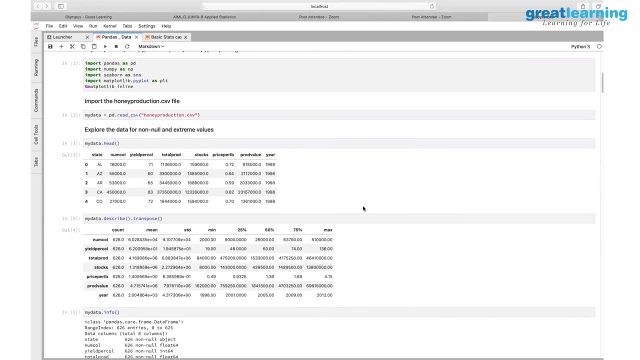 These are the five different questions they are asking for. We'll try and answer as many questions as we explore through the data. So, given that I assume you have familiarity with the code- basic pandas and everything, I'm just quickly running through. 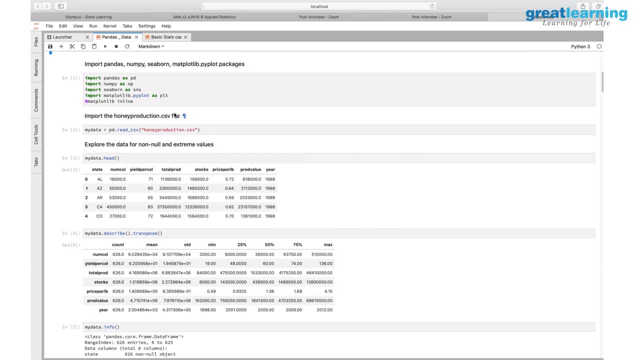 But anyone has any question related to any syntax or why we are doing certain things, please feel free to ask me a question. Are we good so far in terms of understanding what the case study is? One question is why we put the percentage matplotlib inline. 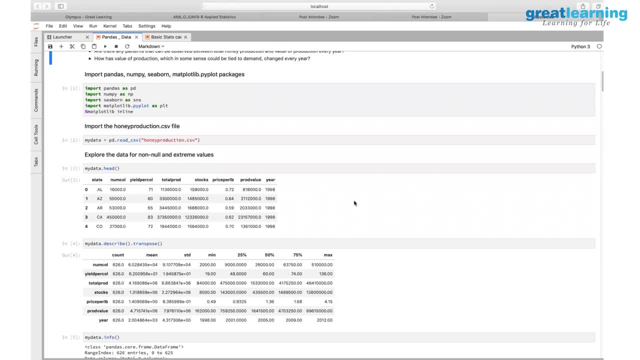 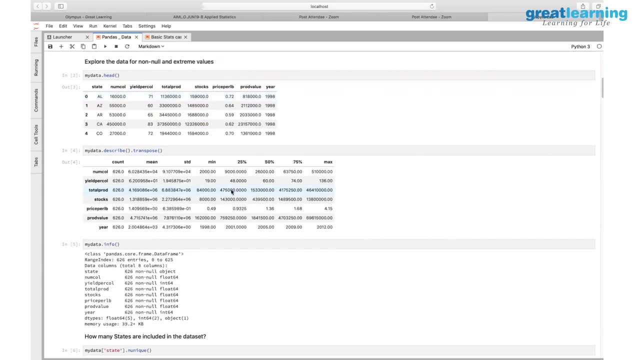 Does it mean to show the graphs inline? I will explain that. We'll come to that. See, Basically it's not a problem. Basically we import matplotlib every time, Just to quickly answer so that we close the question there. So let's say, for example, you have your graph. 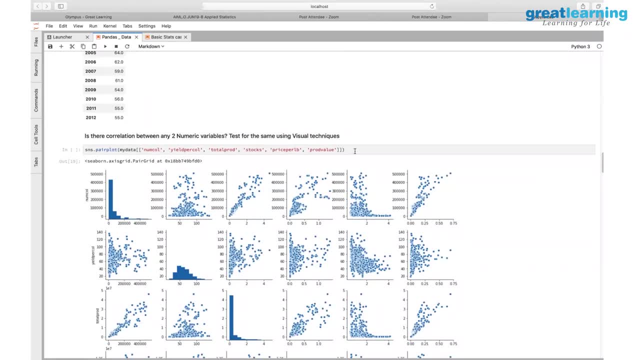 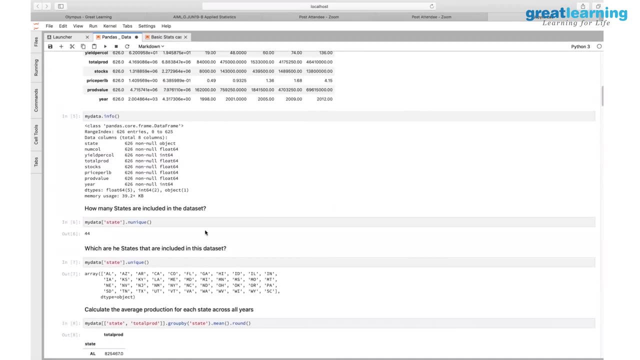 We say snspairplot. You put this. The moment you show this, a map gets created, But the map is not shown to us. You have to explicitly say that pltshow. Unless you say pltshow, the graph would not be displayed. 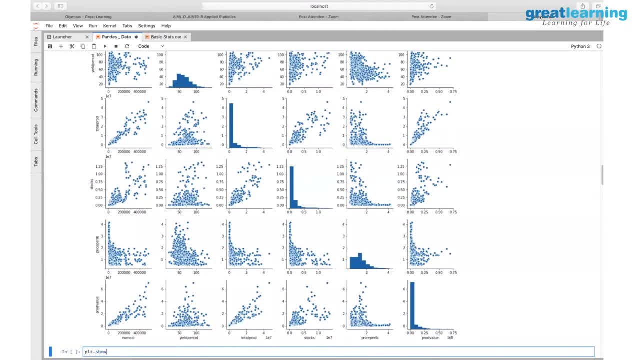 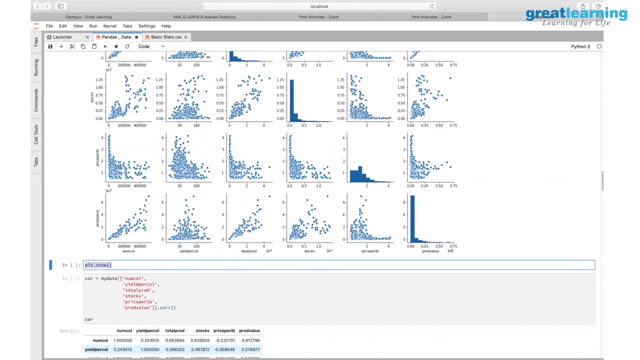 You should type something like pltshow. Then the graph gets displayed. The graph will be in the memory. You have to type this, So every time you create a graph, the graph needs to be shown. Instead of that, you do matplotlib inline. 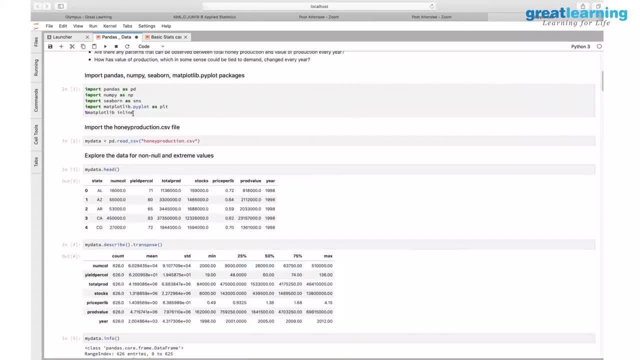 This particular syntax that is out there at the beginning. This takes care of displaying that image automatically. You don't need to explicitly type pltshow every time. Is that clear? Yeah, Got it, Ram, Thank you, Thank you. So now we are importing pandas. numpy seaborn matplotlib. 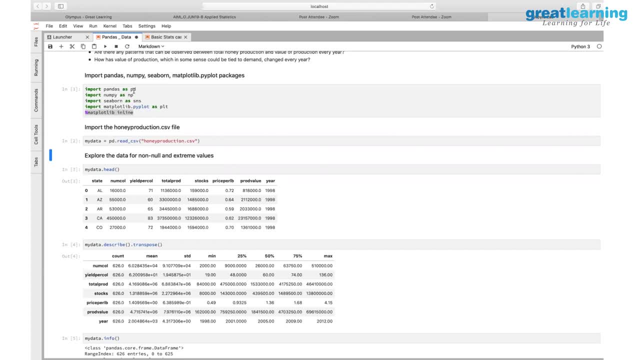 These are the four things that we need. Pandas is primarily for creating the data dictionary. Numpy is for doing some mathematical calculations as required. Seaborn and matplotlib are primarily the visualization tools libraries that we use. So we're using, as usual, the read CSV function to read the CSV file that is out there. 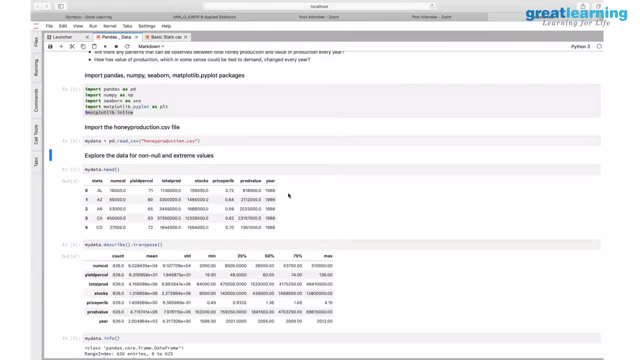 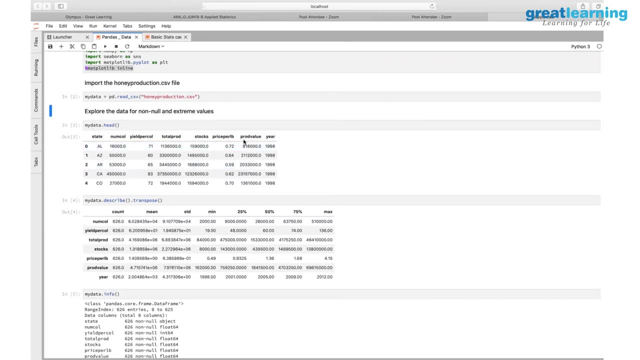 Honey production. But anyways, once we go through that we'll see all the variables here. So mydatahead it has. These are all the columns, As we saw at the top. the state is there. See here: state which variable. 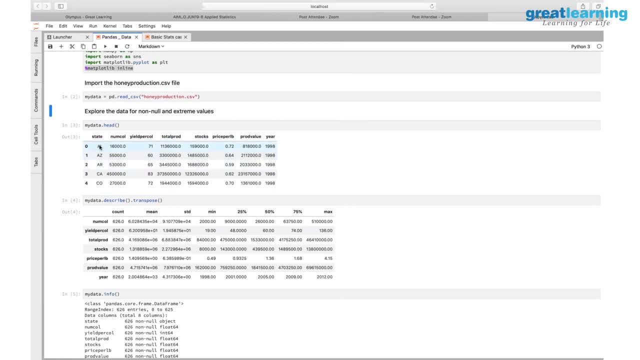 Now connecting the dots back, which variable is state? We discussed the types of variables earlier, Data types and different types of variables. It's nominal category, right Categorical, A nominal variable, basically. yes, It's just for identification purposes. 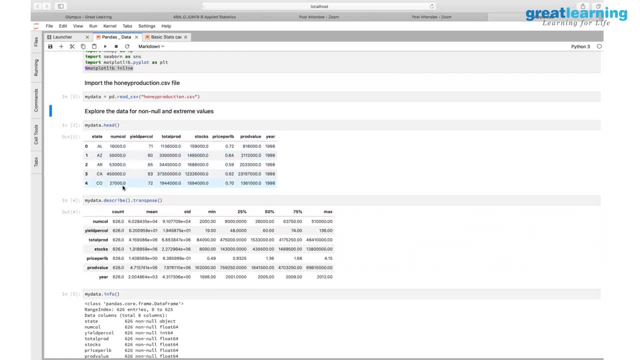 Sorry, somebody has a question. So then numcall, This is a continuous variable, Then yield per call is again a continuous variable. We know total production is a multiplication of these two variables primarily, And then stocks, the worth that these people hold. 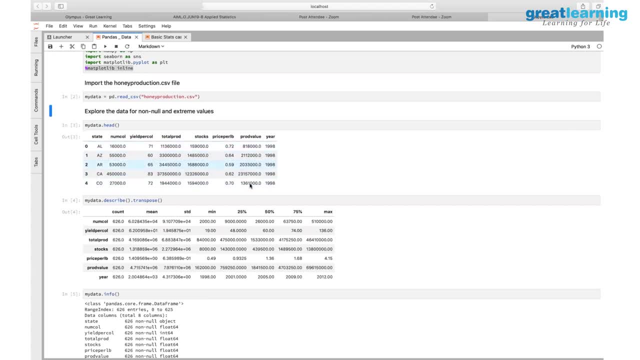 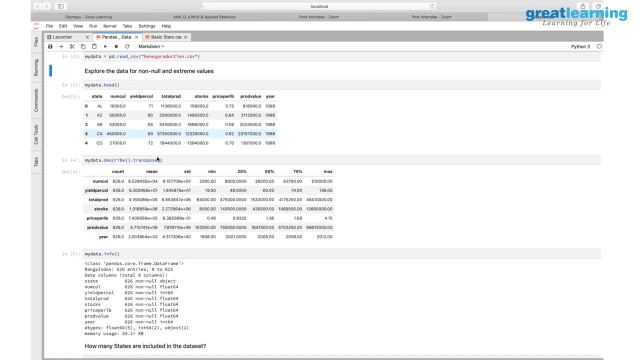 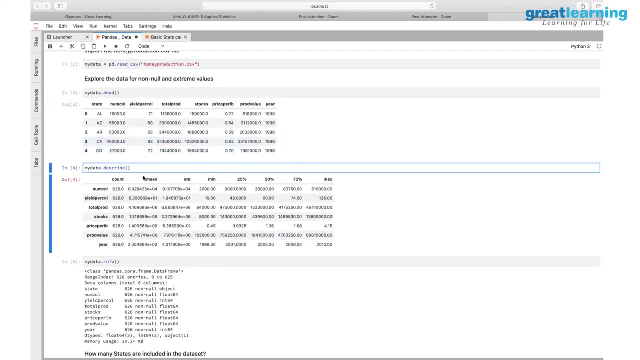 Then price per LB of the production, how much production value and in which year. That's what the data that we have. So now we had I was talking about describe. Let me run this so that I can execute it. It gives the statistical summaries of all the numerical variables that is out in data. 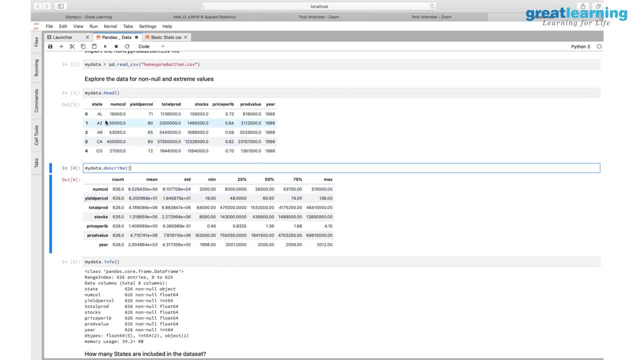 So in this variable, now we have numcall to year, Everything is a numeric variable. if you look at this, This is not a numerical variable. That's why, when you do describe, describe, gives does not include state and it includes. 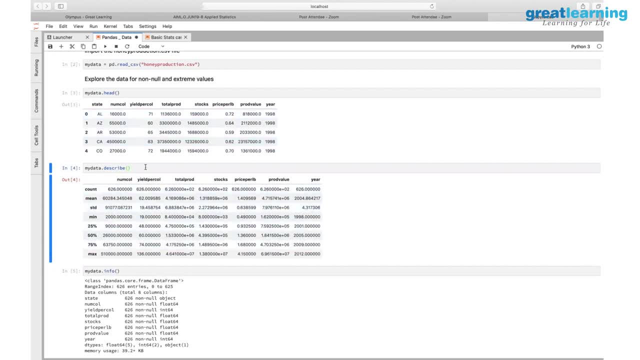 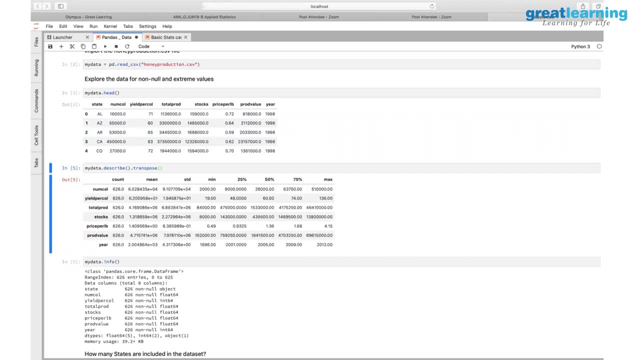 all the other variables, which is numerical variable, And when you do transpose what happens, It just transposes the data display, Nothing else. The count and these things comes horizontally And these variables comes this way. But what if we want to see the state column also? 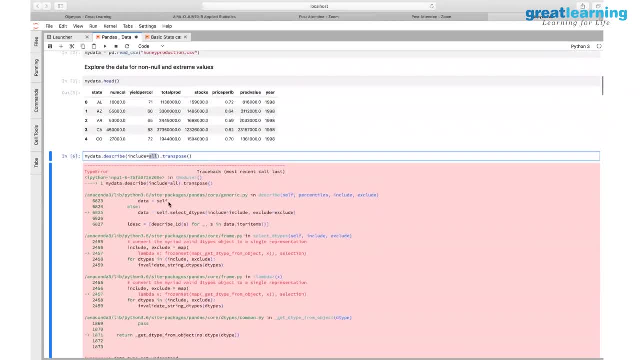 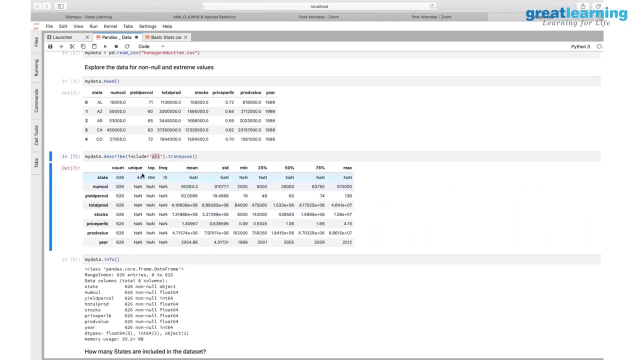 I think all you need to put in the quotes- I think right Quotes- yeah, yeah, yeah. And now I include State. Thanks for that. So if you include state, so how many unique states we have? That also, you can get the sense. 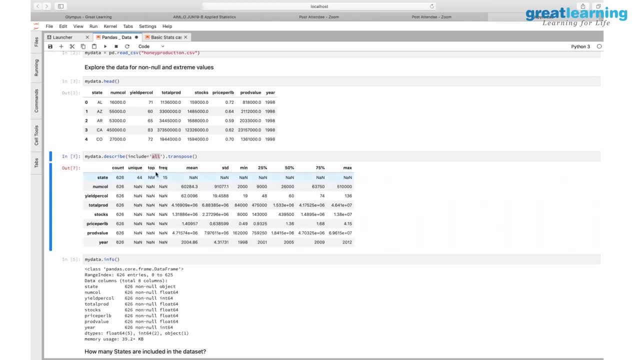 How many unique states you have, Which is the top state, That is the maximum frequency occurring And how many times it has occurred. That's all the data you can get about a nominal variable, So that none of these other things is possible as a numerical analysis. 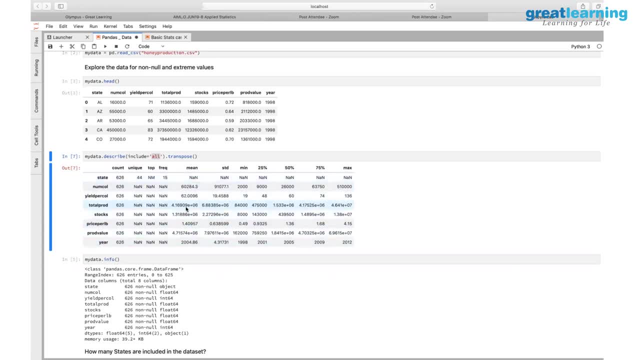 Whereas all other variables are numerical variables And you can get all these kinds of data And interestingly, for the numerical variables, it does not provide this unique Top and frequency variables. in this particular one, Is this looking clear? But just to see, for the year it does all these calculations. 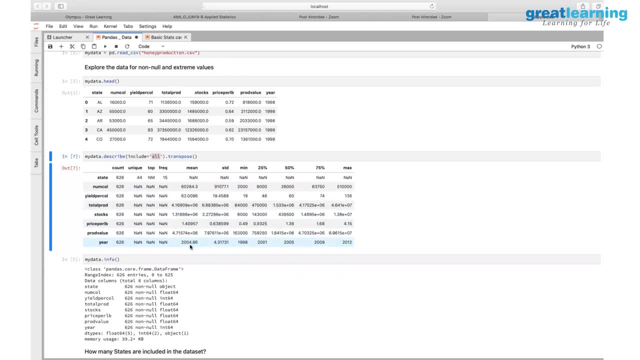 It is calculating the mean year, which is nonsensical. It doesn't make sense of calculating the average year types. There's no standard deviation for the year, Unless you convert the year into a different of a numerical form which is more meaningful for you. 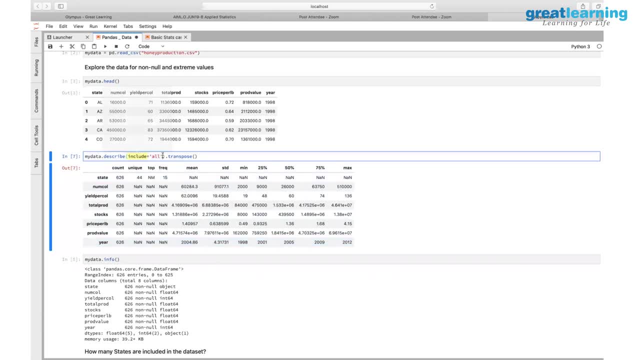 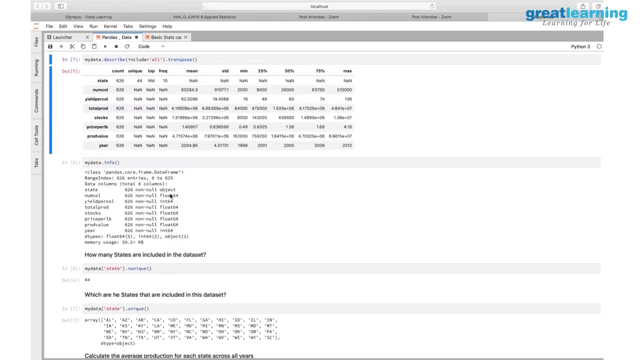 So while it calculates, we might not get value for all, So we need to apply our judgment as to how do we apply that, The data types, as we have seen here. So these are all numerical or float variables. This is an object. 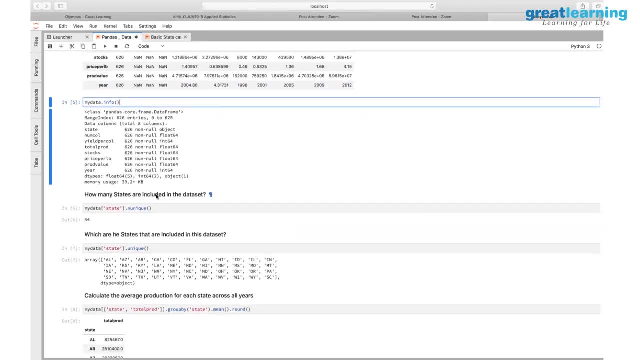 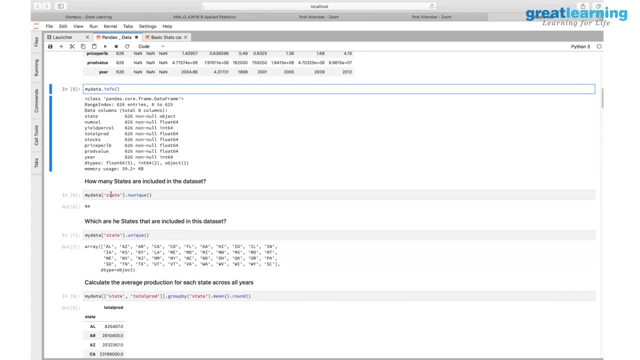 The info gives just that much. Now the question is how many states are included in the data set. We have seen it here when we entered state 44. You can get through this, Or you can just say my data for the state variable. 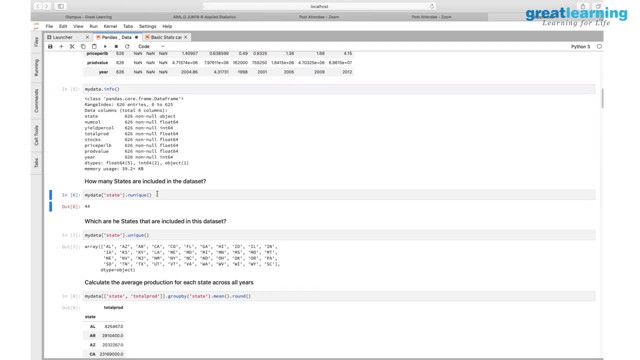 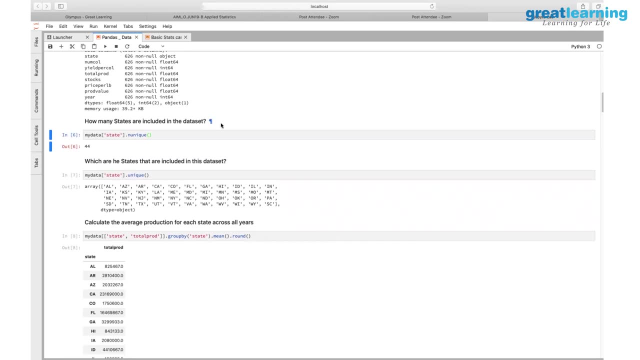 And unique. How many unique values are there? And unique gives you the unique values for that particular column If I want to know how many times each state is appearing. So I know some states have appeared as high as 15. But I want to know it by state. 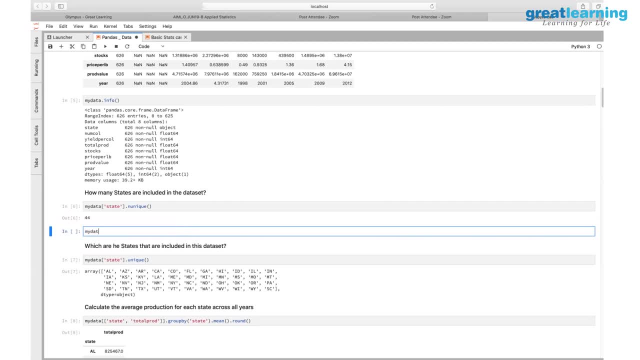 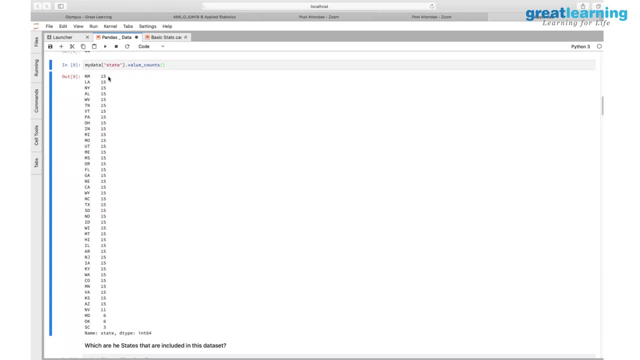 Is there a way I can know Value counts? Yes, Absolutely, You're great. The value counts gives that. So NM, as we have seen there, appears 15 times, Then LA 15. NY 15. All these states are appearing. 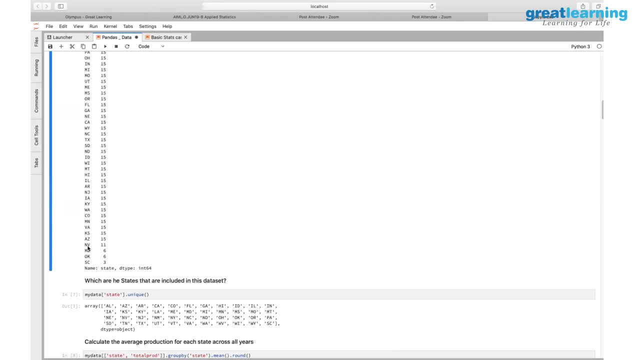 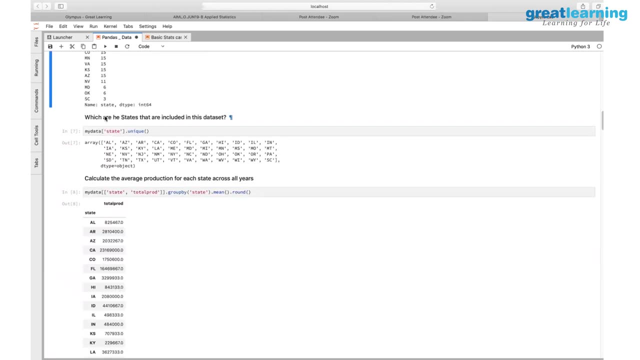 Majority of those states appearing 15. And NV is appearing 11. SC is the one that appeared only three times. That's a simple way of looking at it. Okay, So then, which states that are included? Which are the states that are included? 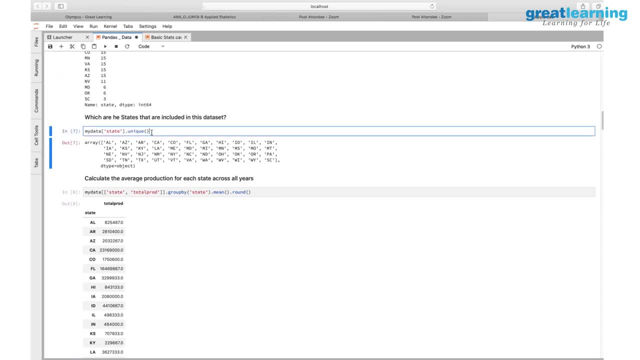 So unique N unique gives you the number of that particular one. Then which state? Unique display of the particular states. This is the one You can get. all unique states that are there. This is the unique value it gives. Now calculate the average production for each state across the years. 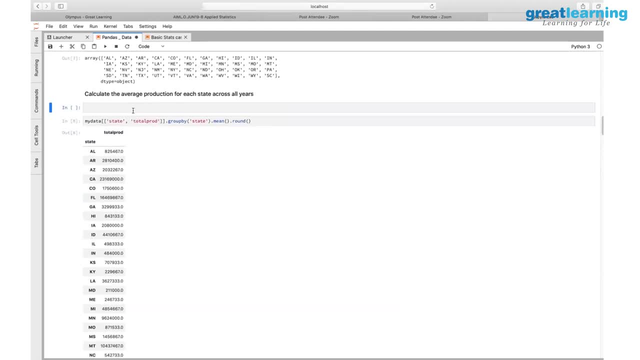 So this is the simple question that looks, But sorry, I want to add one more column here, One more value here. So let's say, for example, you just want to calculate the average of production, total production. So my data. 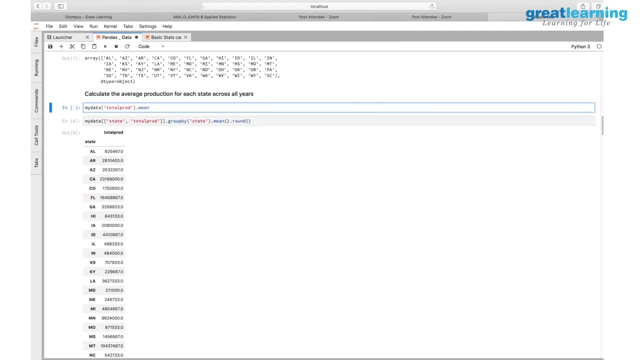 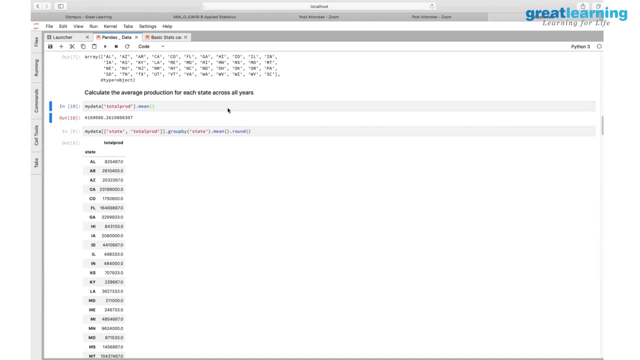 If I want to just calculate the mean of this one, I'll get the mean for that particular variable alone, But that gives me the whole. But the question for us essentially is to calculate the average production for each state. I need to do a group by for that one. 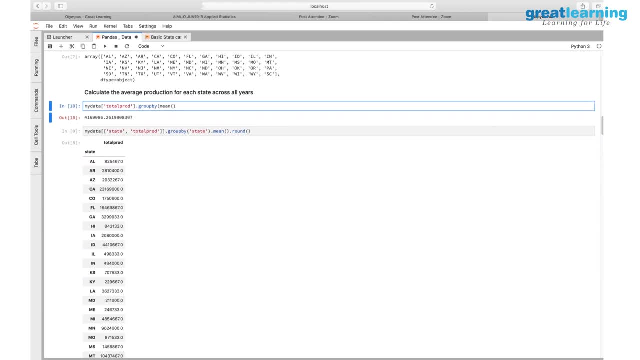 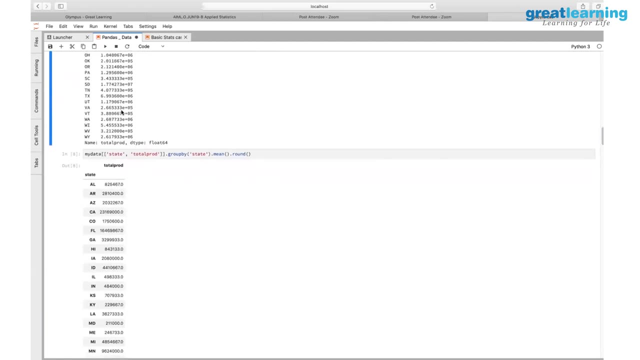 I'm just trying to demonstrate it how we came to this particular one. simply, That's the mean for each of the states- Mean or average for each of the states. But given that we are getting so many dismels, we don't want to do that. 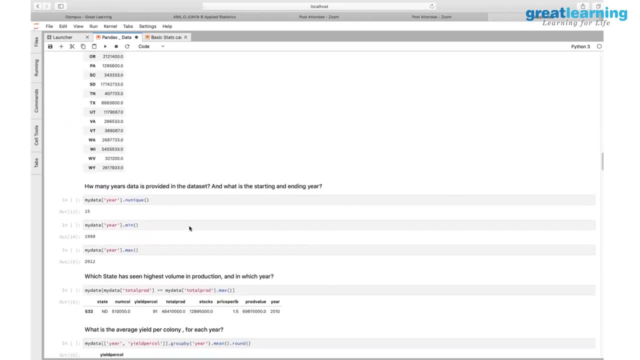 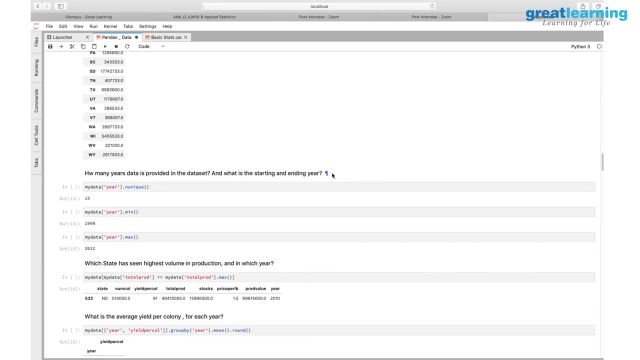 You use a round function, You just get this data. Is this clear how we are using that Right? So then, how many years, of how many years data is provided in the data set, And what is the starting and ending of the year? 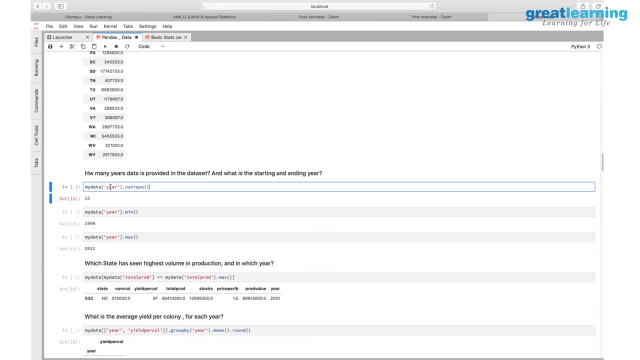 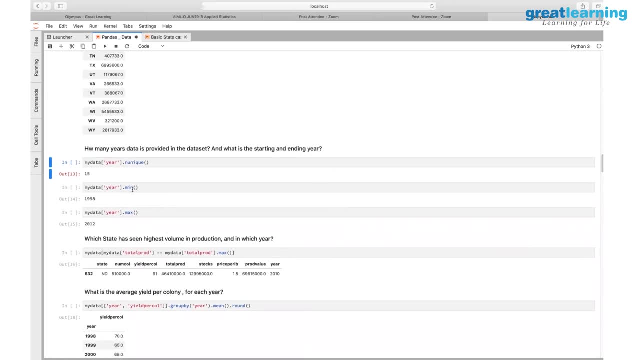 So this is what we are getting. How many years of data? for the year column, You calculate any unique, You get the values. 15 years worth of data is what we have. The lowest of the years. You calculate the mean value. 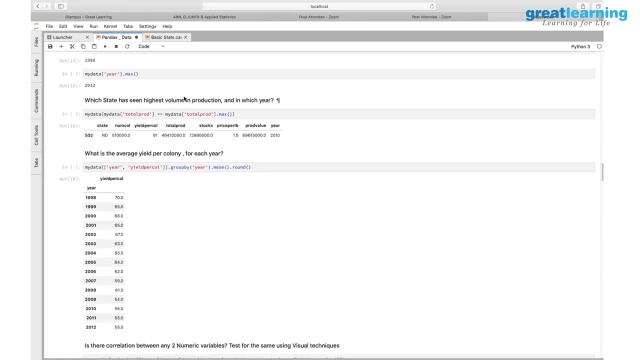 You'll get max value. You'll get the maximum state. which state has seen the highest volume of production? My data production for the total production column. You can get the maximum value. You will get that particular one. So if you want to get all, 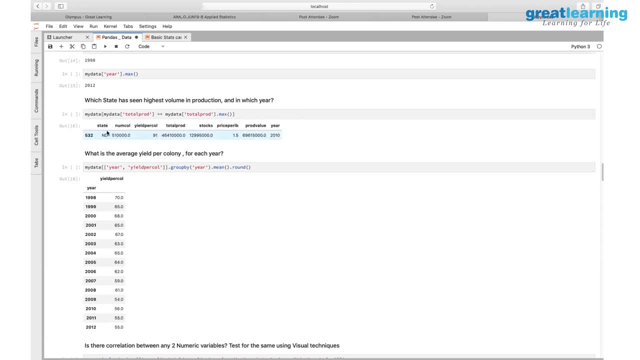 you just use just this much, You'll get the value. You want to get the whole row. This is the syntax. You want to just apply this condition, So the total production value is equal to this particular one. For that, give all my data. 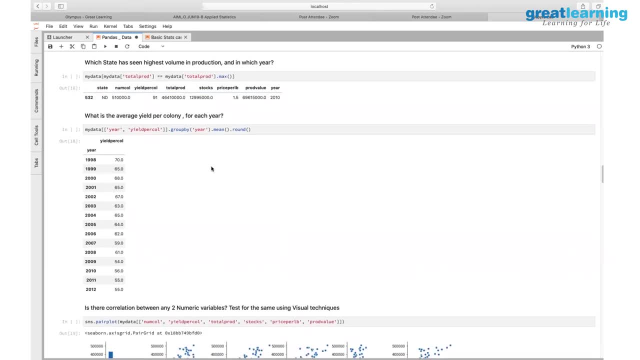 It gives you the whole record for that particular one. Then average yield per colony: Again you apply the same things. Instead of using one, just one variable, you can use two variables also to get the details and you group by year there and get that particular data. 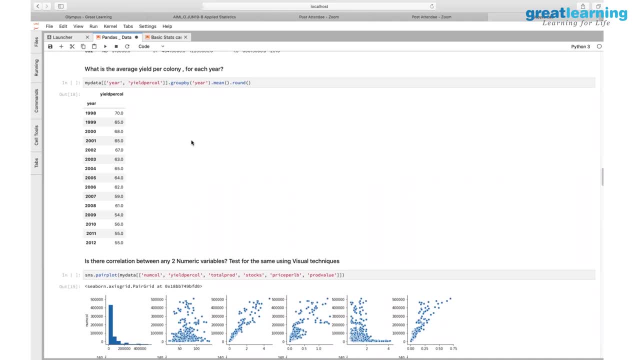 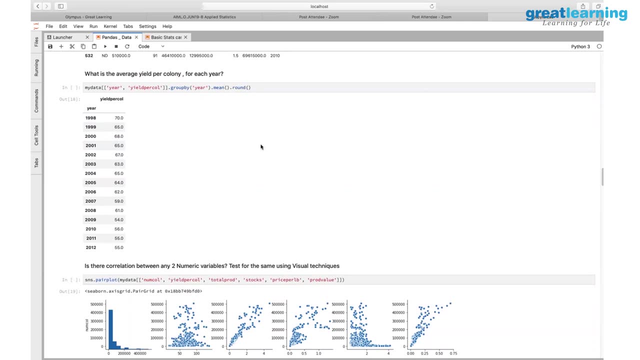 Because you're grouping by year. you will include the year column into this particular one, Then the rest of the process. what you are doing for yield per call is exactly calculating average and rounding it. This is how you get it. So now the question. 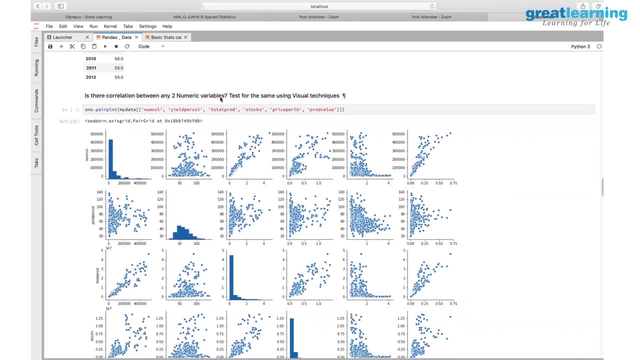 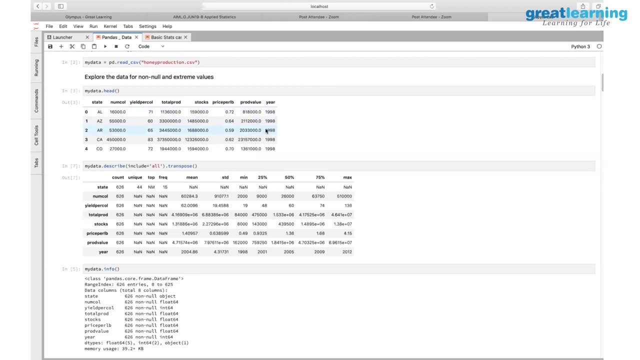 This is an important question: Is there a correlation between any two numeric variables? So how many numeric variables? we have seen 1,, 2,, 3,, 4,, 5, 6, 7 variables Out of the eight variables that are there. 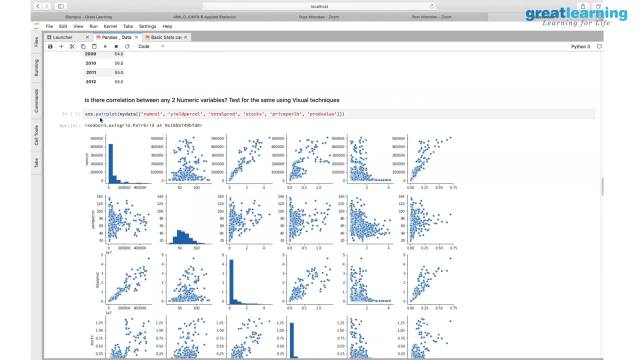 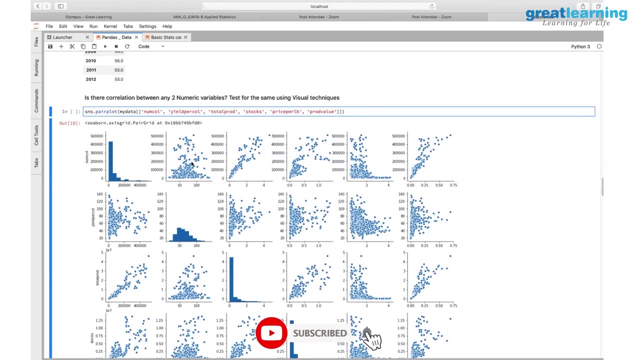 Is there a correlation between eight numeric variables. So SNS is a Seaborn library and it has a function called pairplot. Pairplot gives you scattered plots of all the variables, one with every other variable that is out there in the dataset. 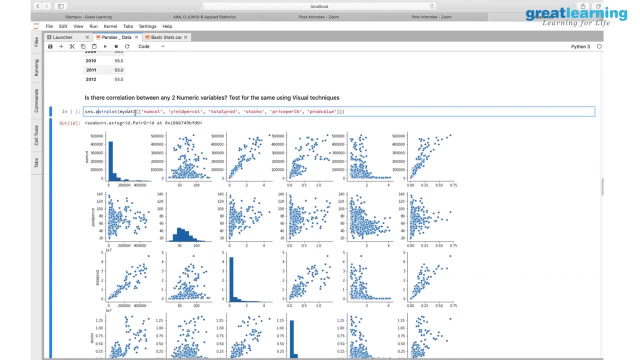 If you use pairplot of my data, essentially it more or less gives you the same thing. But the challenge that we see there is you have a straightforward variable which is non-numeric, So it doesn't gel well. So that's why we exclude that variable. 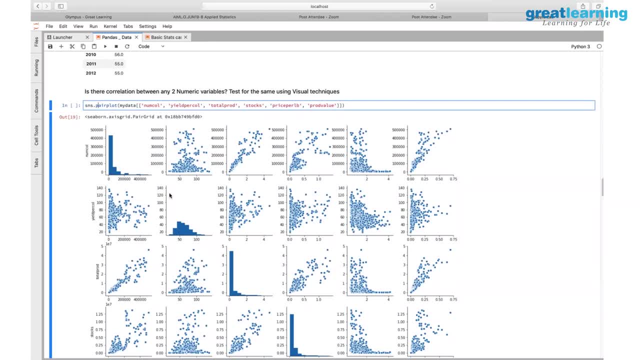 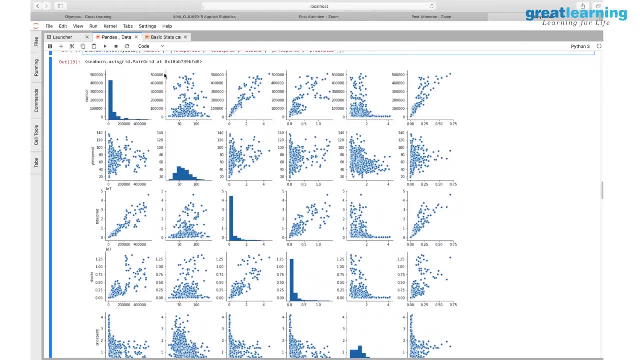 and include all the remaining variables that are there in the data. So now, what is the pairplot doing? So it's, if there are n variables, it produces a n by n grid. So every variable with other variable, But if the first chart is numcall, 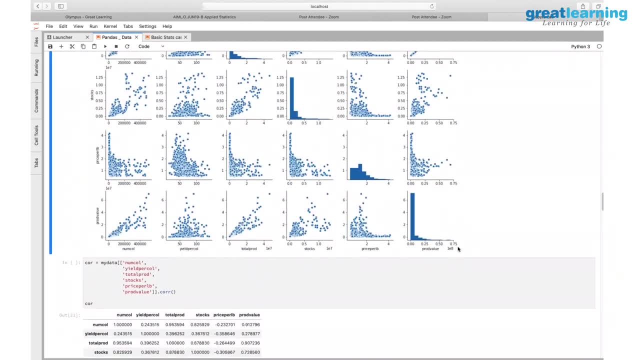 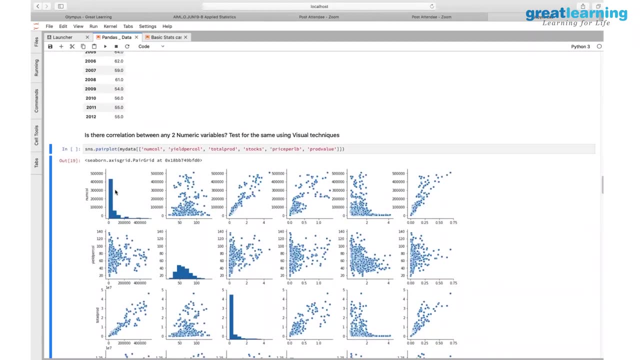 and these are all the variables. and the same variables are listed in the horizontal listing also, So there is no way you can do a scatterplot for the same variable. So instead of that it is replaced with a histogram, So the data distribution of that particular variable. 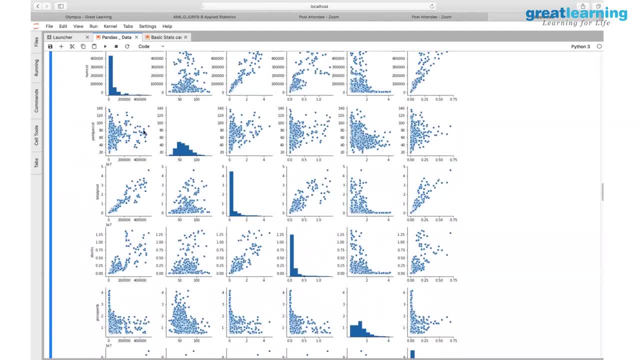 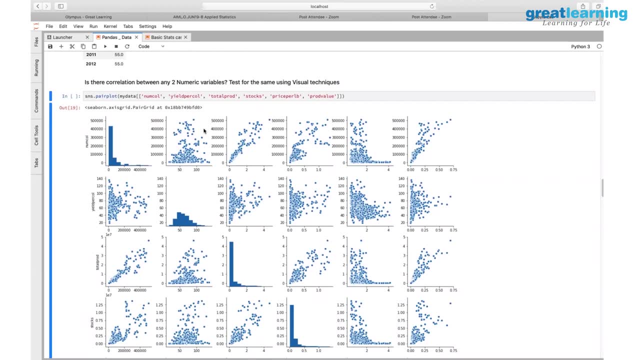 that is shown in the diagonal and all others, a scatterplot is shown. So how do we interpret scatterplot? So this data distribution should give you some trend. If you just take this numcall variable with the yield per call, what is this telling us? 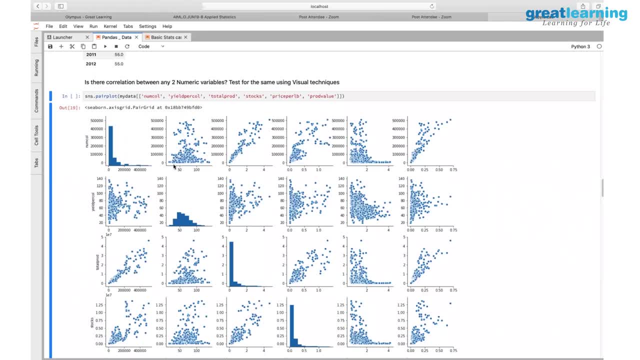 Majority of the honey producing colonies have very low listing. Only a few are scattered in the upper echelons. Otherwise, majority are concentrated just in this particular one. And what is the third variable? Total production. So production versus number of colonies. 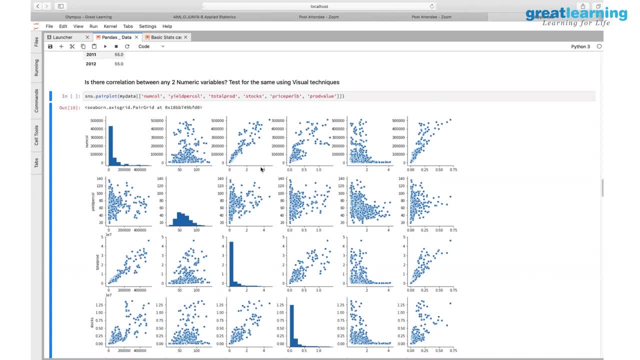 As the number of colonies increase, the production also increases. So this is pretty much a linear relationship. that is out there, You can see. So now, if you have heard of the correlation- anyway, we have touched upon the correlation, We will touch upon correlation. 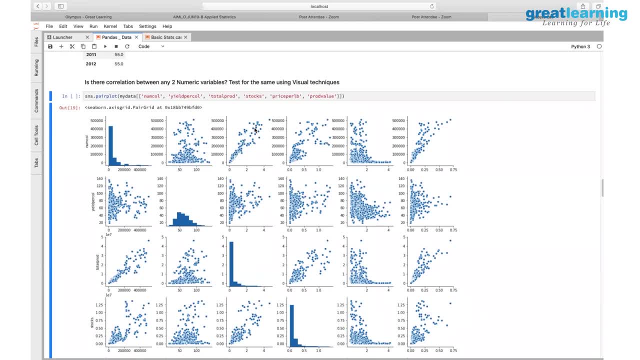 when we go into statistics. But now that you got, you know, watched the videos already. I'm asking: what is the correlation here? If somebody has a sense of it, you can answer. What is the correlation in this scenario? Total production and number of colonies. 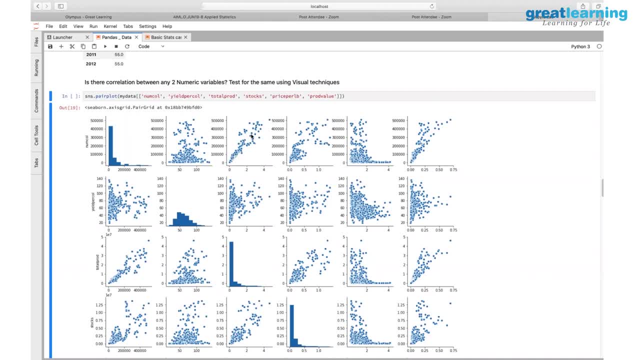 have a positive correlation, right, Positive correlation. So yes, positive correlation right. But can we get a sense of what is? how much is the correlation value? Closer to one? Closer to one? Absolutely, Because this is pretty linear. 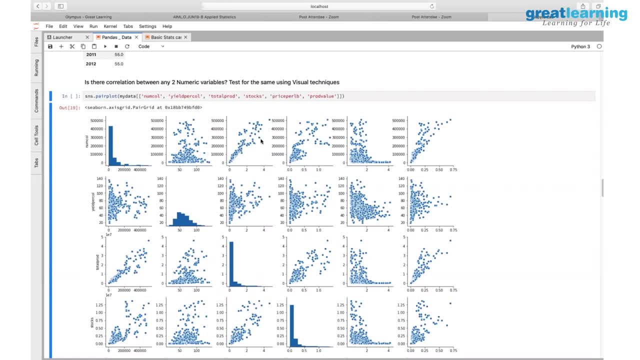 going along the diagonal. So if this is increasing, this is also increasing. This is increasing. So, except for a few points where, even for the low value of this particular one total production, you get a higher number of colonies, This is a pretty linear relationship. 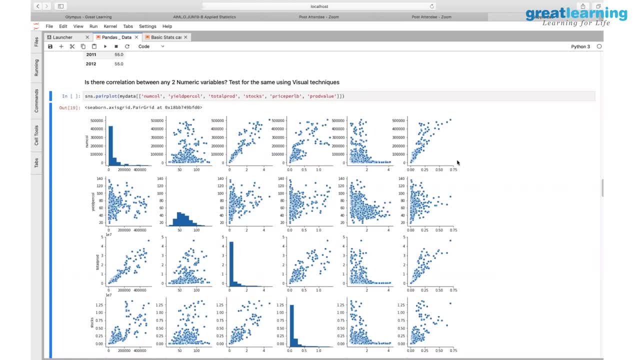 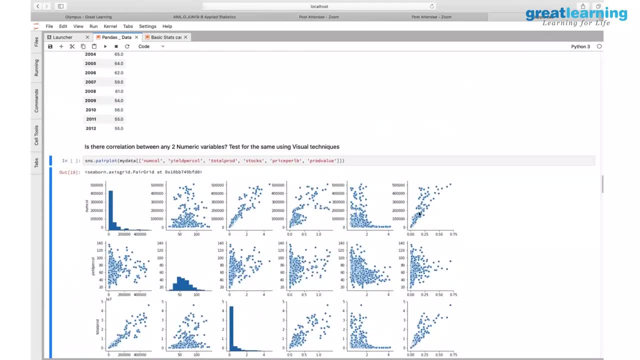 That's what this graph does, But we'll talk about how to interpret the graphs a little later. So this is again another variable: Num, call and production value. So the value of that particular one is also pretty much linear. And if you take this particular one, 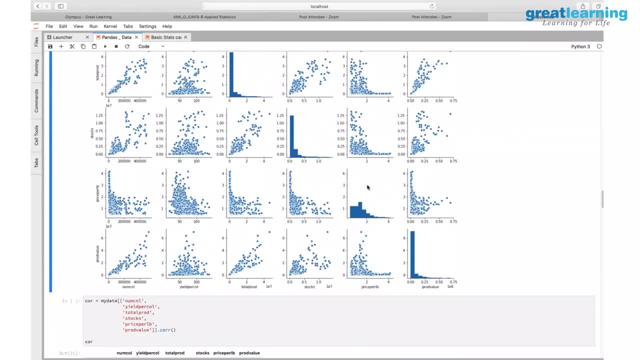 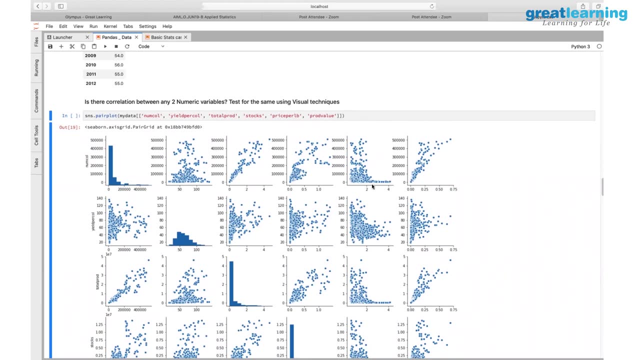 which is this variable, that is price per lb. So this is pretty much constant. Only for very few these things you have a higher value. Otherwise it's more or less stagnated and concentrated in this region. It's only this much variation. 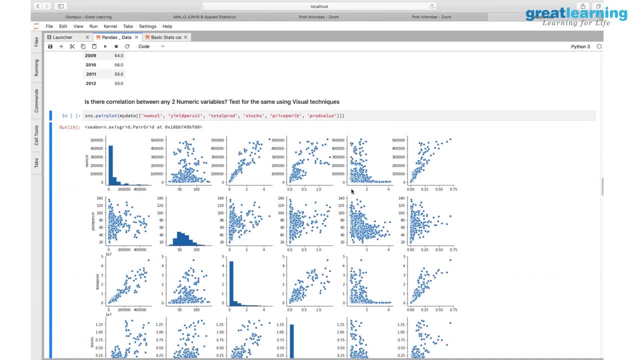 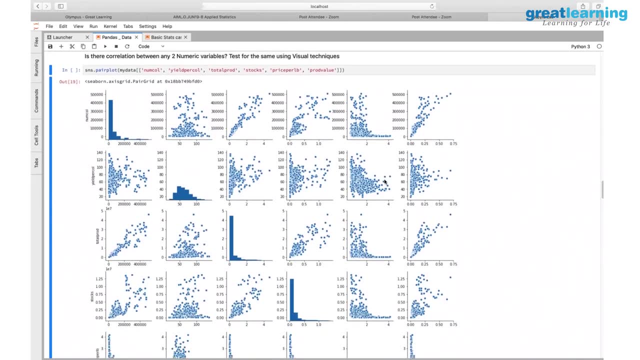 but predominantly in this range. This is very, very acting differently into the things. Now, interestingly for you, this whole pair plot that we are seeing is something kind of a symmetrical. Either you can take the upper triangle or lower triangle, because you see the exactly. 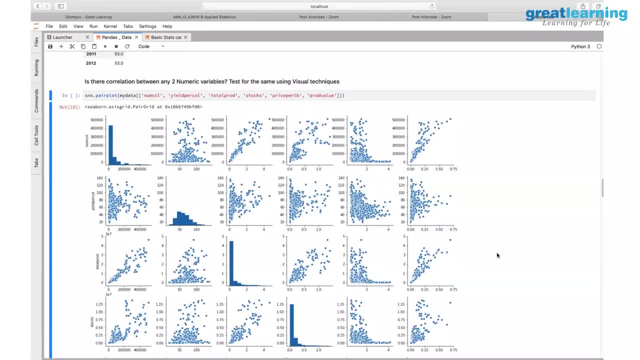 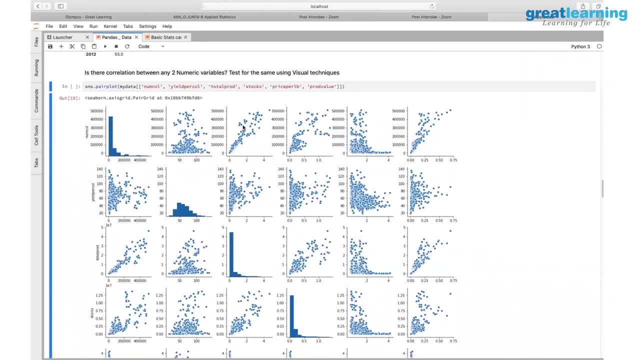 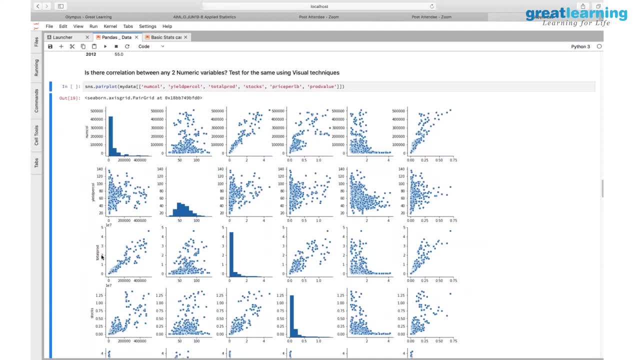 and the same graph here and the same graph here, but labels change. Here it is numcol versus total production, Here this is total production versus numcol. So it's a mirror image, but exactly the same graph. So either you can focus on the lower half. 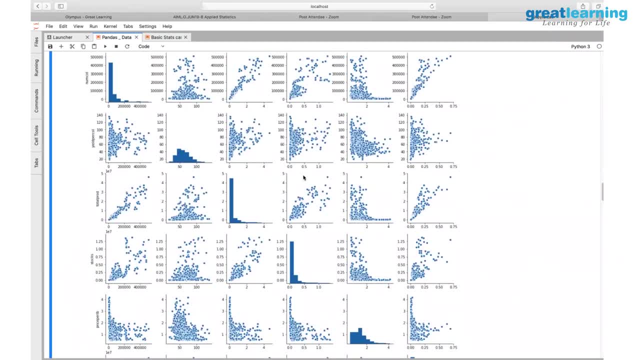 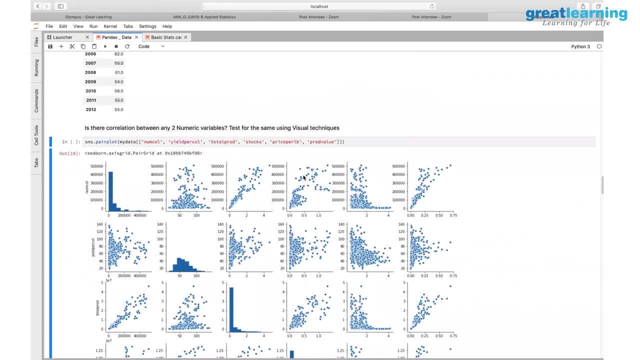 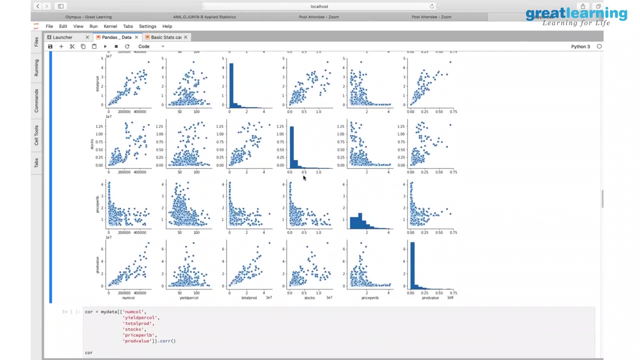 of the triangle or the upper half of the triangle. You don't need to look at all graphs to interpret the information, because it's symmetry. Any questions on how do we get that correlation thing? Okay, We'll move forward, Thank you. so this is the visual representation of this. I'm sorry, question one concentrated. 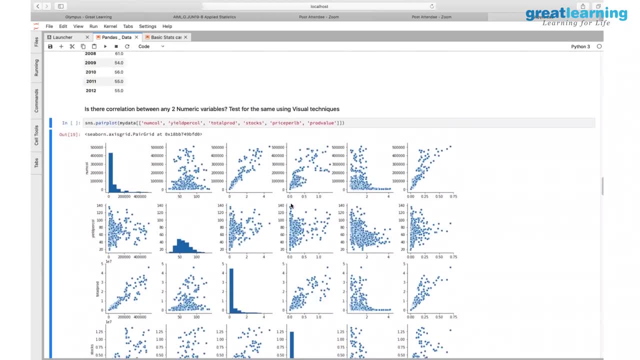 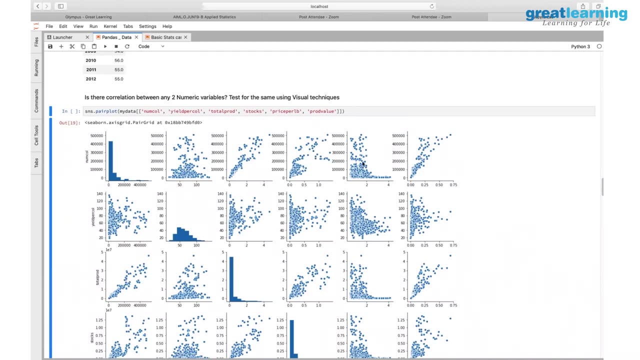 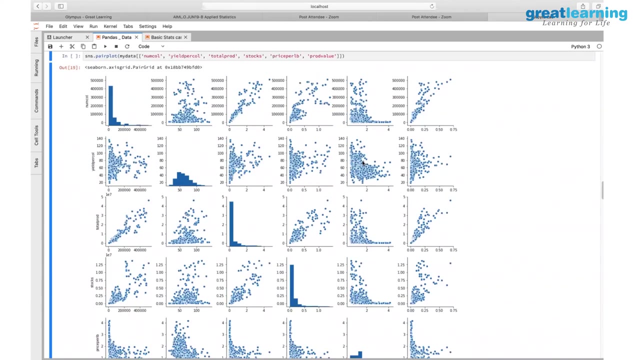 one that is second example: yeah, this one, this one, I fight next, next to next this one. okay, so, let's, let's, let's follow. sorry, yes, it is a voice is breaking. I'm sorry, you're going to hear me. I will type it. yeah, I can hear you know, okay. 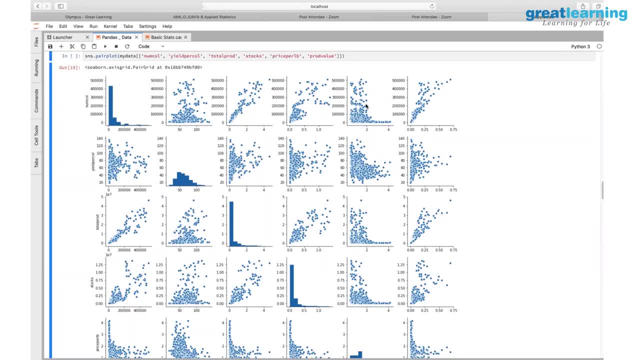 it's like I can hear you know pulse, like a step input, like like that, the relation, or yes, if you look at that particular one, the variation is appearing between this one to this one. so let's see what variable this is, then we can start interpreting this variable. 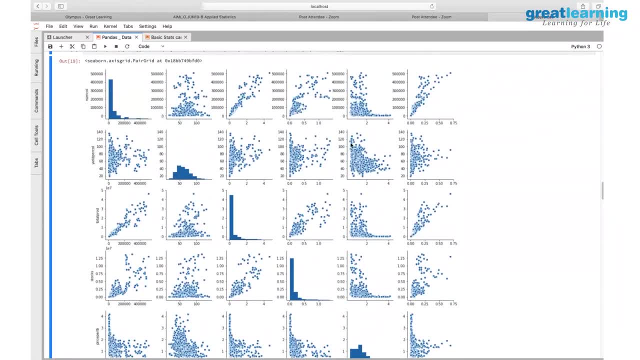 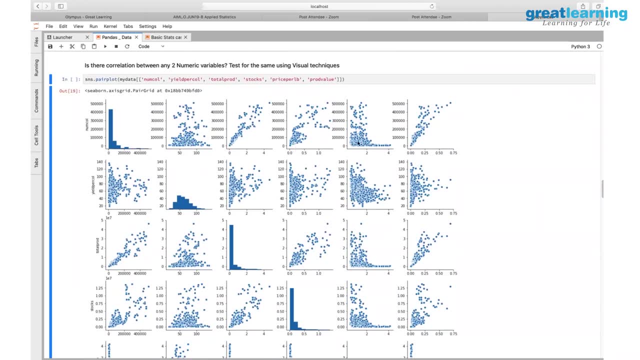 is price per lb. okay, so we are looking at price per lb- how much price for ld is costing here, and this is about number of colonies. so irrespective of the number of colonies as it goes up, majority is primarily concentrated in this zone. you can see my most moment here, yeah, 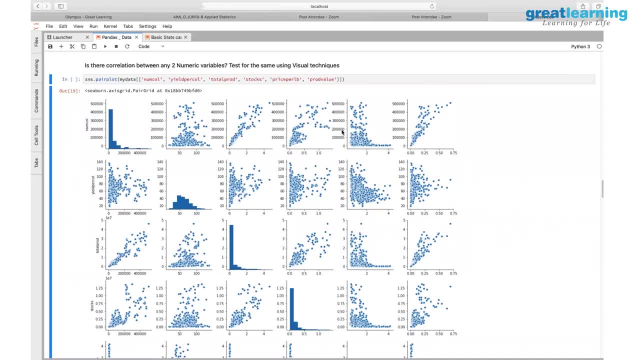 so sort. majority is concentrated in this particular one. so till twenty-thousand number of colonies. the price is within this particular range and just this much after that for very few colonies. essentially the price as you. as the number of colonies are increasing, there is a higher price coming in. there could be any number of factors that are influencing the price variation. 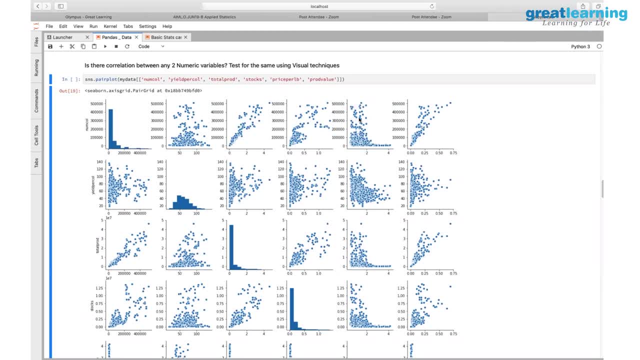 there this thing, so fewer number of colonies are in this zone and here. if, as you move this side, what is happening? the price you are getting per lb is increasing. you are getting a pretty high price compared to this particular one, but there are not many in that zone. what does this tell me? 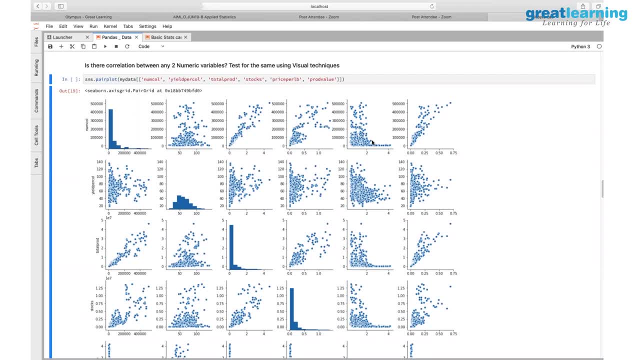 so there are certain of certain colonies which are getting a pretty high price, but those are far and few. there are not many. it could be because the quality they produce it could be very rare in nature, or it could be those are the ones that are going to a high demand place where particularly 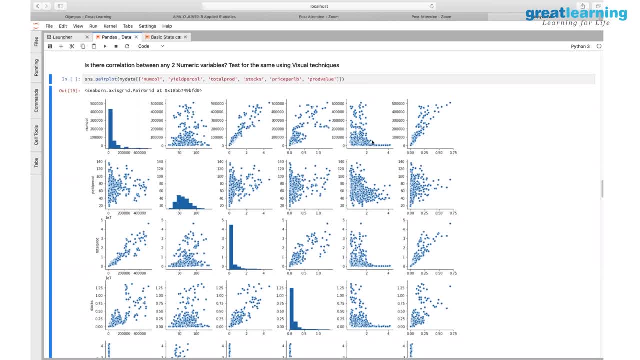 people are looking for that particular type of the thing. whatever the reasons could be, there are very few colonies that are getting pretty high price. otherwise, more or less everything you are getting is very high price compared to this particular one, but there are not. many is concentrated in this zone. not much variation is happening. price because of the thing that's. 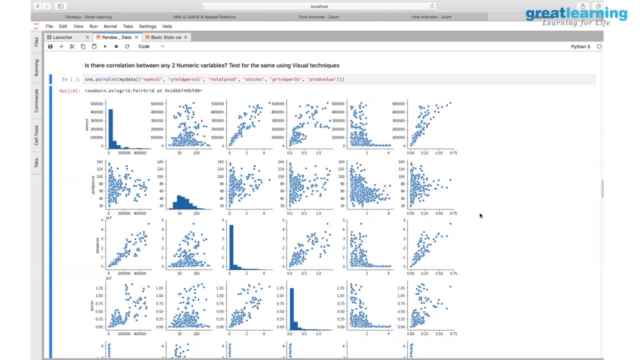 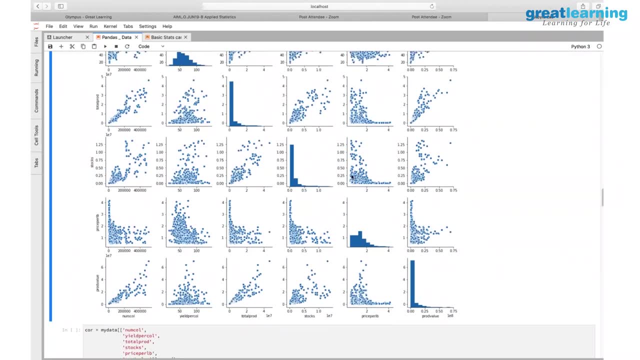 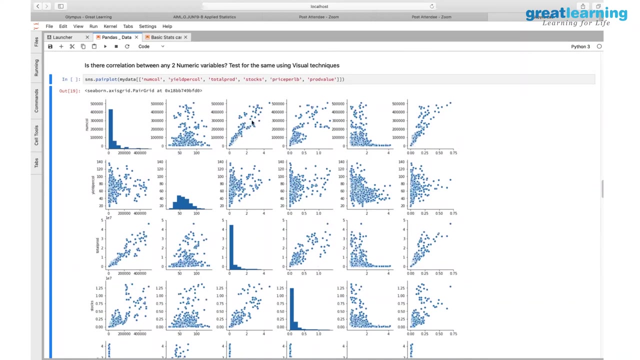 the interpretation we'll get there. does that make sense? yeah, right, okay, so now the important part here is at this point, as i, as i asked the question earlier- i think prasad someone answered- what is the correlation here? essentially, yes, it is a positive correlation. the correlation value is closer to one. 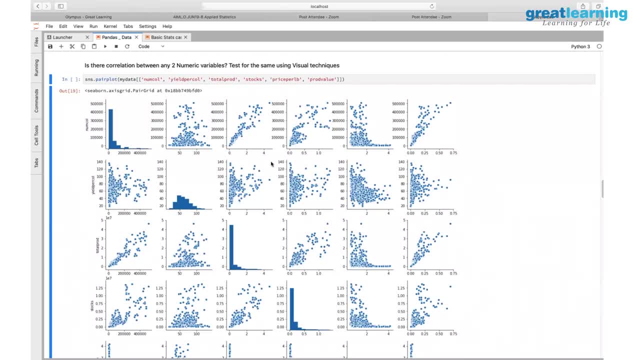 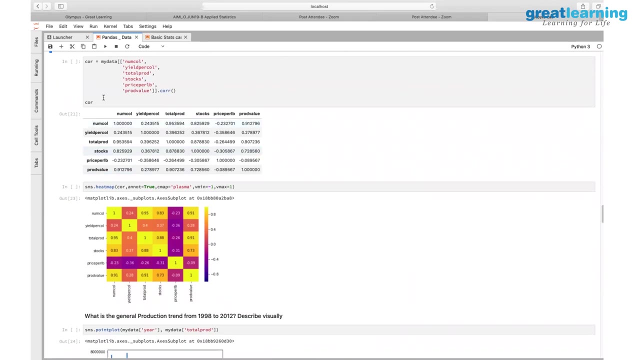 essentially visually you can see on this particular one. but if i have to see exactly the correlation between each of these variables, what is the numerical value of the correlation that exists between these variables? i can just do a core function. i create a heat map, i can do a car or 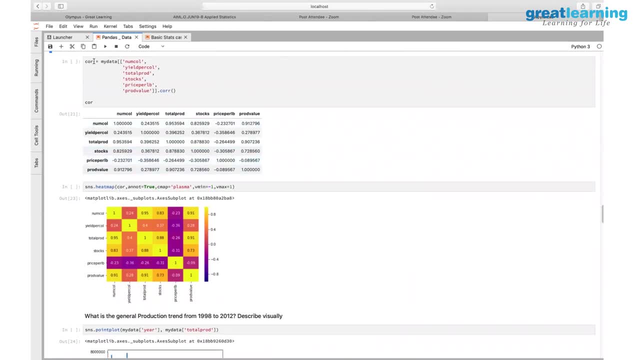 heat map. whatever i can do and apply that particular, see here i am creating an additional separate data set with all these variables and i am calculating the correlation on this particular one and storing that in car, which is this table. so this is nothing but the correlation between 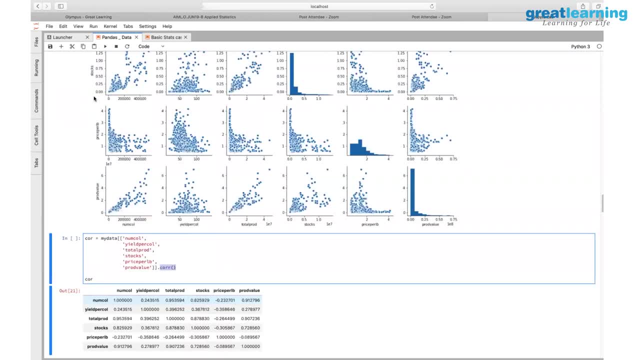 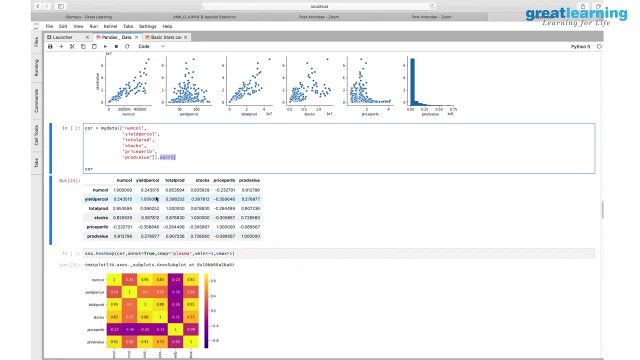 the same set of variables that we have seen, because a correlation between the same set of variables is the same. so the correlation with the same variable, numcol versus numcol, is always one. so that's why, you see, the diagonal is always one. and then again the symmetry that i talked about. 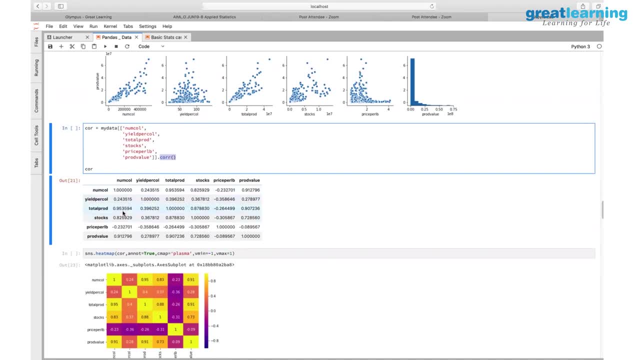 point two, four, three, five, one, five. point two, four, three, five, one, five, nine five, three, nine five, four, nine five, three, nine five, four. here also you can look at the lower half or the upper half. essentially, okay, uh, did you understand what i mentioned by car? so it is about this car is a. 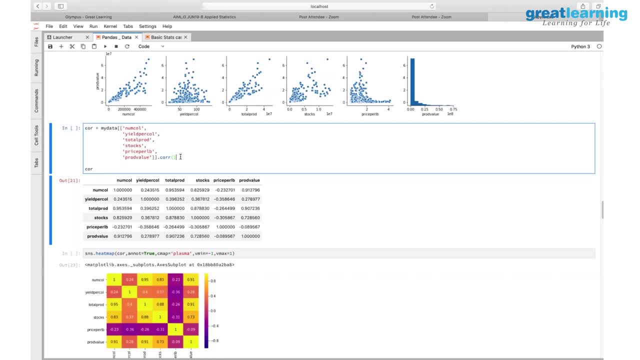 function used to calculate correlation. it returns the correlation for a given set of variables. if you take two variables and do car, it just gives correlation for those two variables. here i use six variables. it is giving correlation for six variables. i'm just not hearing any notes. i'm 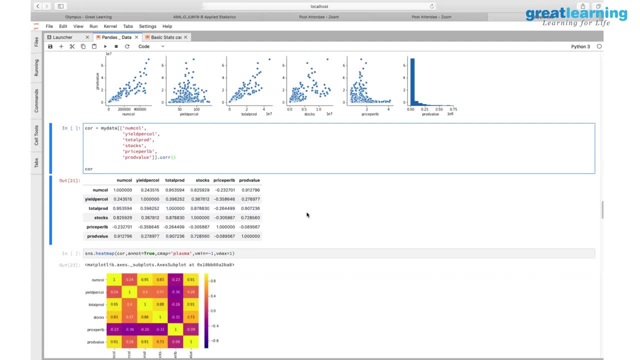 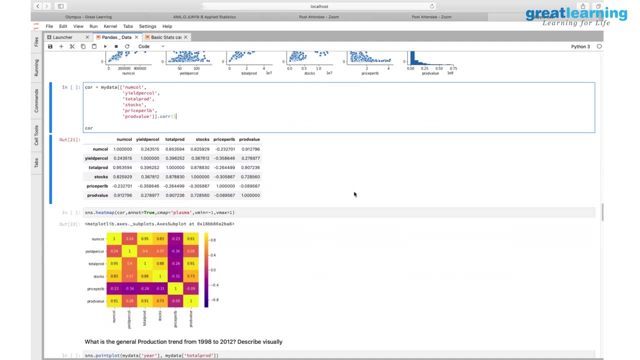 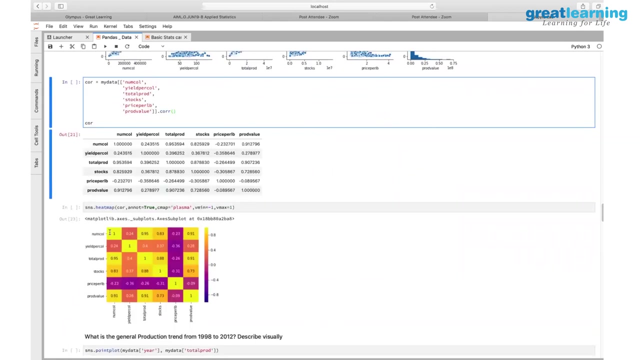 actually taking that, as you understood. but i'm wondering: okay, uh, so the as the value is closer to one, yes, it means it's. i can hear: okay, as the value is more closer to one, uh, does it mean it's uh strong now? yes, uh, if you see the correlation, good question, so let's come here. so, if you take this numcol variable, 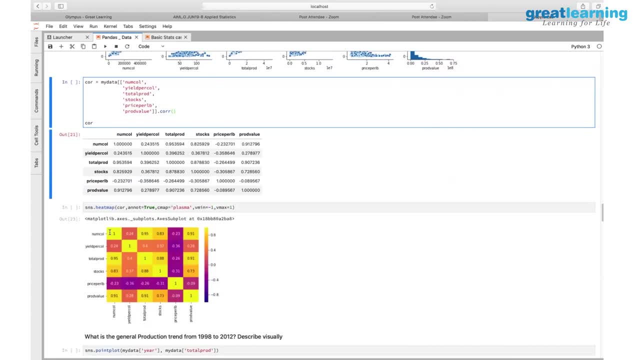 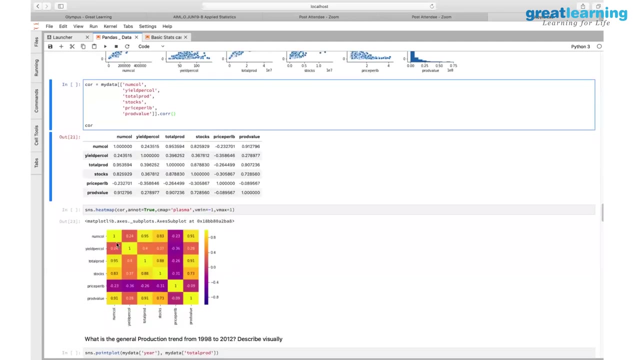 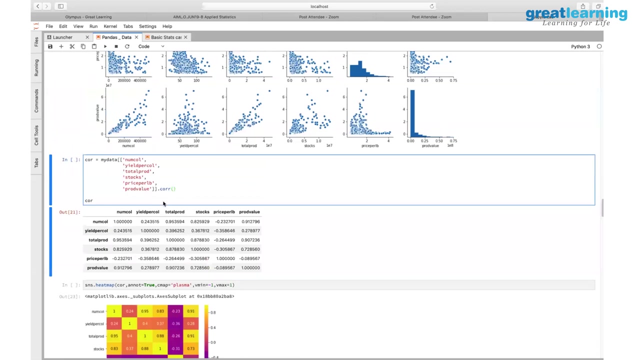 here: total production variable. what is the value we are seeing here? 0.95.95. so yes, take that value, for example, and take yield per call versus numcol. what is the correlation? we are seeing? 0.24, 0.24, 0.24. so let's look at both the graphs. so this and this is the same, this is 0.24. 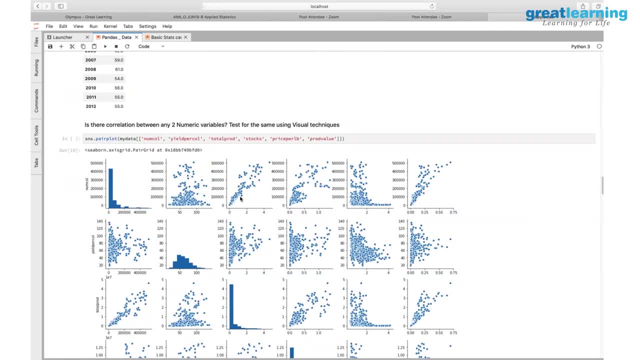 0.04, 0. climbs this script. this is 0.14 essentially. and what is the correlation here? we saw 0.95. so this is pretty linear in nature. it is going along the diagonal between the two things. so if the line goes exactly in this direction, uh, diagonally which? 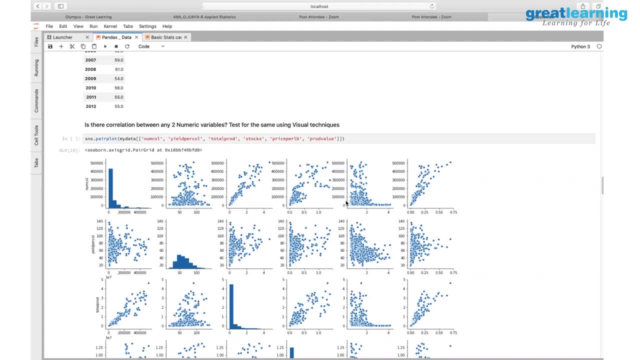 means this value increases, this increases. as this increases, this also increases. it is not like this is increasing, but this is not going. so if you look at this particular one, this has gone up to: only E is not increasing, it's just this much. whatever the variable, i'm just using price per lb column. 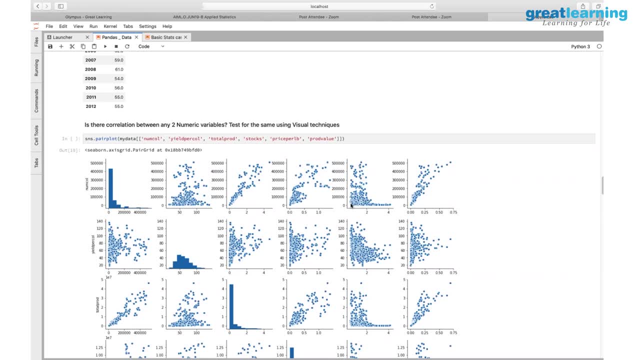 it is only going this much, so this cannot be linear. so it has gone maybe linear to this part, but beyond that there's nothing. it is only one directional that is not growing. so the correlation in this particular one you can see, for example, what is the correlation we are seeing minus 0.23. 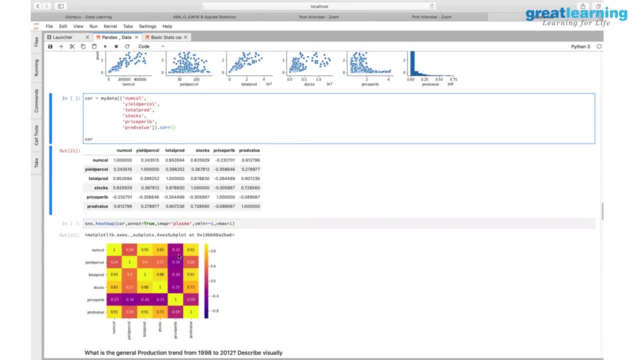 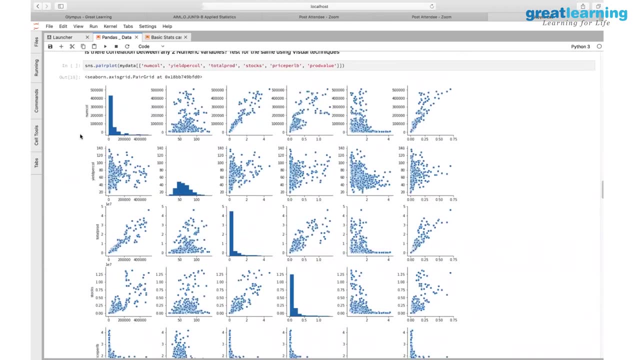 so anything that is closer to zero means there is not much of a correlation, either positive or negative. we'll talk about what is positive or negative later, but that value is that much, okay, hello chaitanya here. yes, take the third. that is third and fifth example on the top. 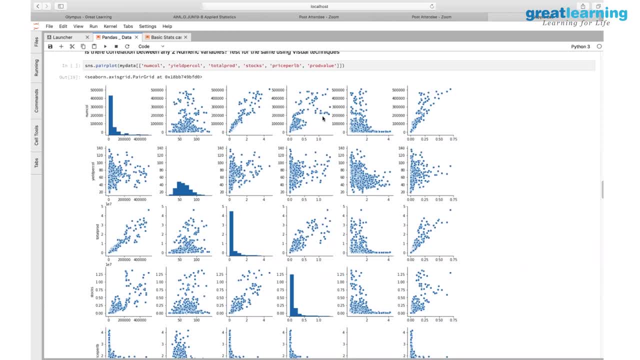 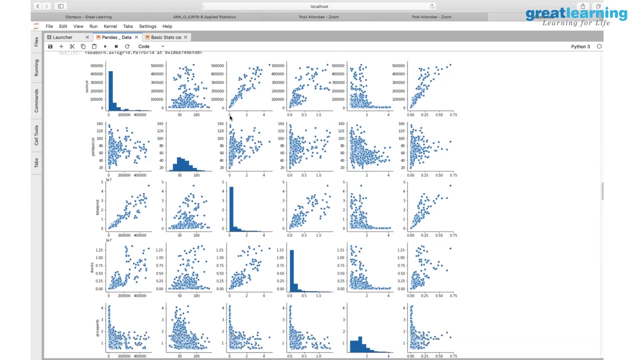 so here, if we convert into the equation, so it is like a y is equal to mx, maybe c is not there. it's a straight line equation. yes, this, this is y equal to mx. precisely because this is going through the origin, the c is not there. if let's say, let's say, for example: let me see if there. 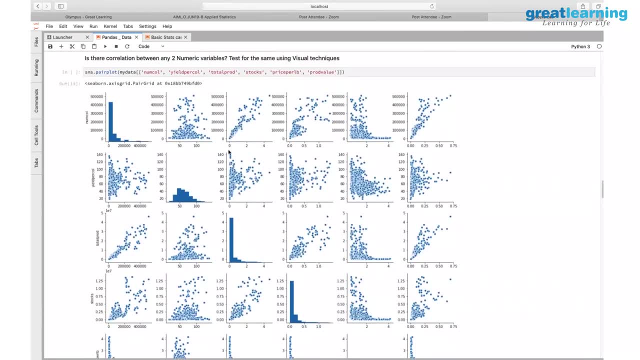 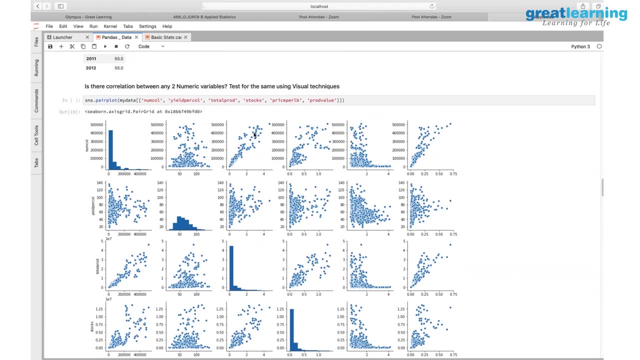 is another graph that talks about that. no, let's say, for example, let's say, for example, another graph has come like this from here at 20 000. the line goes: this whole points comes from here. what does that mean? there is a c component. irrespective of whatever do, there is a basic. 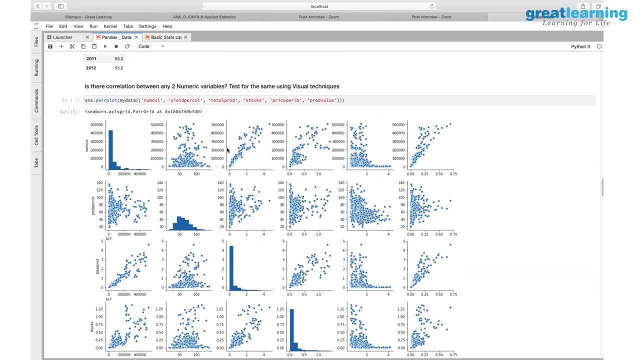 element of production. basic number of colonies that are there, which is 20 000. so that's why that is intersecting the axis at this point. it goes for like this: yeah, then the c component comes into play, otherwise this is going to this one: y equal to mx. yes, you are right. and then fifth is a. 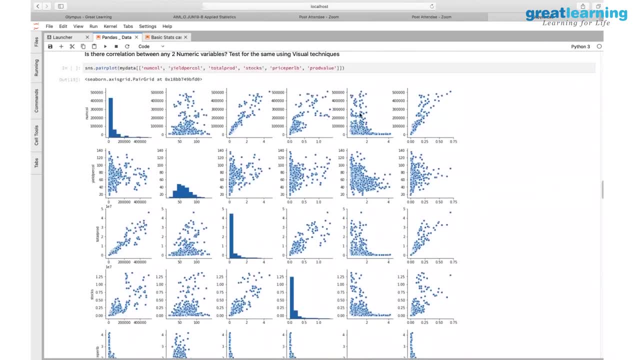 fifth, or this is fifth, same row, that is, y is equal to mx, so this is y equal to mx, so this is equal to c. right means there is a, even if it is changing, or yes, yes, so there is no. x component actually does not have any bearing on y. okay, this is how to find out. that actually means this graph. 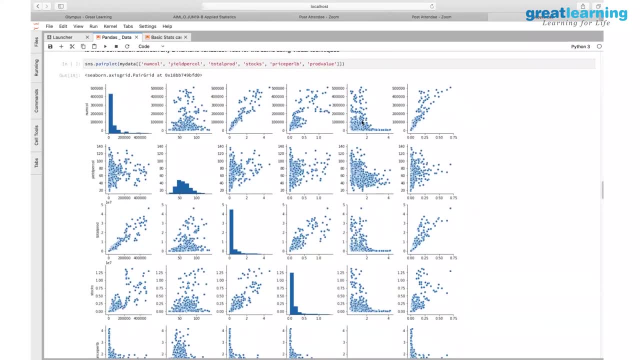 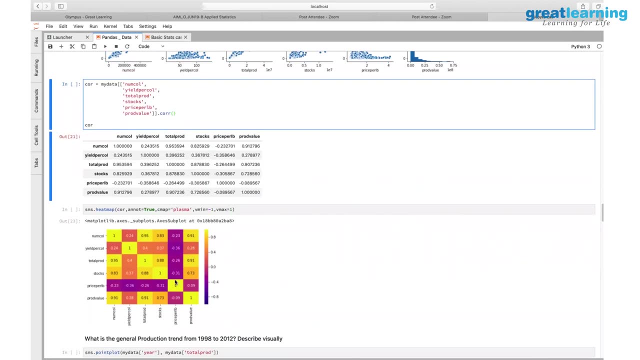 which is you are shown. there is that, uh, the colorful graph down the function is there, right? that is yeah, yeah, yes, that's a heat map, right, yeah, this is a heat map. how to get this heat map? that, yeah, how to find out the like, the equation from this or? 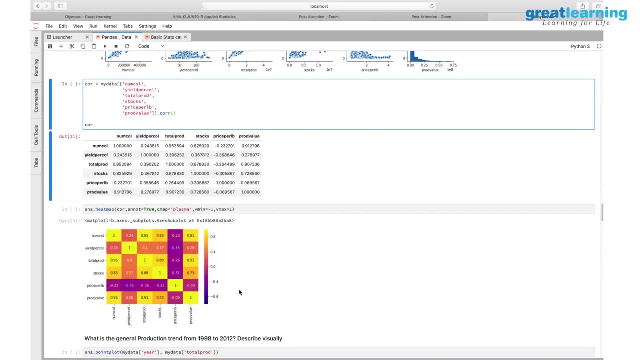 i think we are jumping way ahead about the equation part. we'll come to that probably in the next one or two sessions. we'll think about creating equations: what is the dependent? then? we need to understand a lot more things. what is a dependent variable? what is an independent variable? 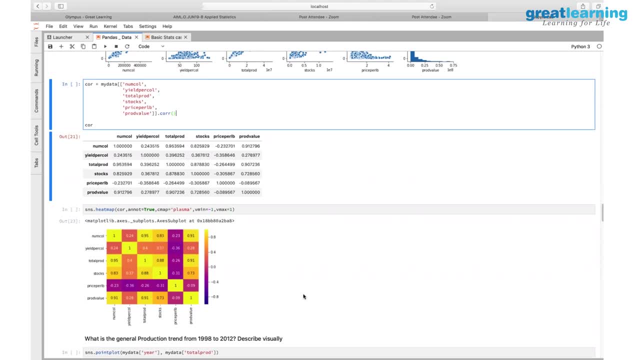 what impacts these variables, what exactly we need to look before we form an equation. we'll come to that, definitely, i think, because you asked that question about y equal to mx and going through the origin. i explained that, but uh, just hold on for one more class, maybe we'll come. 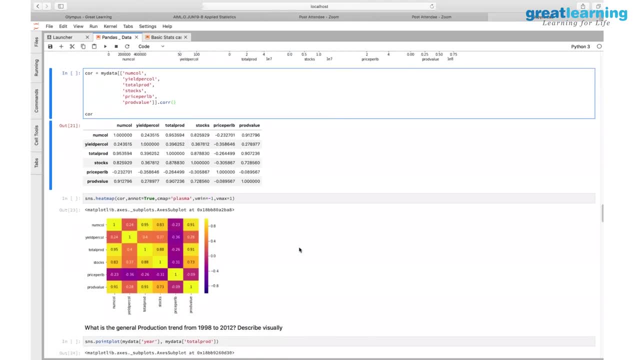 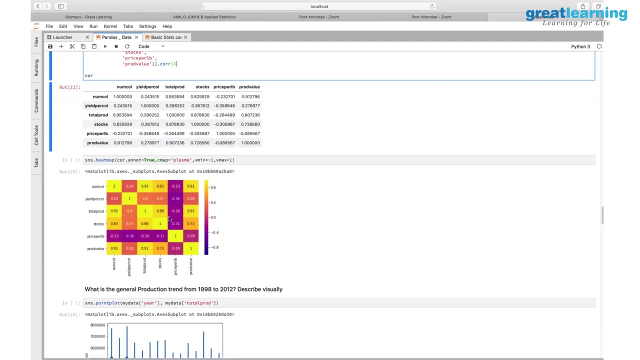 back to that. so so that's the concept of the variables and coming with equations, okay, right. so here we'll come back to this correlation and in correlation, essentially we are looking at the values that are coming here. the same represents, so, as you get a higher value, 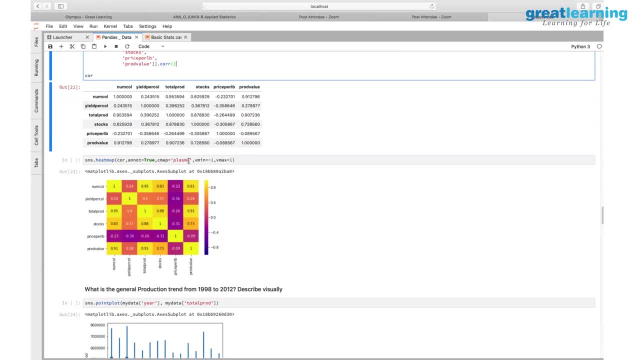 the color code. color coding can be anything. there are different color patterns here. the c map is nothing but the color map. they are using a plasma. then there are different color maps. you can just explore different CMAPs that are possible that you can use Matplotlib. color plot object. you can search on Google. 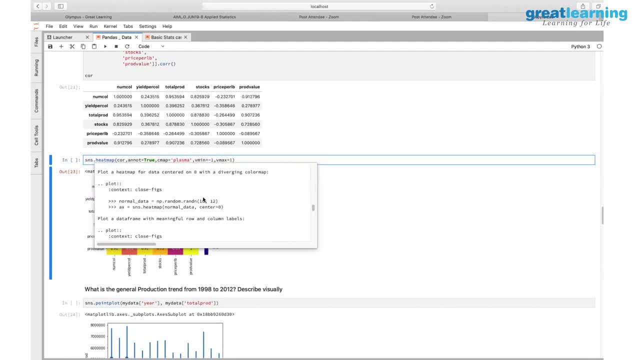 you find the different CMAP values available. You can apply any of them to get that value, But there are multiple color map codes that are available. The color patterns change. essentially You'll see different color patterns. Plasma is one example of that one. 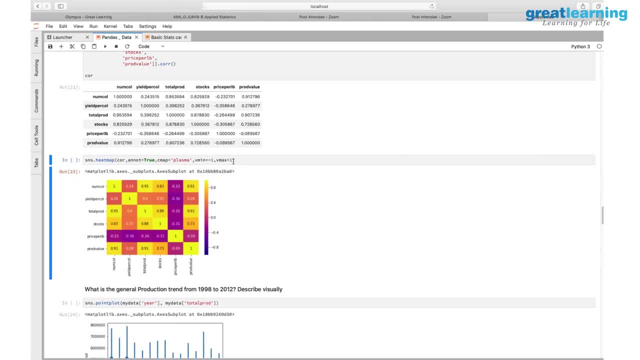 So minimum value is minus one, maximum value is plus one Because, for correlation, the value ranges between minus one to plus one, And that's why we have defined vmin and vmax values for this grid essentially. So this is the map, essentially. 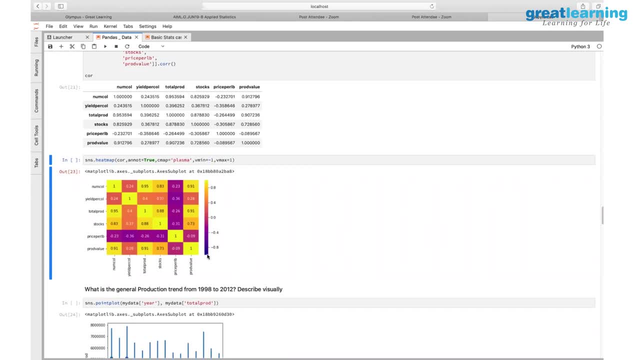 So you see, it starts from minus one, goes to plus one. Minus one is completely dark, plus one is completely yellow. So that's how the color coding gets decided. So the CMAP and these values decide this line and color coding. essentially, 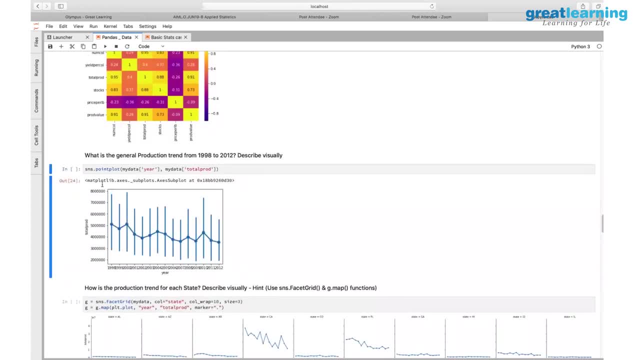 Is this part clear? Yep, Yes, Ram, All right, So the next one is point plotter: Ramon. one question. So this, This heat map is used, not specific to correlation. is it So when you said minus one to plus one, so it can be? 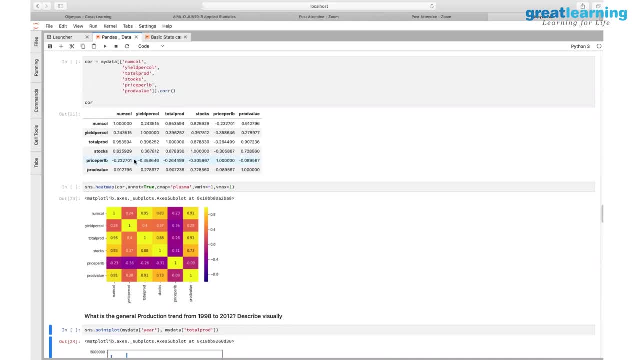 Yeah, not specific to. It can be used other ways also. It can be used other ways also, But predominantly this is used here because a correlation map makes it easy to understand visually what are the things that are really correlated with each other versus not. 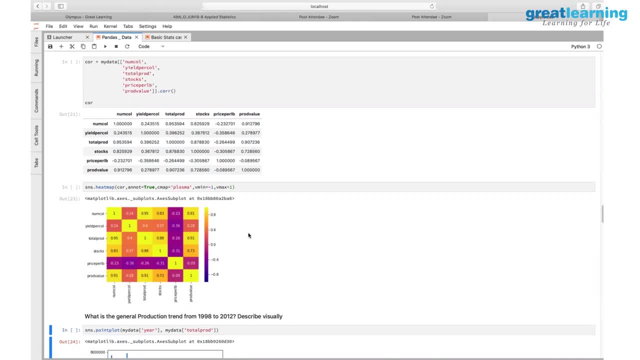 That's why we use. But heat map can be used in different contexts. Let's say, for example, you take 100 states that are there and on different parameters you want to see just in Excel. you see right, For example. let me go to Excel simply. 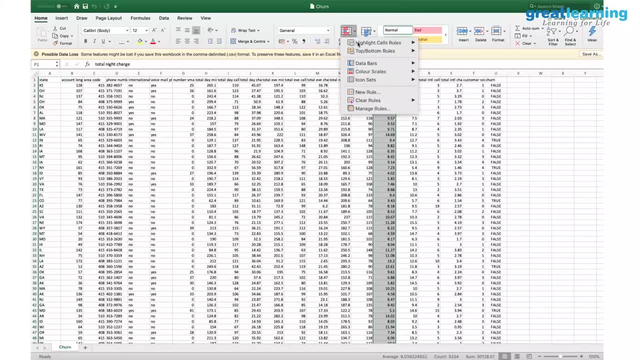 Let's say, for example, this value, I select this value, I do a conditional formatting and maybe this is also color coding in a way, So you can do this kind of color coding also using that heat map variable. essentially Okay. 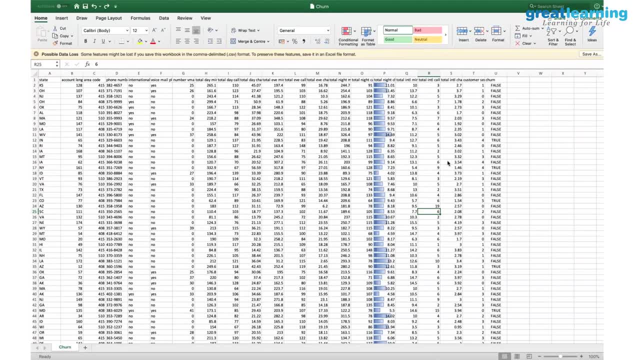 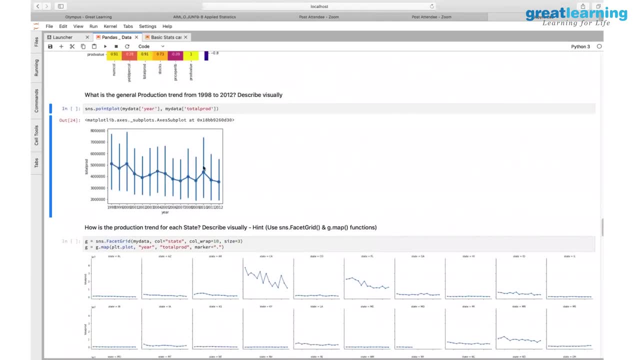 Got it. Thanks Got it. So it can be used for any purpose. Correlation is the example of the instance I'm using here, but you can use in different contexts. Okay, So moving on to point plot. Point plot essentially is about for each of the variables that are here that you list in this point plot. 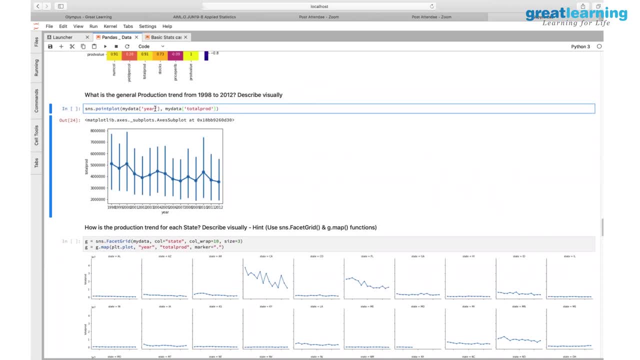 Here, for example, we are taking the total production and we want total production by year. That's what we are trying to do, So this draws a line. essentially, This is for each of the years. What is the total production happened? 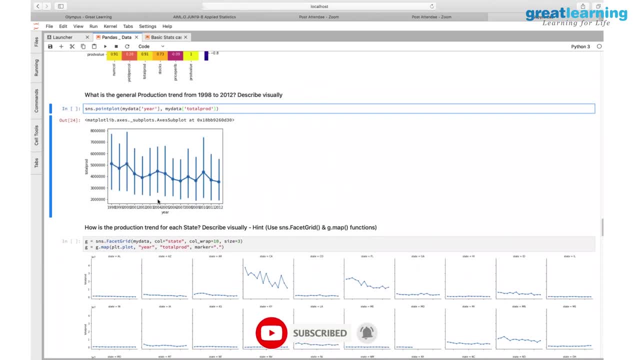 You see. So if you see this graph for one second, ignore the vertical lines that are out. What does that tell you? We'll come to that. So if you take this vertical plot, so what is the interpretation we are getting in? 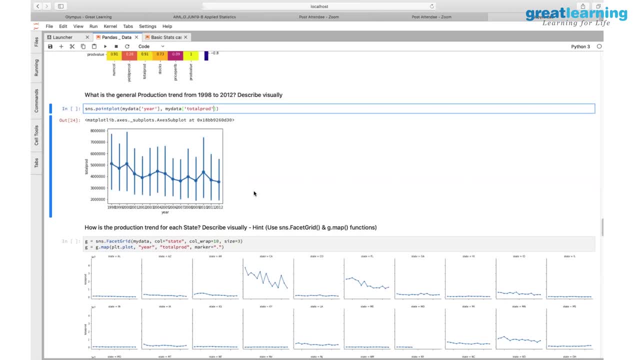 The total production over a period of time is going down. That's what the hypothesis that we have seen, And that's the same interpretation we are coming here. But now, why these lines? What does this tell you? So, each of these lines, the point plot, sorry, 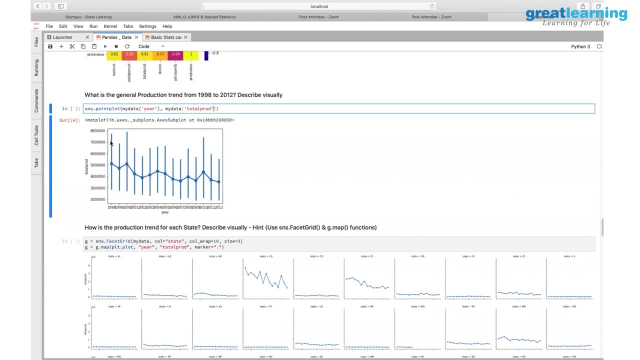 It's a range, right? Yes, it is a range. So what is the range that is coming here? What is the minimum value that is out there? And maximum value. So this tells the whole value, But the total range that is out there is given by this particular one in that particular year. 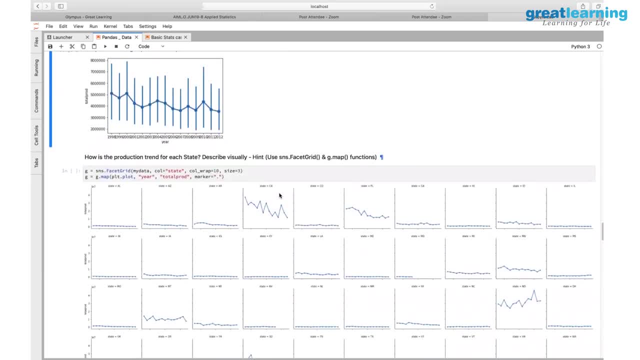 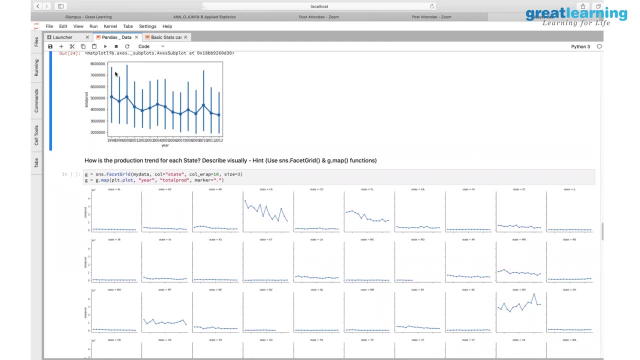 That's the variation you get Clear. That's what the point. plot uses an additional value. So, even though value is decreasing, 2010 seems to be an exception. The production has been phenomenally high in that particular one, which is reflected by a small bump there. 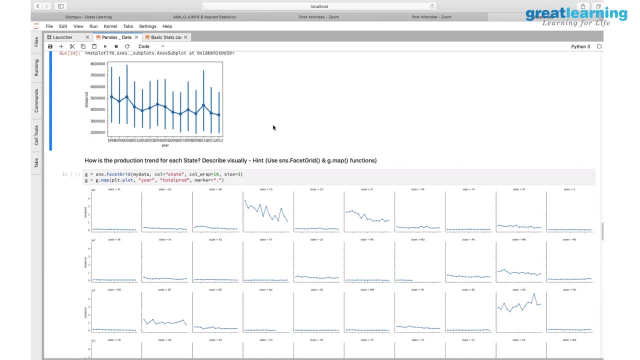 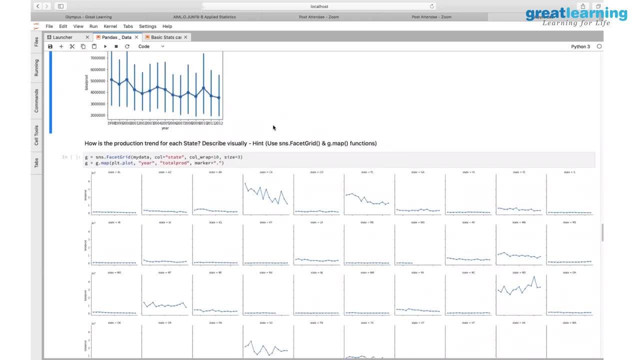 So this gives you a much deeper view than just a point plot and a trending line showing the drop And the production over a period of time. That's one way to know the things. Now the last question: How is the production trending for each state? 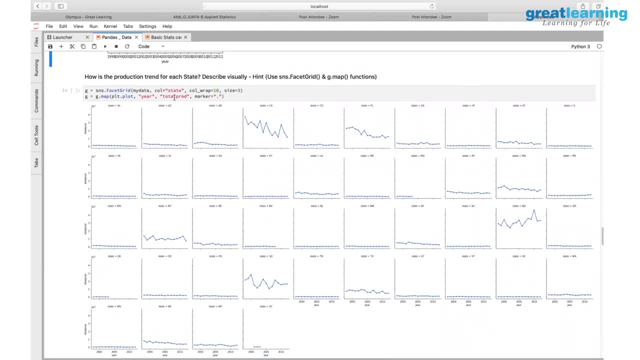 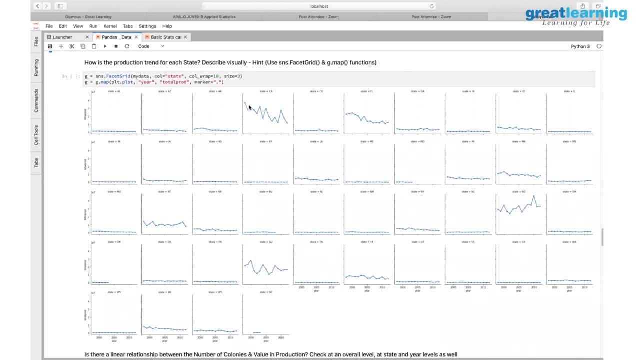 We'll just take the production variable again. So here I talked about facet grid. right Facet grid helps you create this grid structure. All I can define how many graphs I need to create in one row, which is column wrap. These are the columns. 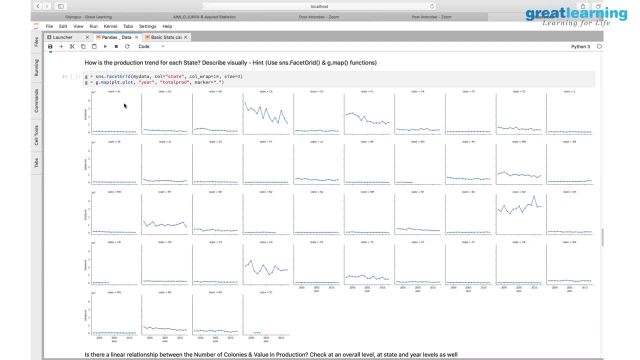 So the column wrap I defined at 10.. And size is three by 10.. And size is three by 10.. And size is three by 10.. This is the size is a three by three grid, Each map size. That's how it defines. 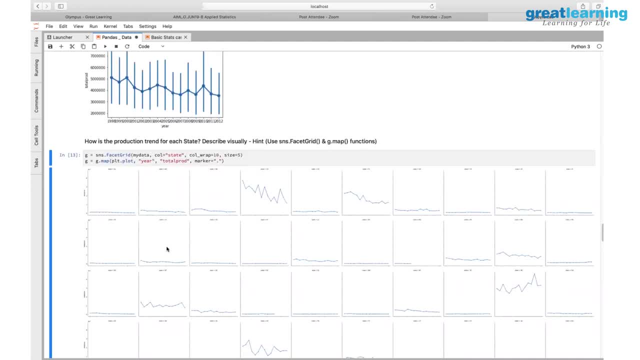 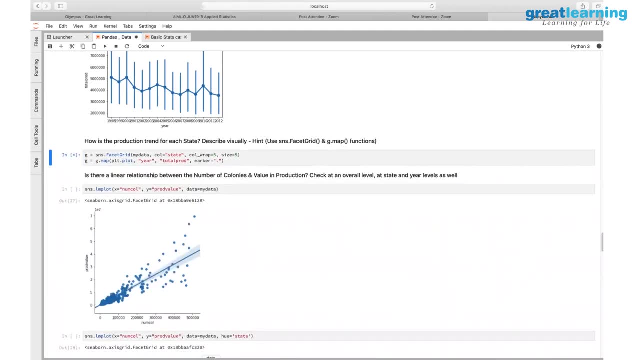 If I change that now, the grid size changes. It has become even smaller. It is getting different values. If I say only five columns per column, it creates a different way: One, two, three, four, five, It creates five columns only. 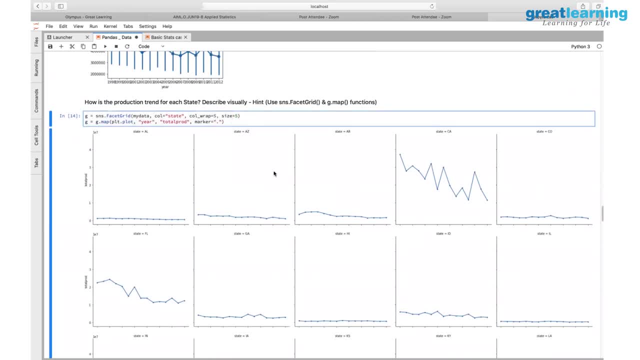 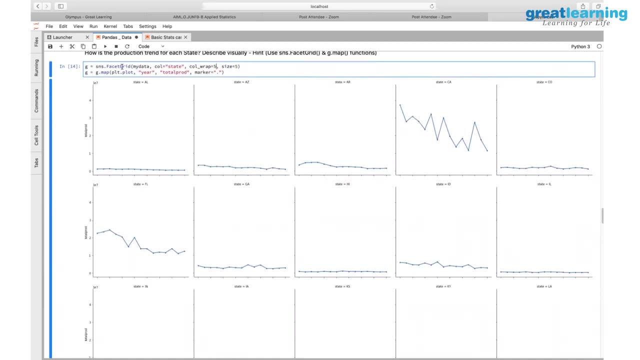 So you can just play around and see which works, given the number of data. you're looking at which column you're looking at, how much you want to do. You can start exploring, But what this does, It plots. this is basically a context setting. 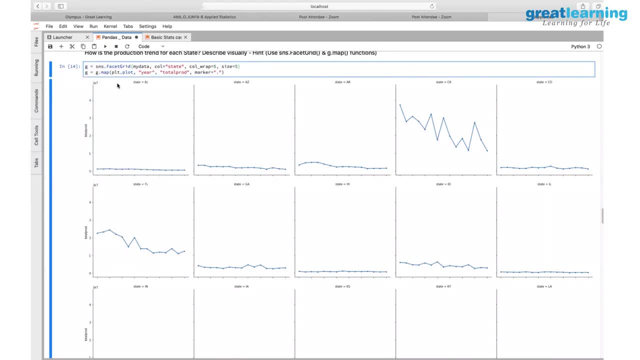 This face it does not do any kind of mapping. How your map should look like is defined by face it grid. You understand that part right? So here I want five columns, and size of each graph is five. That's what I'm defining. 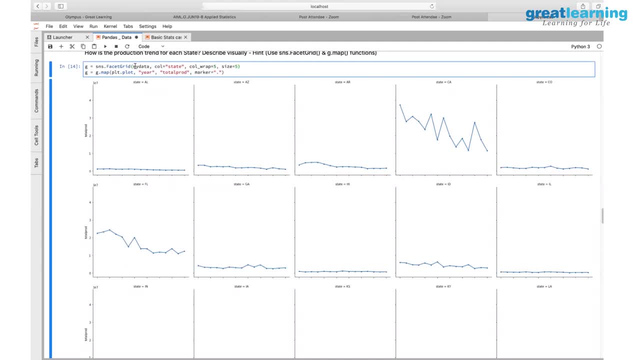 And the basic, and it should be based on my data set. I defined that. Now that is assigned to this variable called G. Now, through the G, I am mapping a plot between year and total production. So the year is on this X axis. 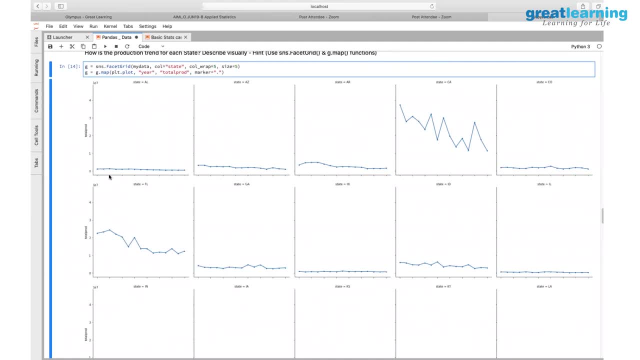 Total production is on my Y axis, So I know per year how it is a thing that is coming up And the marker is dot, which is nothing but these dots that you are seeing here. The marker is this particular one. The PLT dot plot is showing. 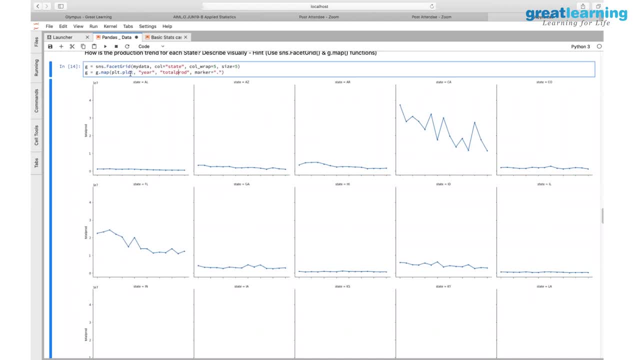 So the PLT dot plot that we are using is the plot created here. We are plotting that here, passing that to G, which will put that into this face it grid that we created. The data gets mapped into this particular one. So now it is. 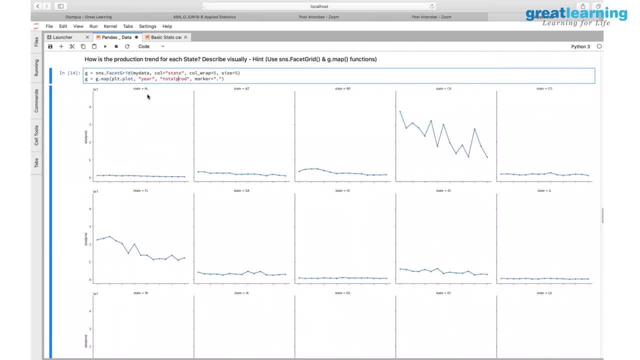 It's about interpreting this data. See some of these variables in. for the state L There is no change. It has been the same, Maybe marginal drop. It is looking the same here. It is slightly up here down, But this state, California, seems to be an interesting one. 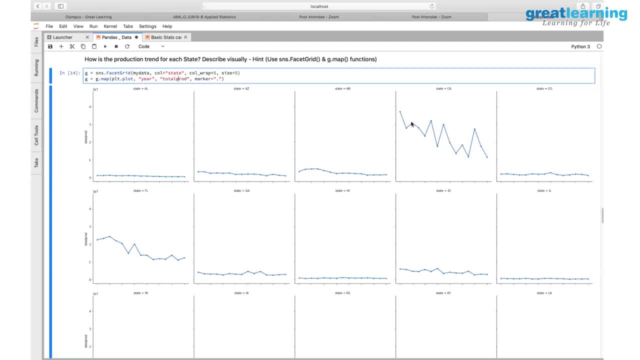 It is overall. If you look at the trend line, it is dropping. It has dropped marginally, gone up, then continuously down for two years, then gone up, Then there is a significant drop, significant up, then continuously dropped. But overall, if you look at the trend line, it is dropping. 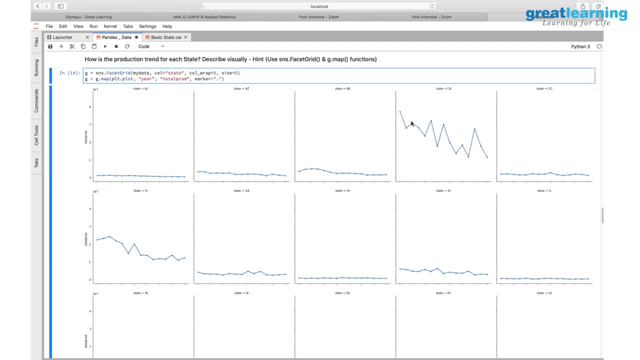 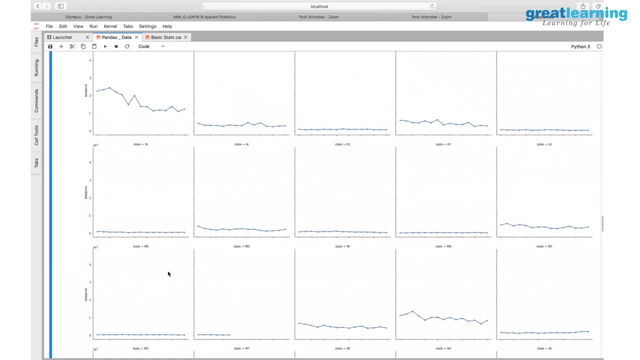 So so you now you know, based on this information that this graph, That California is acting very differently, Then, similarly, Florida is acting very differently, but most of the states are more or less showing the same trends. These are the quick observations. 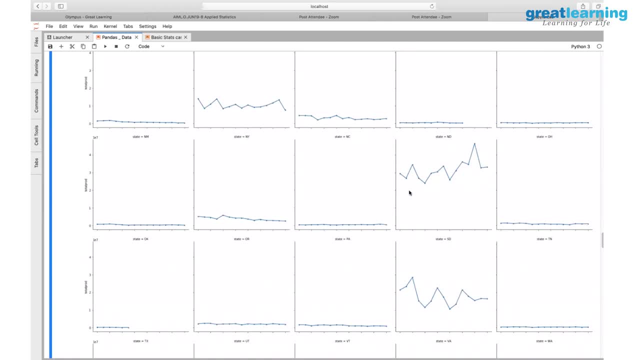 And this state is interesting, San Diego- you are seeing an upward trend. Actually, even though ups and downs are happening, you can see a marginally upward trend line on this particular, which is an interesting state to look at, So once you identify this. somebody asked about creating multiple hypothesis. 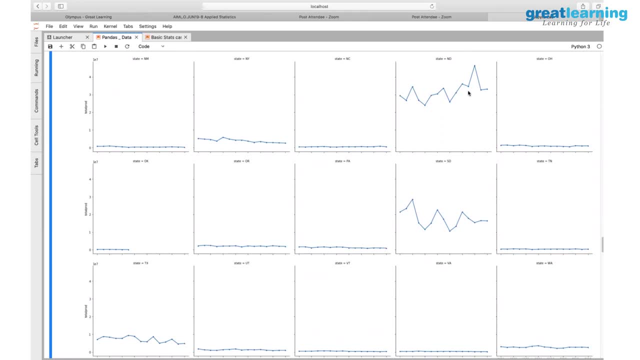 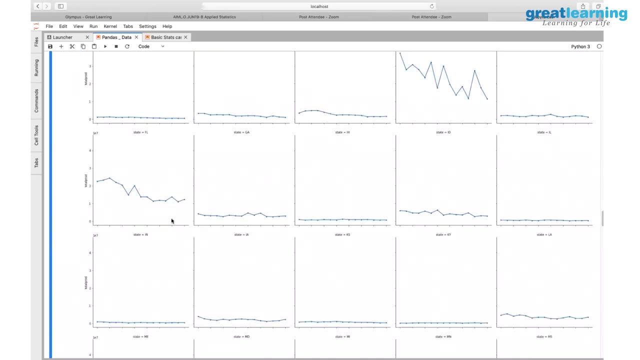 Maybe I create a separate hypothesis As to why not Dakota is acting differently or why a San Diego, San Diego, California or Florida or these are acting differently compared to those. you create separate hypothesis for them and then you can do deep dive analysis accordingly. 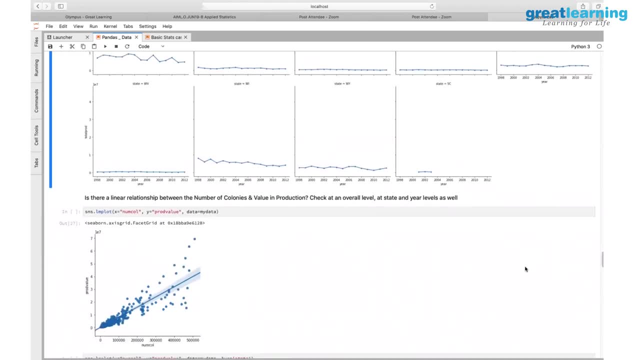 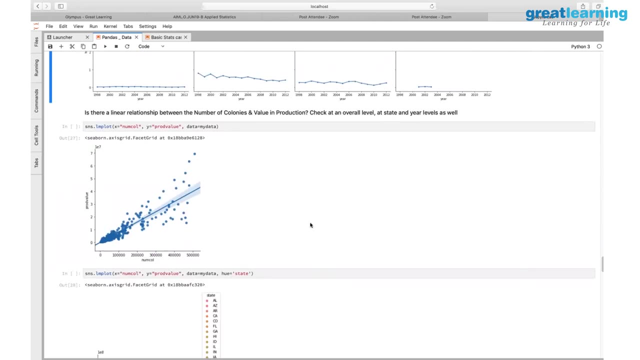 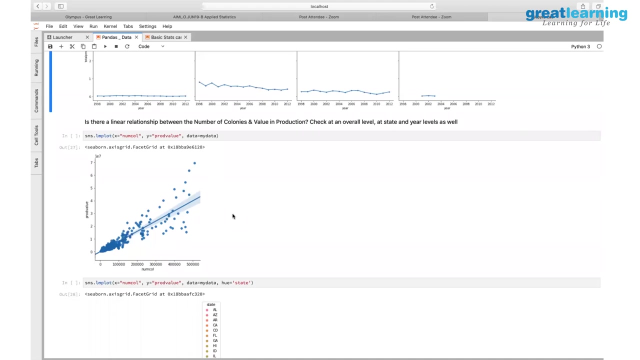 That's how you can use these graphs for your purpose. Does it make sense? Yes, ma'am, Yeah, yeah, Good, So now we are getting into something called as a LM plot. LM Plot is predominantly a scatter plot. The advantage that it gives you is a trend line that I talked about. 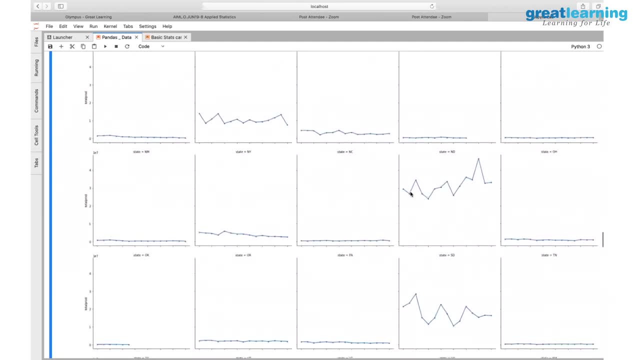 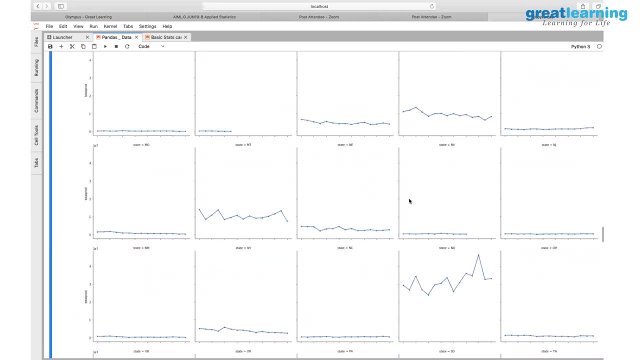 If I create a trend line for this one, this chart for North Dakota, it is slightly going upwards. If I create the same trend line for California, it is a declining trend. So the same graph you can create here using the num call and production value, two different variables taken. 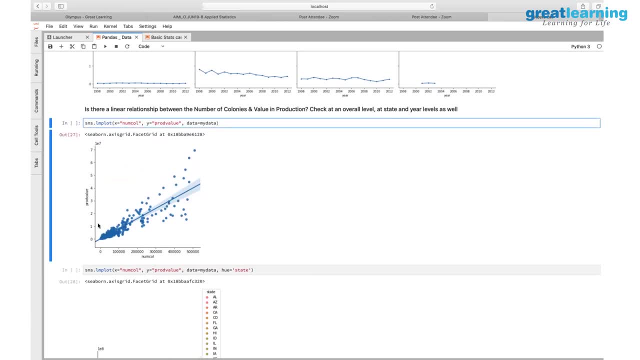 But for num call, if you draw a scatter plot for this one, it creates Just to use a scatter plot. it creates a scatter plot for this. But what does this LM plot does? It creates a trend line for this. You know how much is the? where is the trend happening? 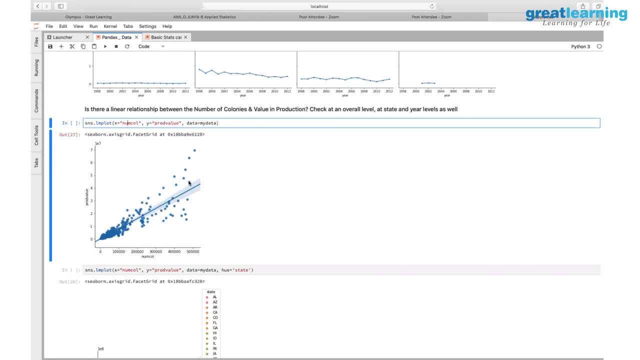 So now can you, can you see this small blue shade happening around that line? Yeah, exactly, Yeah, right. So what, what? what is the shade indicating for me? Any any guesses? It's the range of the trend line. 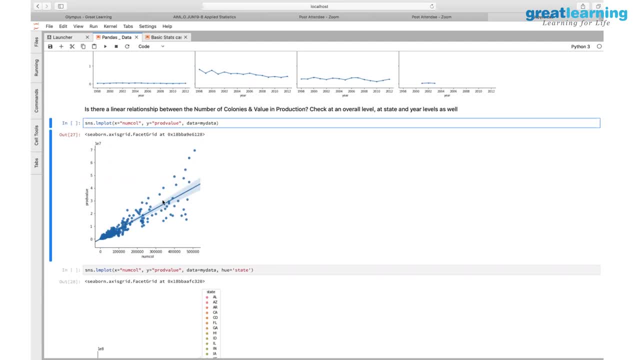 Range of the trend line. But more importantly- but you don't see that same- The shade dispersion at the beginning of the thing you are seeing. it is increasing only when you're going on the other end, Because the data is linear mostly here and more concentrated in this part. 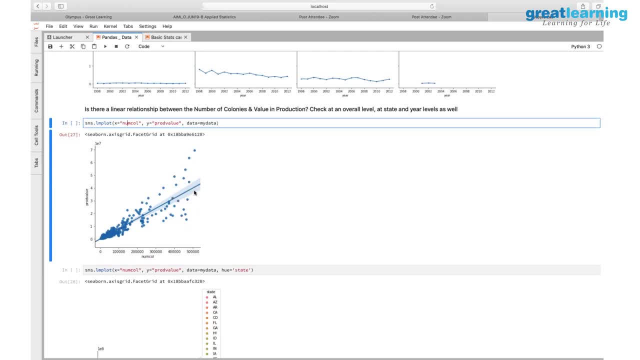 As you go to the thing, the data is getting distributed, The shade distribution is also happening accordingly, And the correlation is going down as the as the graph is moving up right? Yes, Yes, Because it's not like a completely diagonal 45 degrees. 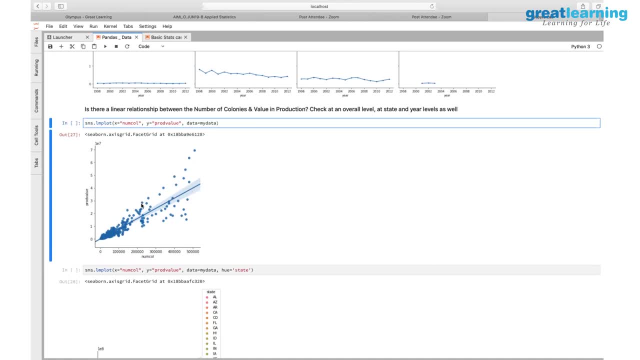 It is more at 35 degrees or 40 degrees, somewhere around that one. It's not a 45 degree, And the dispersion Is happening more in the data as it is going on the higher values. The same thing is reflected by this shared at that here. 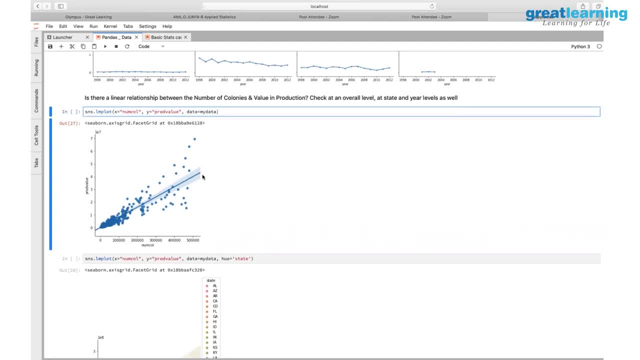 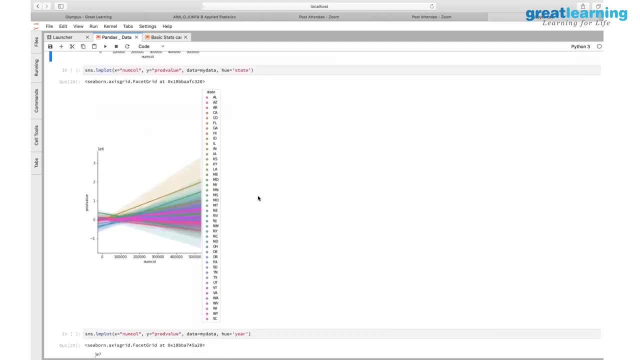 That's what LM plot can tell you when you look at the data. the syntax is. once you share this file, you can use the syntax and start exploring for different variables and look at that Now in the interest of time. this is another version of the LM plot, but you're you're using, you're breaking it by hue. hue gives you a variable use. use a categorical variable where you can get the distribution for all the categories in that particular variable. 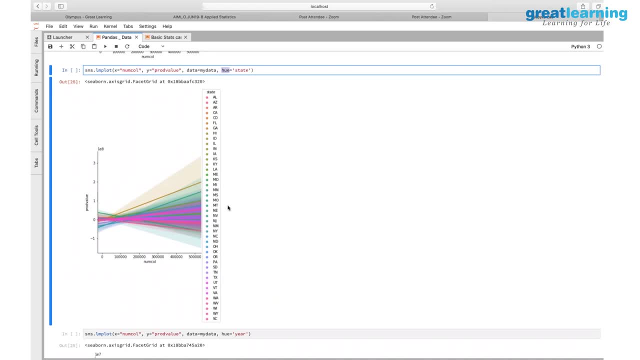 If I take state state, has some 15, 20 states listed or 30, 40 states, whatever it is. but each of the things, the distribution is shown, while the map is confusing. It's a demonstration and you can get a sense of how the overall distribution is coming up for all the states together. the trend lines. 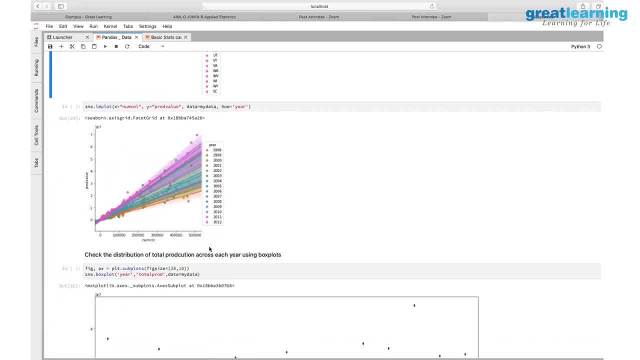 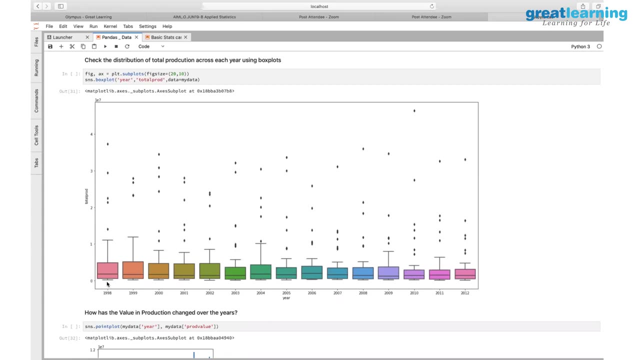 That's what it shows. So again, LM plot by year, same thing. Now this is a box plot. So what does the box not say? as we have seen earlier, a minimum value. here at the bottom- This box, lower part of the box- this talks about first quartile. the line inside the box talks about medium. 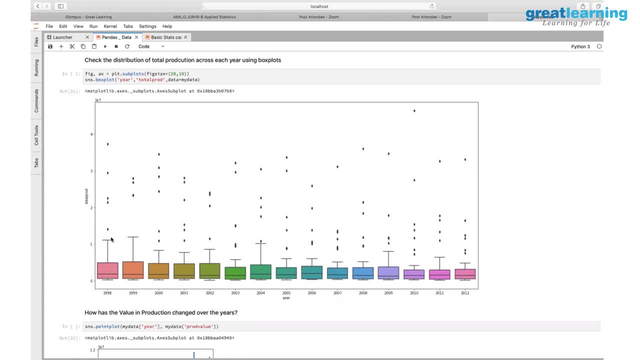 This line talks about third quartile and this talks about the maximum value. That's what the box plot tells us. That's what we interpreted right. But now you see a lot of dots here. I know I've been in them. talked about this dots in the video. 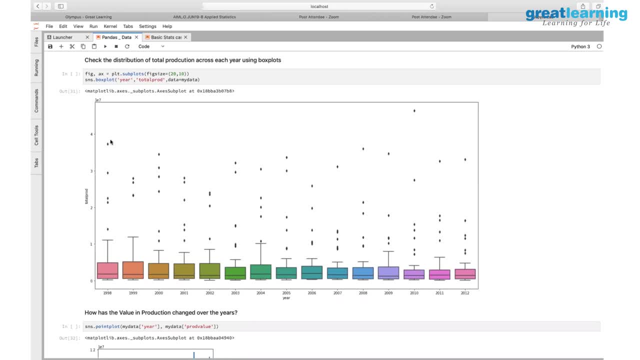 Does anyone remember what this darts in ticket outliers? Yes, They are the outliers. But my question is: if you have a maximum value here, how come there is a value which is an outlier above the maximum value? The maximum value is calculated based on that 1.5 into IQ, IQ. 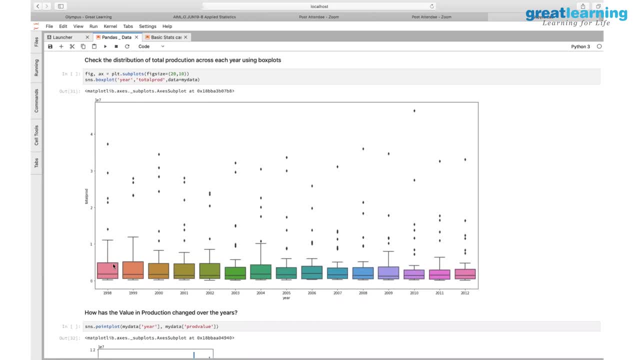 Yes, right that that is calculated using 1.5 into IQ. for those people who are not in sync with that IQ or concept I come and then we talk about it. So basically, when this box plot is created, it takes all the value into cognizance, then it defines the accept. 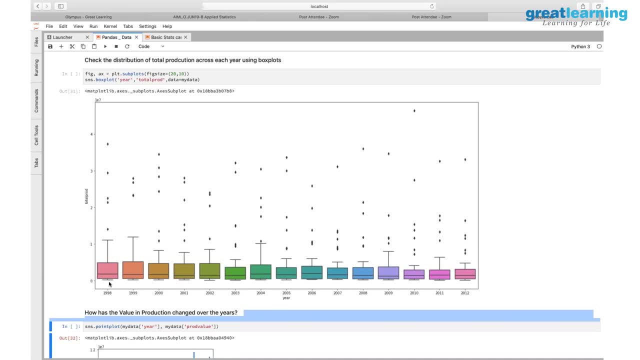 To pull range of minus 1.5 to plus 1.5 of the IQ or value. IQ or is nothing but Q3 minus Q1. This is third quartile minus first quartile is called as IQ or and you take the IQ or value and multiply that by 1.5 on the minus side and on the plus side of these things. 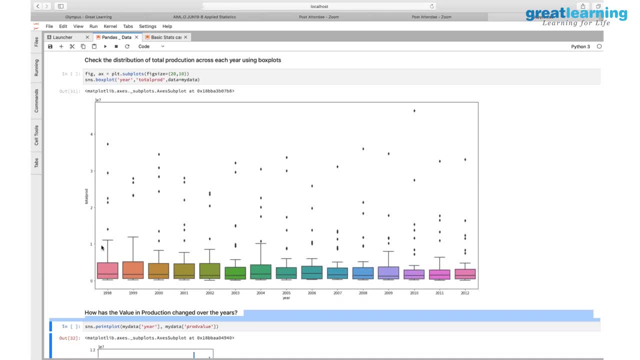 Then you get your minimum maximum values decided and then whatever the values lying above that higher value of 1.5 IQ or that you are getting in, those will be identified as outliers. That's why you see all These outliers across, and this happens more. 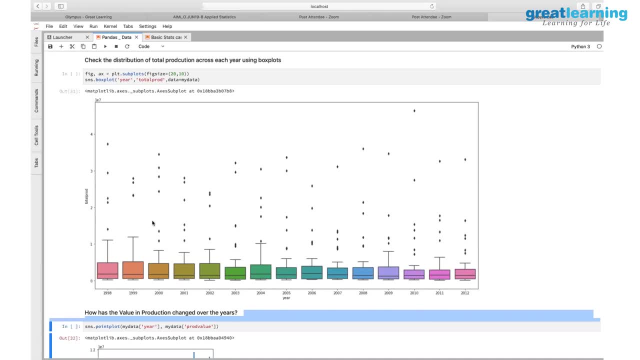 So when you plot all of these things together, let's see how this box plot is getting created. So we are creating a figure and access. access is primarily for this grid that is creating. So the size of this plot size, basically 20 by 10..